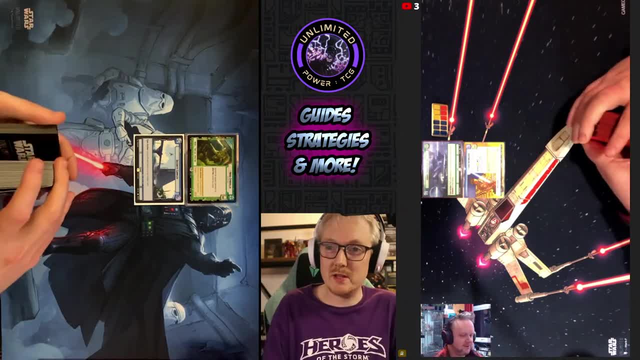 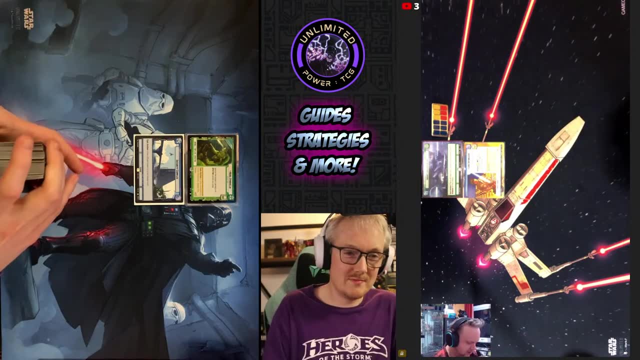 made like two improvements, or hopeful improvements, to this deck since I beat Tony. Okay, So I've added: Do you care, Do you want to know? No, no, no, I don't. Do you want it to be a surprise? or you have no idea what's in my deck? I have no idea what's in your. 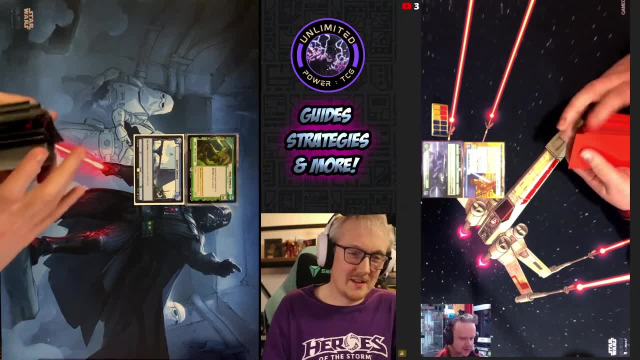 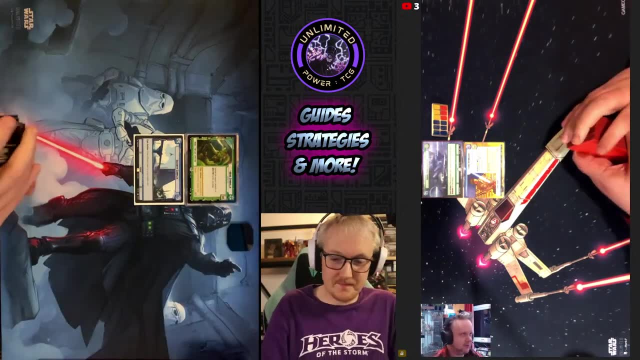 deck. All right, then let's do it that way. That sounds fine. Yeah, All right. Are you shuffling, Are you? I am shuffling, I'm good to go whenever you are, Since you can't cut my deck, then that's going to not be a thing, really Cool. And people are tuning. 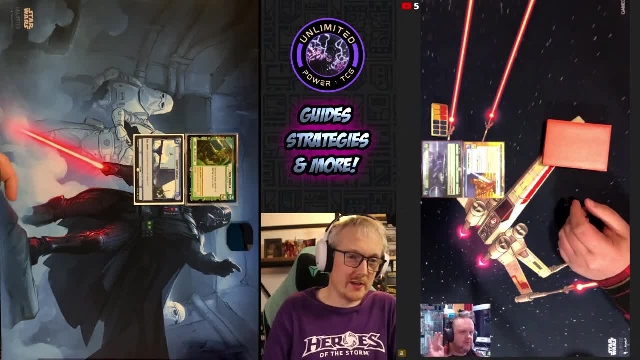 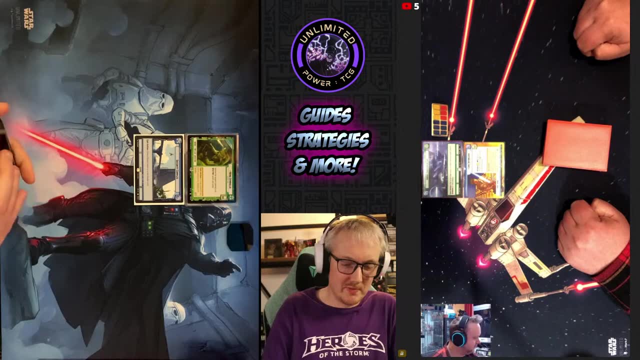 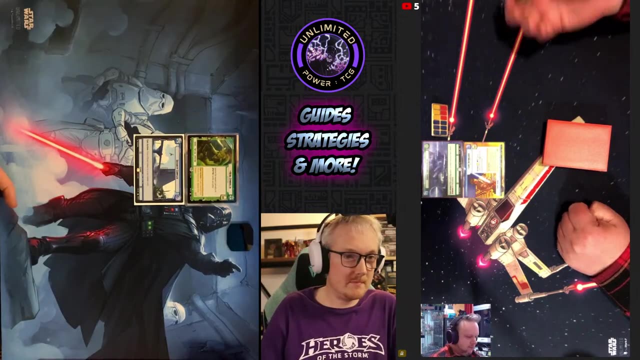 in. We've got five people watching live. Good evening everybody. Feel free to ask any questions. Yep, Anything else you might want to say that Star Wars-related. by all means, may the Force be with you. Thanks for tuning in. Absolutely Cool. I feel like I'm shuffled. That's cool. 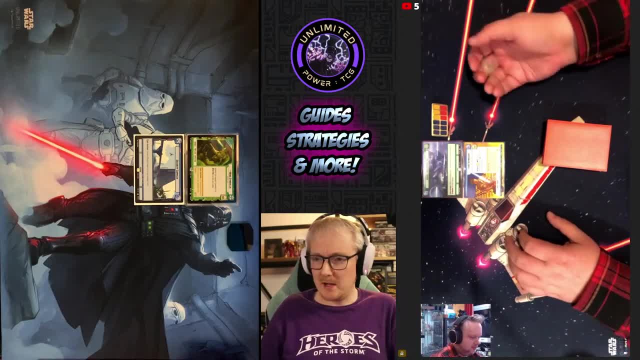 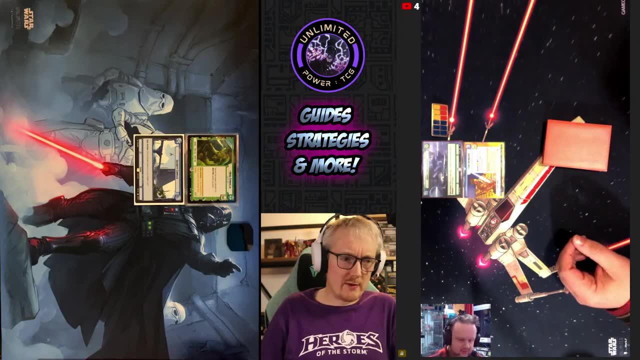 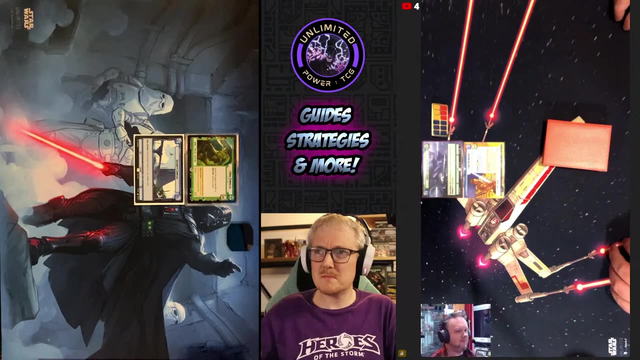 Right, So call oddscom Odds or evens for initiative. I'll go odds. That is an odd. Would you like the initiative? There's no downside. if you like having it in turn one, I think so I'll take the initiative. There's a very rare downside but it depends. 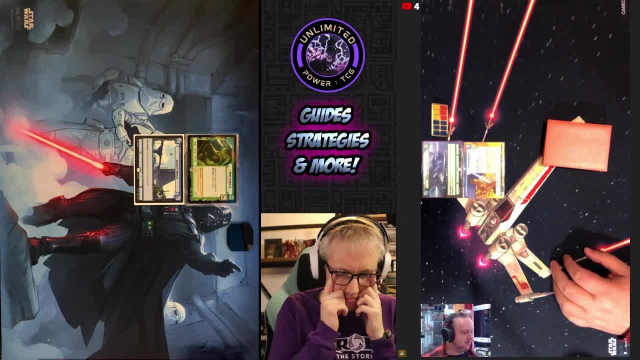 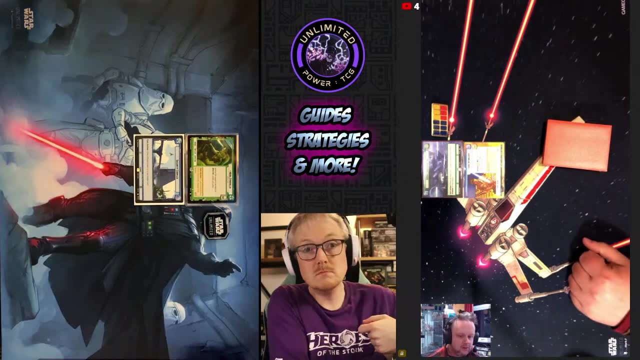 if you want to see what the opponent does first before you react to it. But generally speaking, it's considered good to take the initiative because then you can take the initiative for the second turn and act before they do. Good point, So I'll take initiative. 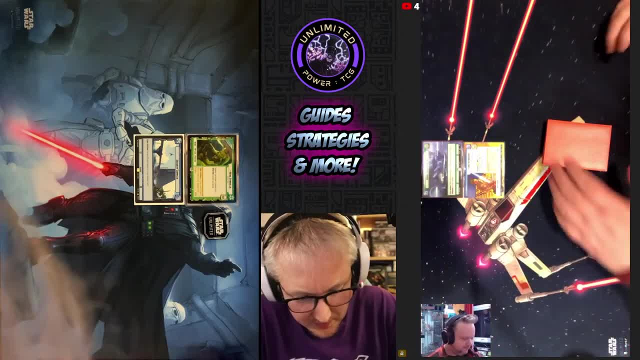 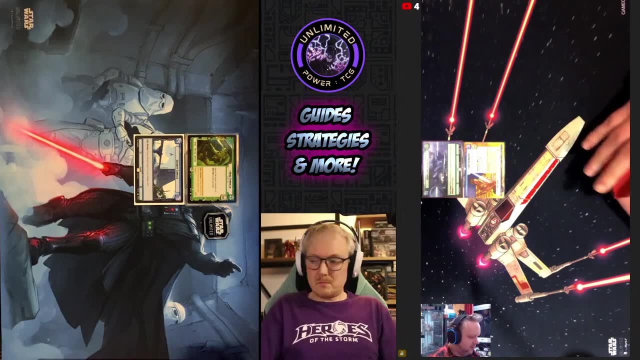 I am running Hera and the Security Complex. So the Security Complex epic action is: I get to give a shield to a non-leader unit once per game. Yep, And the Energy Conversion Lab, epic action is the infamous one. Play a unit that costs. 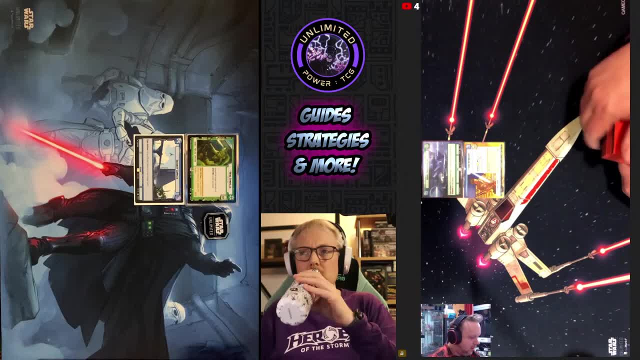 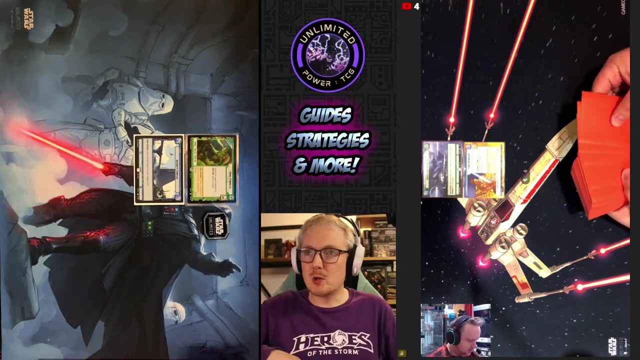 six or less from your hand. You have to pay the normal cost. as always. Give it Ambush for this phase, which is fairly tasty. Ambush is very nice. Okay, Cool Luke's action is you get to exhaust him and spend a resource. 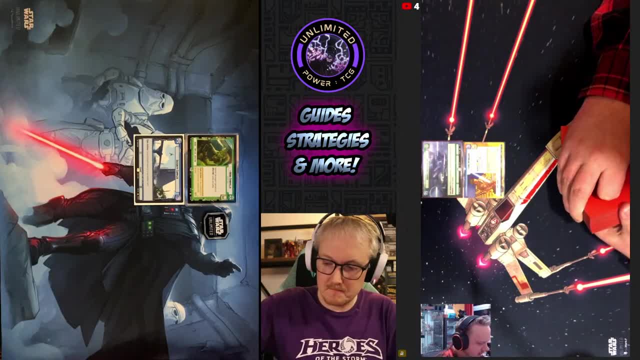 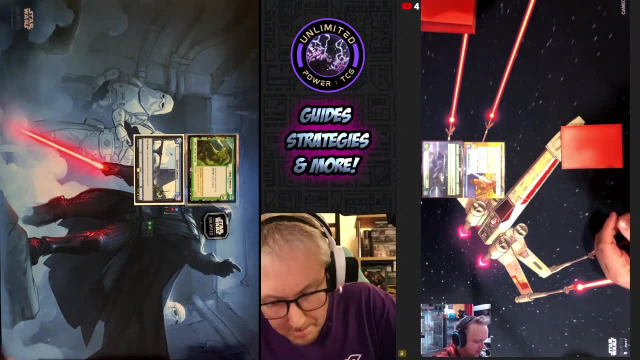 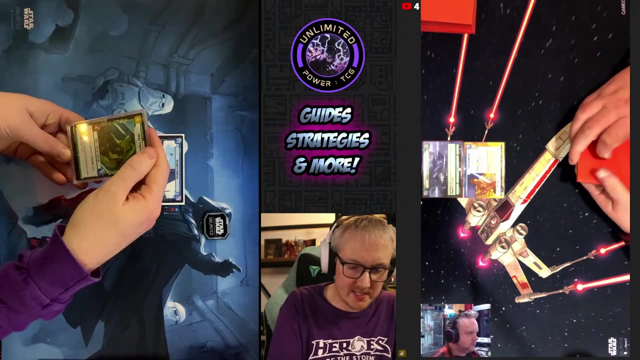 You give a shield token to a hero unit that you played this phase- Yep, Very good. And he deploys on turn six. Sorry, he deploys on six resources, So that's his epic action at that point. Cool. So Hera deploys on six as well, And her thing is that I can play any Spectre cards. 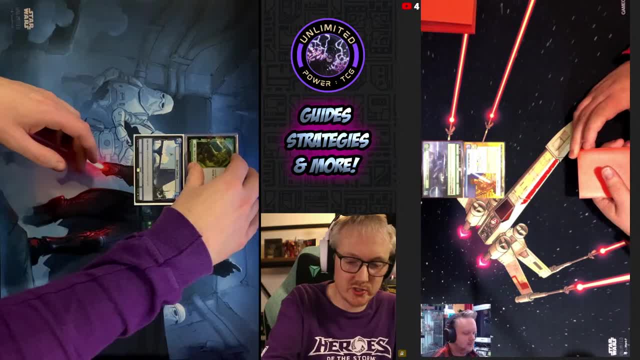 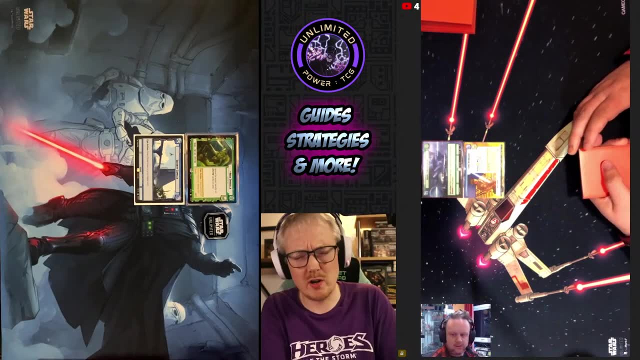 without the aspect penalty. So if you see me play any red cards, such as Sabine or Zeb, and not paying any aspect ratio, that's literally why- And I think Zeb is a very good card, actually because he does like four- 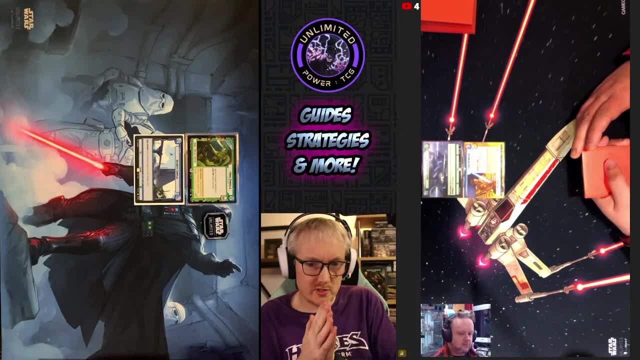 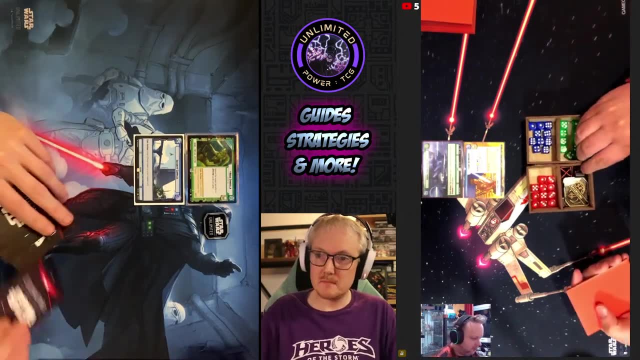 He does like four damage after he kills. We've got two people here in chat, the Crusher and Steven. Hello guys, How are you doing? You ready to draw? Yeah, I'm ready. I've drawn my six, Just as a record. I don't have a set of tokens bought. 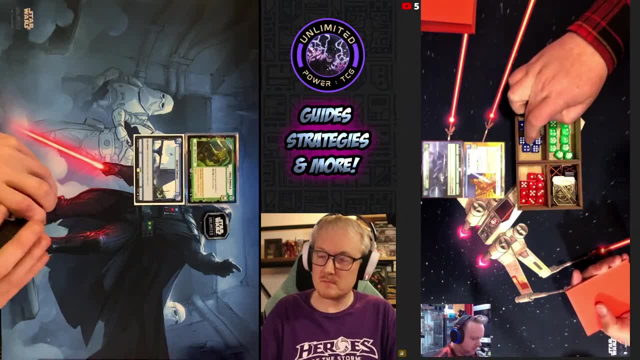 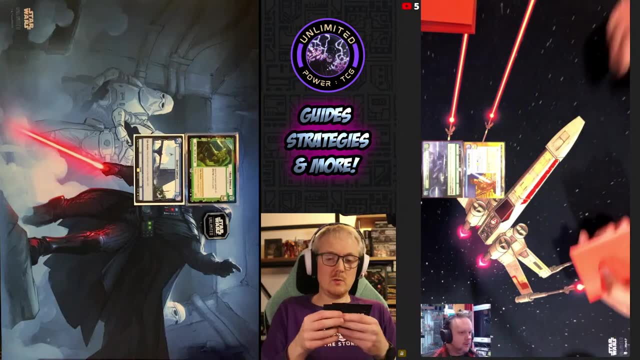 so I'm going to be using red D6 for damage, blue D6 for shields and green D6 for experience tokens, if they'd be needed. Okay, Okay, Sounds good, Right? Wow, a mulligan in this hand I have. 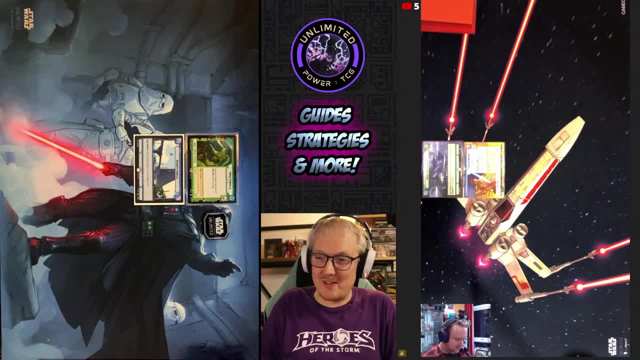 Not a good one for you. A lot of six or seven cost cards there- Way too much. Oh, this is not the best starting hand, but it's also not the worst one, So I think I might have to suck it up and go ahead with this one. 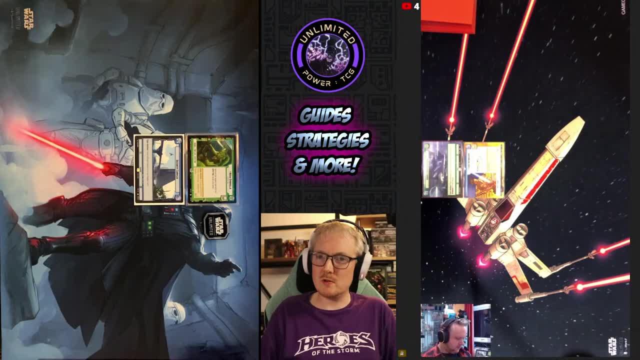 Okay, Are we playing best of three tonight? I put best of three in the YouTube thumbnail, so I assume we'll play best of three. It doesn't take horrifically long to play. There's no real reason why not. No, I don't think we'll be that slow. 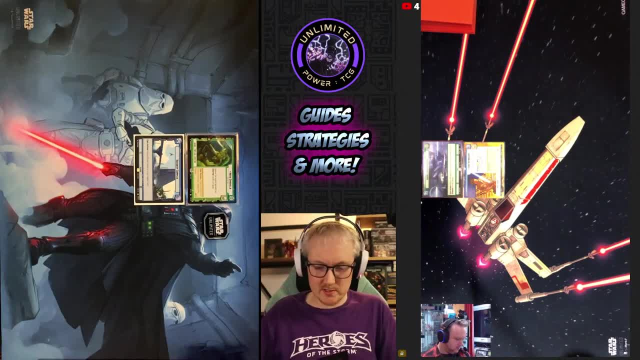 All right, I'm mixed again. I'm going for number two: Six cards. Let's hope for something a little bit better, Right? So we do that. Let's resource that. I don't think I want to keep that one too. 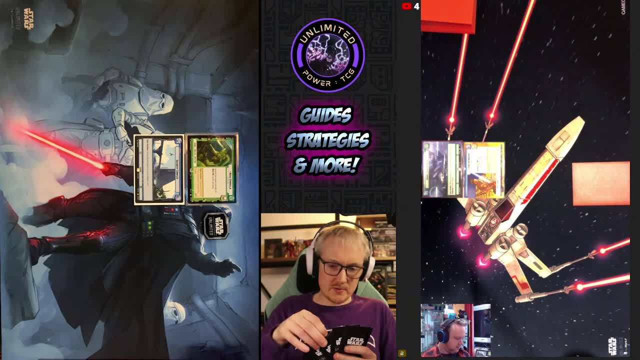 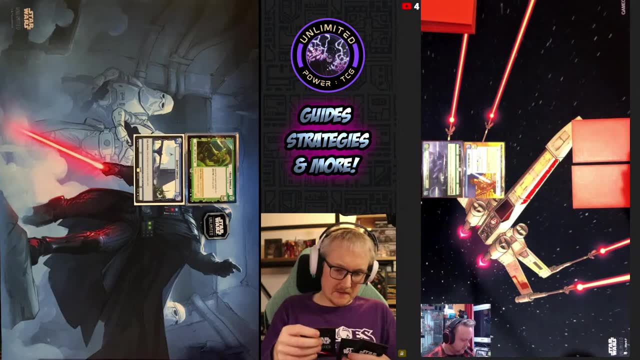 badly. All right. So turn one: we're resourcing two units and then we are up to two. I guess That might not be the best call to make, but we're going to make it anyway. So there we. 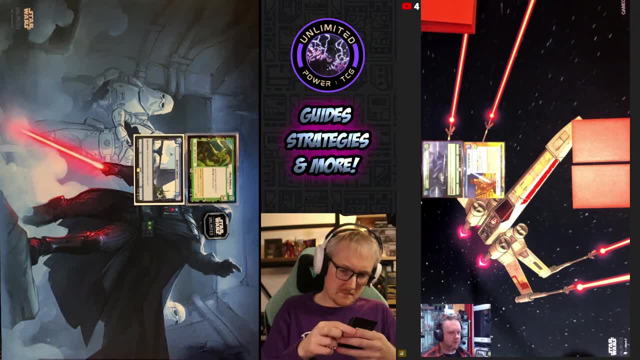 go. If you want to look away from the screen briefly, I'll. If you want to look away from the screen briefly, I'll. I'll show the screen my hand and it will be rotated for the people who are watching. Go for it. 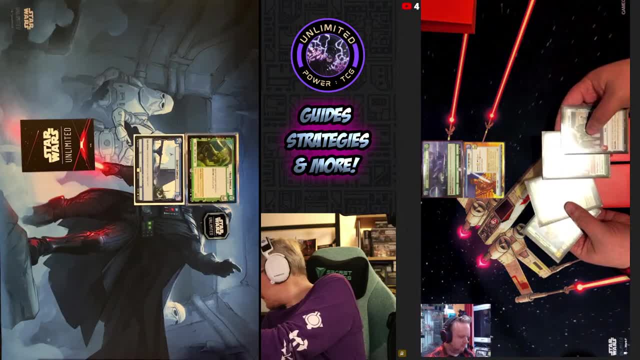 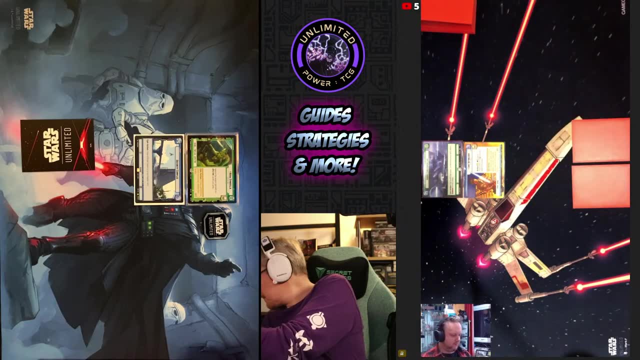 I suppose that's the thing. Right, There we go. This is what my starting hand is, having resource stuff which you might not be able to see due to reflection, so I'll tilt it a little bit. There we go, Cool And off again, And I'm looking away, if you want. 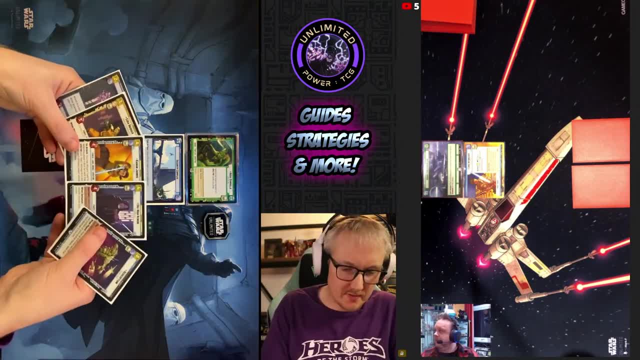 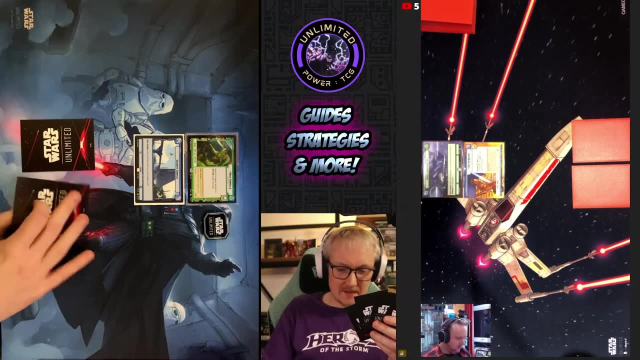 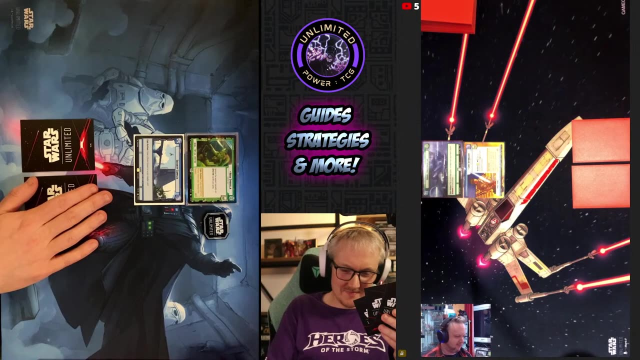 to do the same. My starting hand is rough, Okay, Is this after you've mulliganed? Yeah, Oh, okay. Well, you have the initiative, sir. Okay, I'm going to take the initiative. Oh yeah, That is rough. Okay, Fair enough, I'll attack two and play a battlefield. 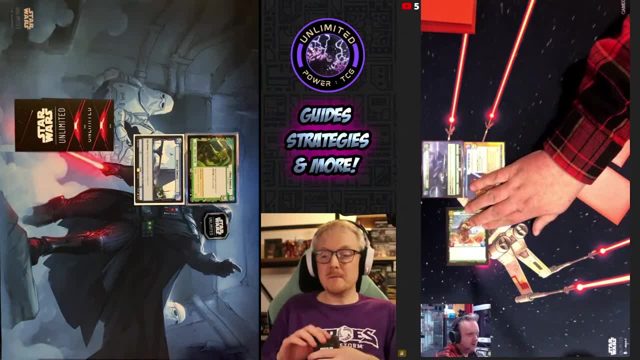 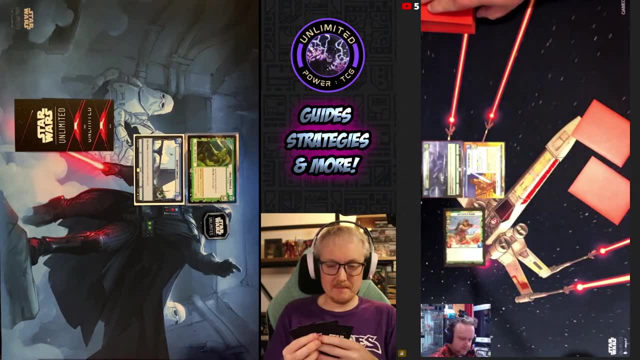 marine down. Oh, nice card. There's no special text. Here's a 3-3 ground arena. I have nothing else to do, so I will pass. So next battle round: Yep, Here we go. What do we have? Do we call them battle rounds Or turns? 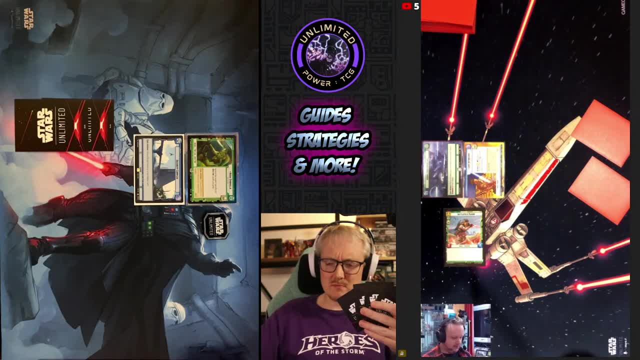 Turns rounds something like that: yeah Okay, All right, Here we go. Oh, I'm going to resource one, All right, Oh my goodness, Oh my goodness, I kind of want to keep all of these. 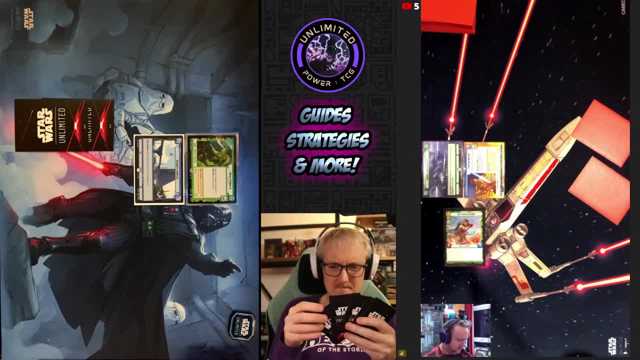 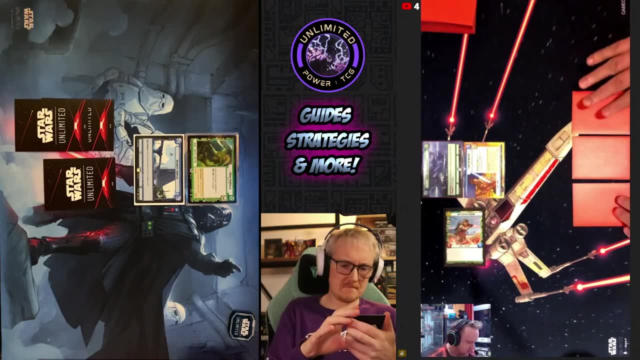 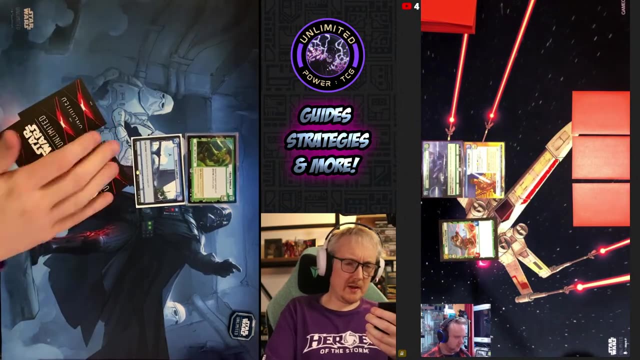 All right, I'm going to resource one, But if in doubt, always do that. So let's play that down and ready up And you have the initiative. So what would you like to do? I'm going to play at top three. I am going to play Ezra Bridger. He's a 3-4 force rebel. 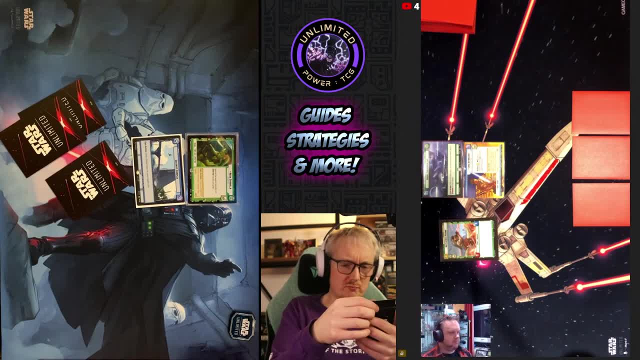 specter When this unit completes an attack. look at the top card of your deck. You may be able to use it as a weapon. Yeah of your deck. You may play it, discard it or leave it on top of your deck. 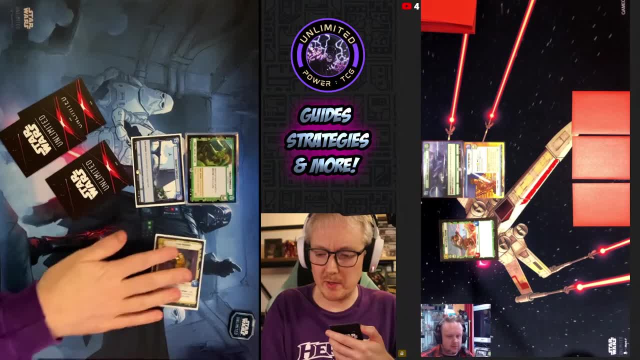 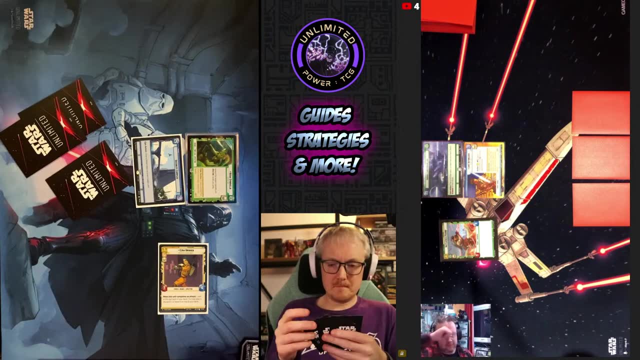 You put your infantry on the left, so I will put mine on the right and then we will match up on the street. Yep, that makes perfect sense. I was going to suggest the same thing if you weren't going to do it already, so that works Cool. 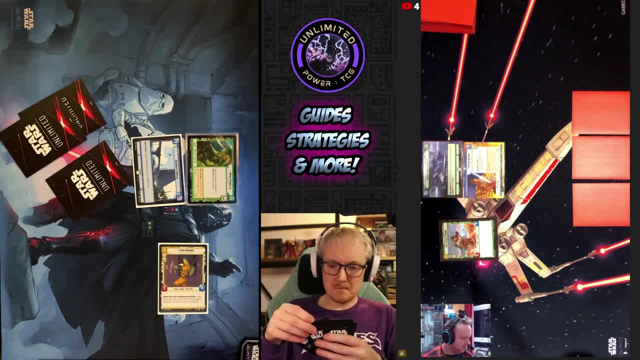 Excellent. Ezra is mildly annoying. I can't kill him this turn because he's a 3 drop and I'm well. he's a 3 cost and I'm a 2 cost. so how do I wish to do this? I think I'm. 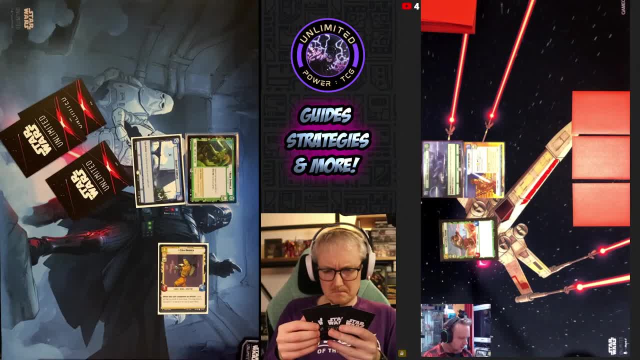 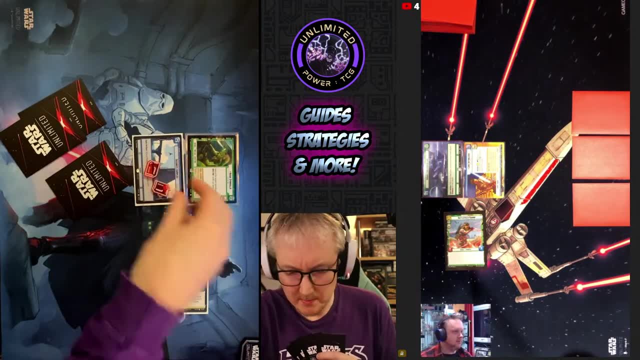 just going to do. 3 to your base- Perfect. May as well start the chip damage eh. 3 to the base, Down to 21.. I will take initiative, Yep, because you've got nothing left to do. that makes perfect sense. 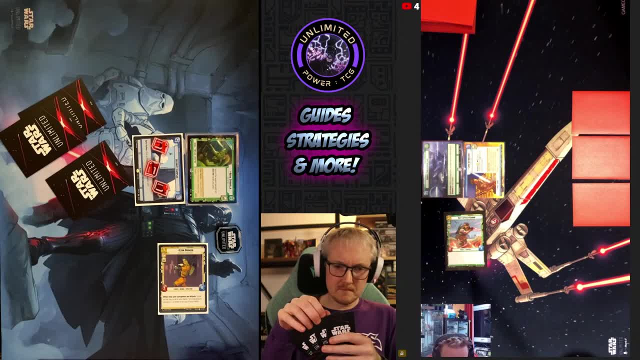 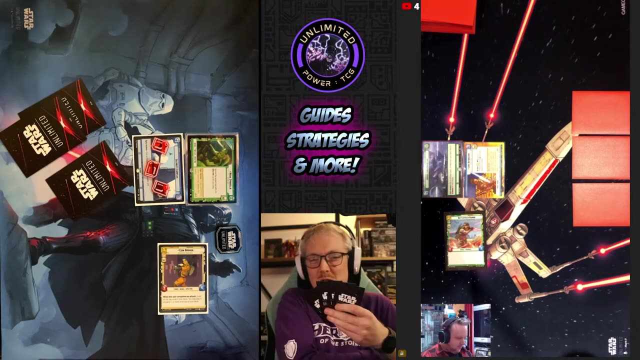 Hello, Phil, Philip, Philip, Arrigo. Yeah, Philip is the guy who's coming all the way from Baltimore to go to our GT here in Scotland. Awesome, Yeah, That's dedication. I was going to say we need to get like a little. 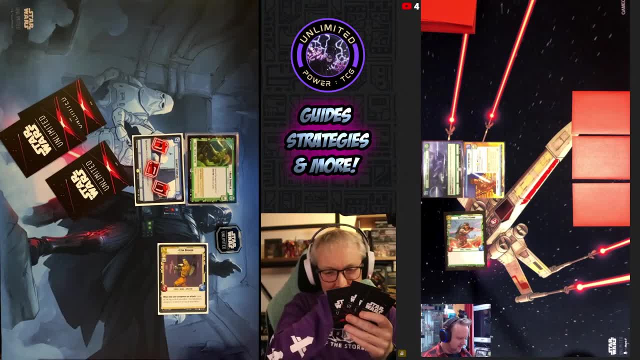 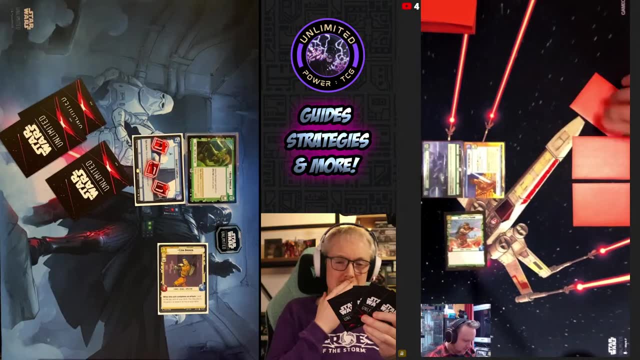 bottle of whiskey or something for the person who travelled longest to the GT. That's not going to work. Oh, I've messed this up slightly. Oh well, fine, We'll deal with it. So let's pay 2 to play. 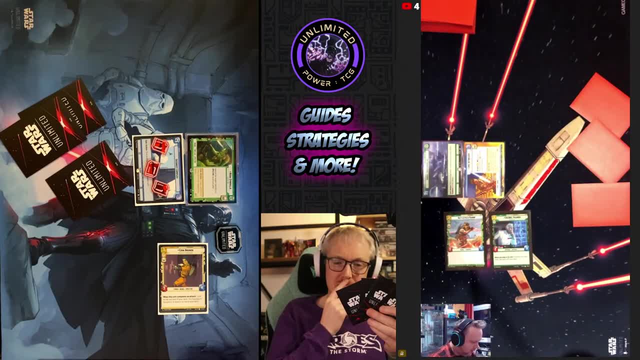 a Colonel Yalarin, who is a 2, cost 2-3. when you play a green unit, including this one, Heal 1 damage from your base. I've not taken any damage, so I won't heal any. That's fine. 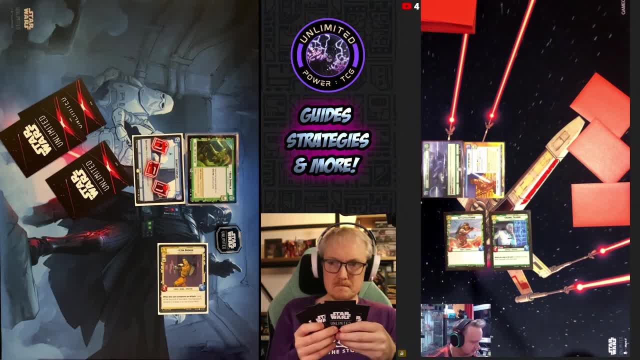 And I can't use Luke to give him a shield token because he does not have the heroic aspect icon. So I now have nothing left to do this turn. I will pass. Okay, Draw 2 cards. Yep Oof. Well, we know what's going down. 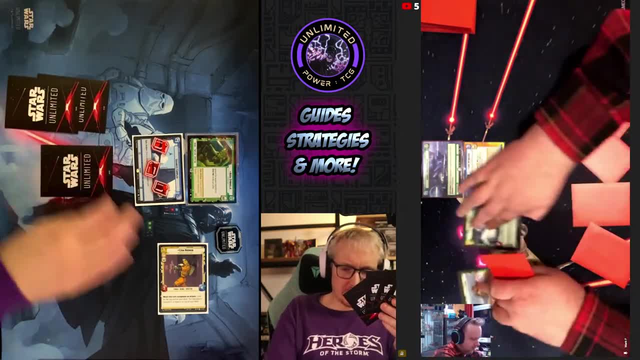 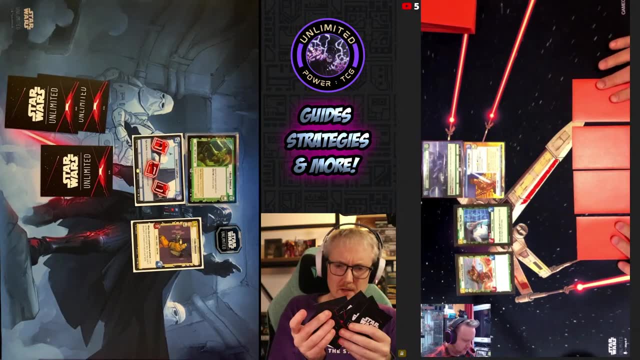 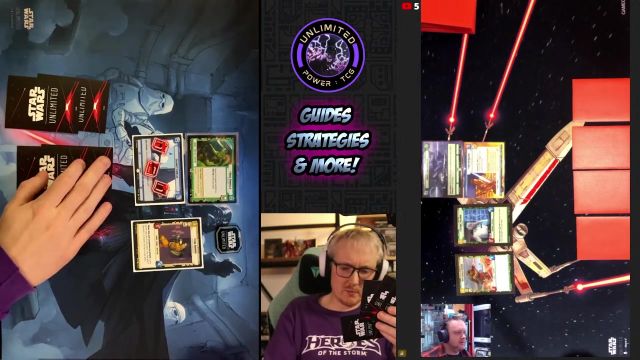 there, That's nice and easy, Cool, Ready up. Let's ready up. I have not had the greatest start here. I will I'll resource this and then I will pay 4 to put Kanan Jarrus into play. 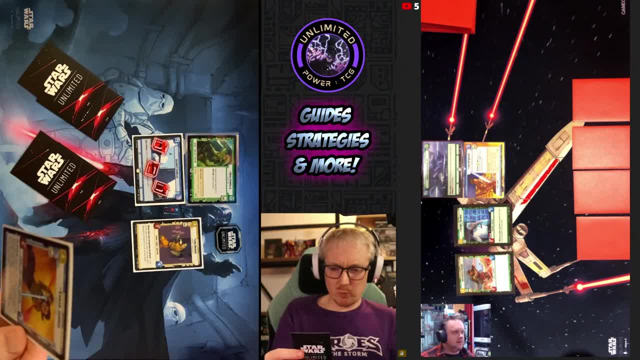 He is a 4-5 Spectre On attack. you may discard 1 card from the defending player's deck for each friendly Spectre unit. Heal 1 damage from your base for each different aspect among the discarded cards. I know it well. yes, 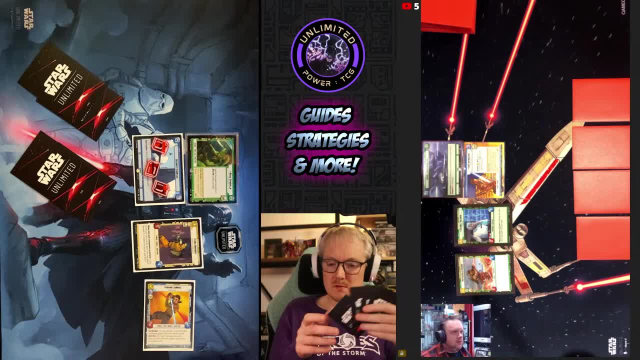 It's quite a good early game drop. Not bad, Not bad at all. Um, What am I going to do? first, You could kill either of those with Ezra and take a bit of damage in return. Um, So I think I'm going to. 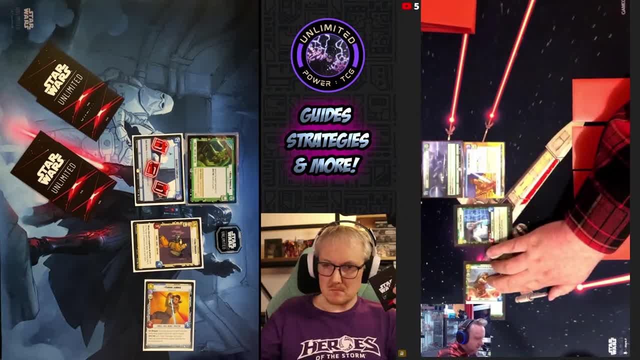 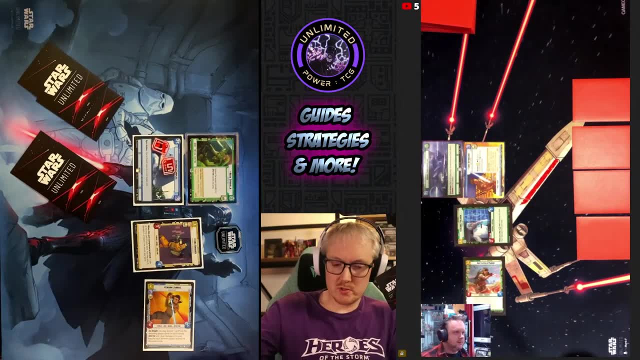 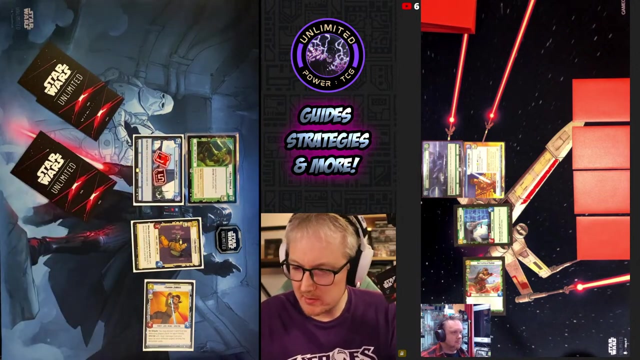 I'm going to have to do 3 to base of the Battlefield Marine first off. 3 to my base. yeah, Yep, Okay, I will then use my energy- Sorry, I'll use my security complex- to give a shield to Ezra. 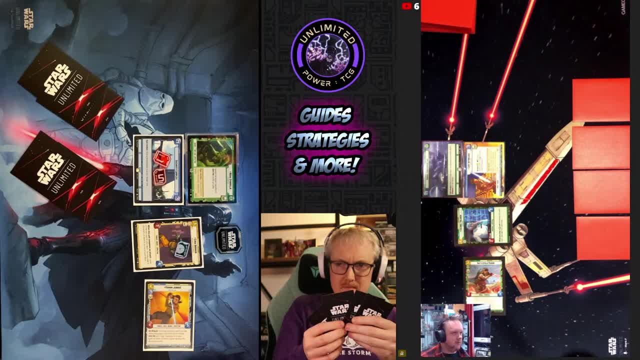 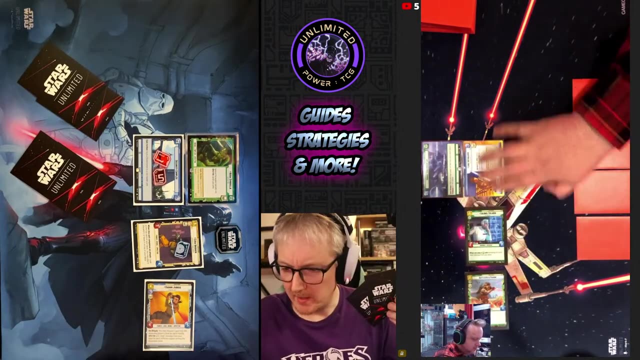 Okay, That seems reasonable. Alright, In that case, you're going to attack one of them and take no damage in return, so I might as well do 2 more to base with Colonel Yelarin. Okay, And then I think I will attack. 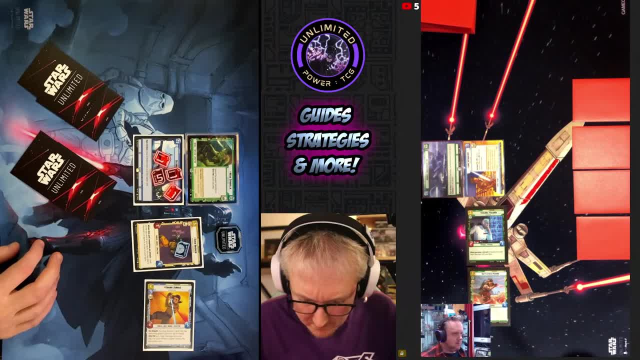 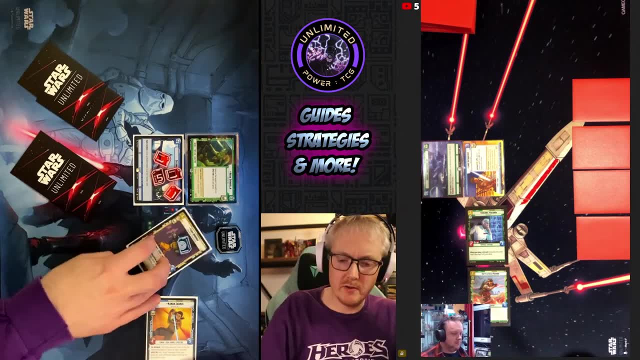 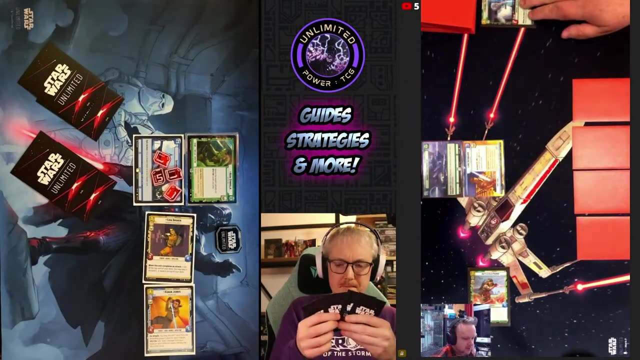 Um, I think I'll just attack Yelarin's Yelarin with Ezra. Yeah, Okay, So Ezra loses his shield and Yelarin dies. Yep, Horrible, ignominious death, Worthy of an Imperial Intelligence Agent. 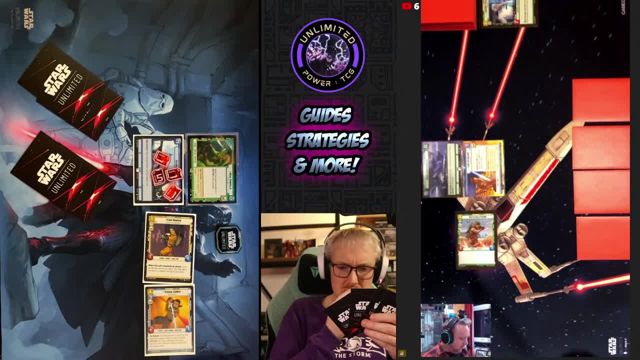 Such as he is: Okay, Uh Right, You're all tapped out. You've got nothing left to do, must be: Uh, I've still got 4 resources to play, so I will spend all 4 resources and play a Bright Hope. 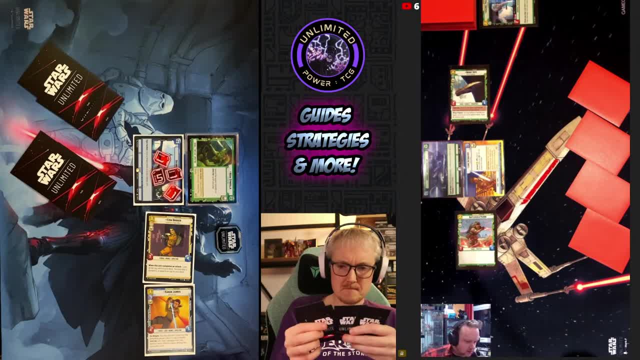 Ooh, Bright Hope's a forecast Command Heroic ship, that is 2-6 Sentinel. Uh, when played, you may return a friendly unit- Uh, sorry, a friendly non-leader ground unit to its owner's hand. If you do so, draw a card. I do not wish to. 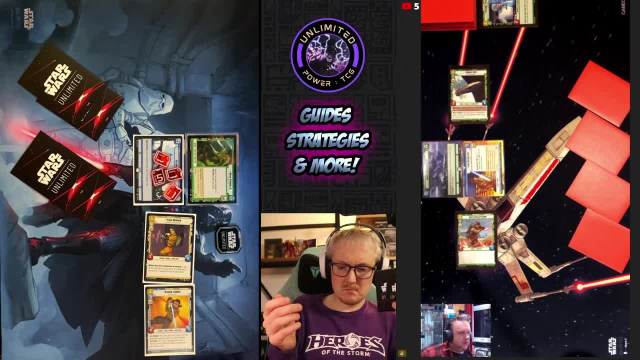 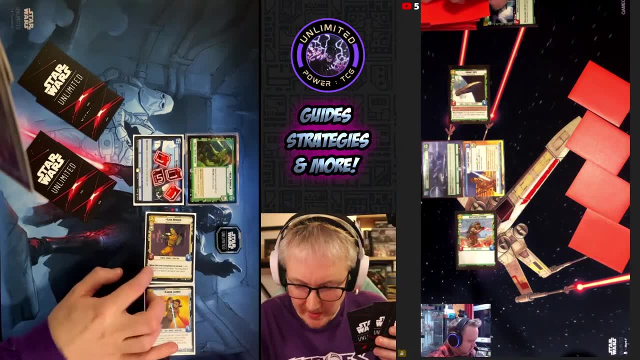 do so, Okay. Uh, You're up, I'll take an issue, Yep, And I'll pass, Okay, Two cards. Oh sorry, when Ezra played, I was allowed to look at my top card in my deck And, Uh, Yeah, sure. 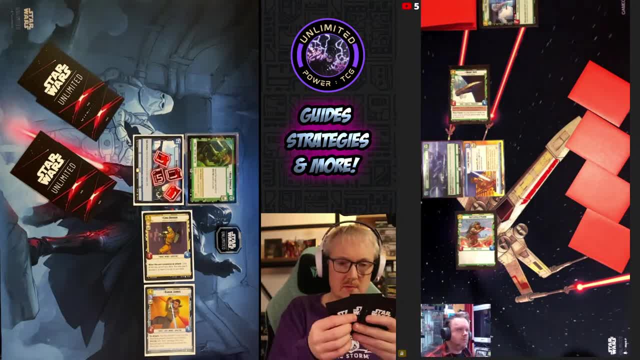 I can play it, discard it or leave it on the top. I'm happy to leave it on top. So when played, or on attack completion or something, isn't it? Uh, when this unit completes an attack, look at the top card of your deck. you may play it. 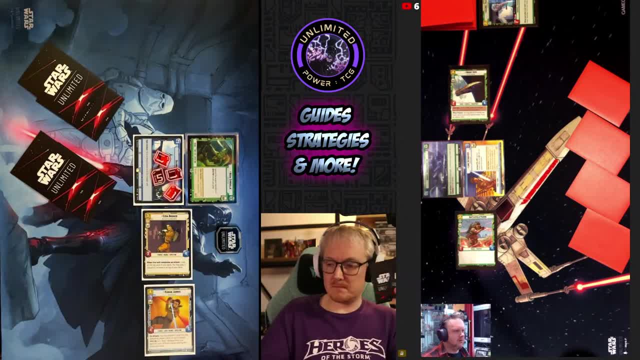 discard it or leave it on top. Yep, You couldn't have played it because you didn't have any resources left to play it, so you could just have left it. or Yeah, I'm gonna leave it because I fancy getting that card. 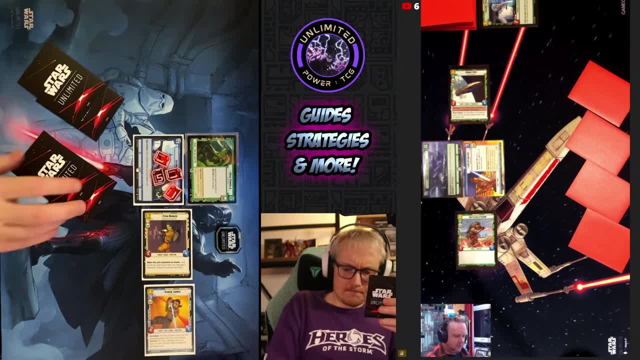 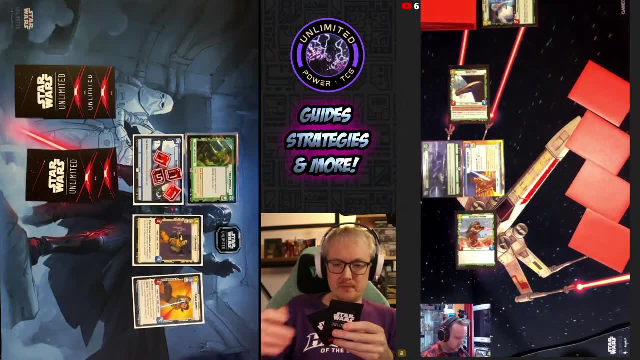 You're happy with it? Yeah, Okay, cool. Uh, you took the initiative, I've passed, Uh, so draw, Draw 2.. Okay, Oh, I untapped by accident for soups. Hmm, I'm gonna be on 5 resources. 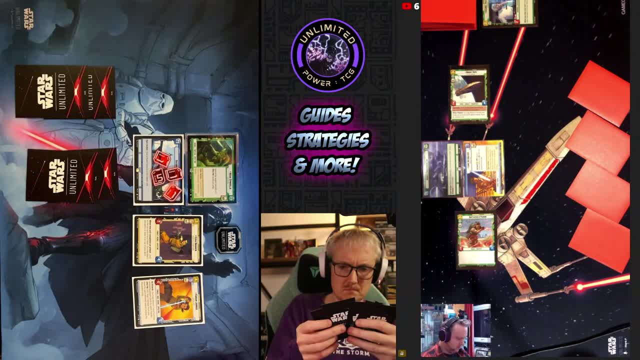 So what do I wanna do? I think, realistically, I wanna do that. I have quite a Ah. Every single card I've got I'd like to keep, but obviously I need to get one down for resource. Yeah, I'll save that for later, I think. 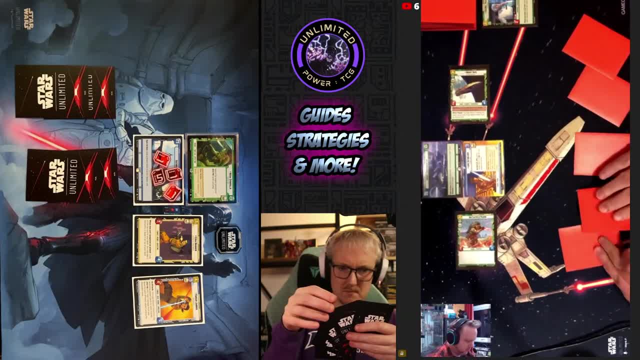 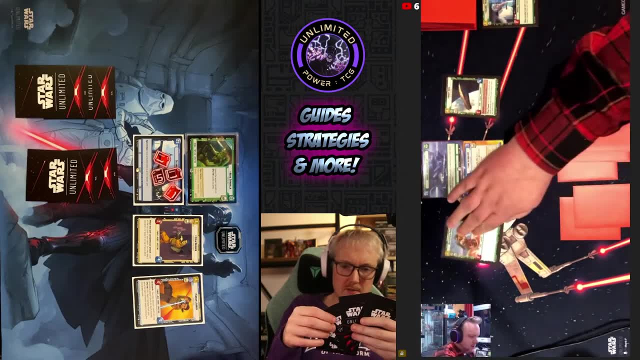 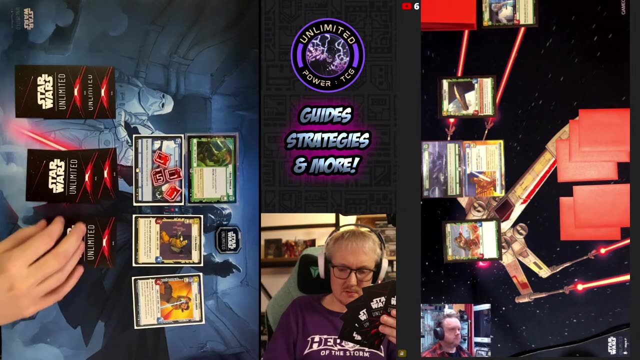 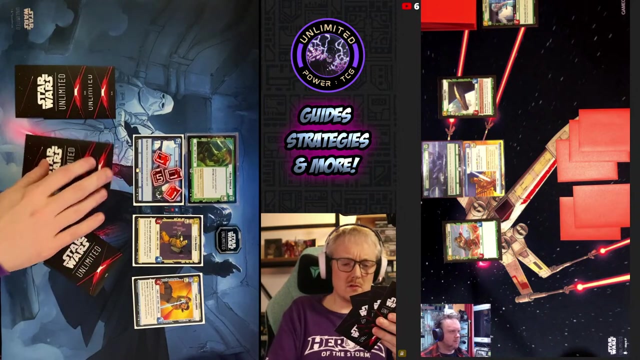 So let's resource this one and ready up, I guess I'm. It's tough, Really tough. I guess I'm resourcing this one And I will start by playing 3. To put a wing leader into play, That is a 2-1 rebel. 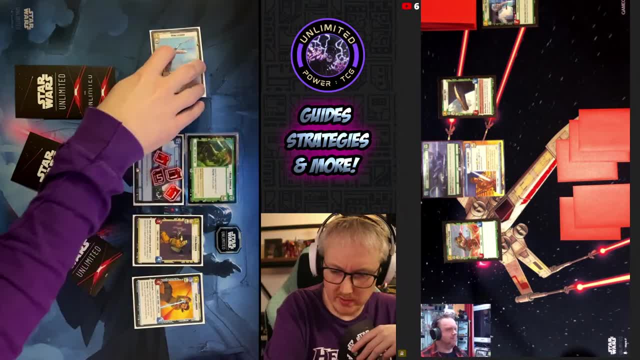 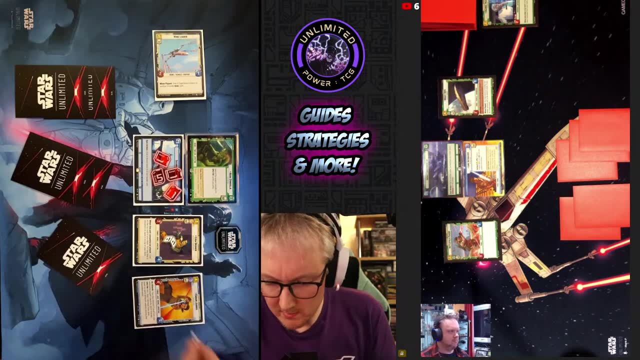 spaceship. Uh, I get to give 2 experience tokens to another rebel unit. Let's go ahead and give Ezra one And let's give Kanan one. No, it doesn't say that. It says: give 2 experience to a rebel unit, Okay, well then, we'll give. 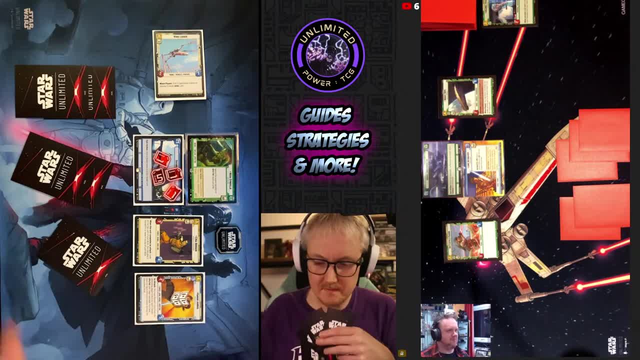 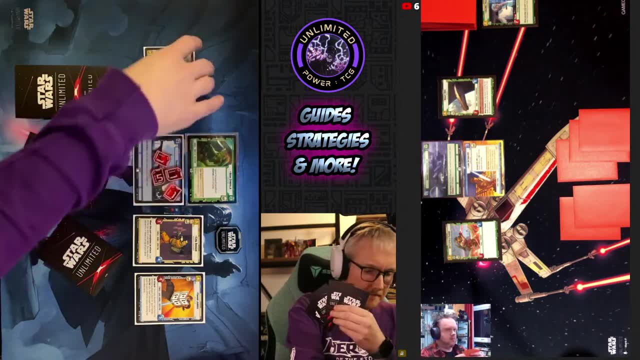 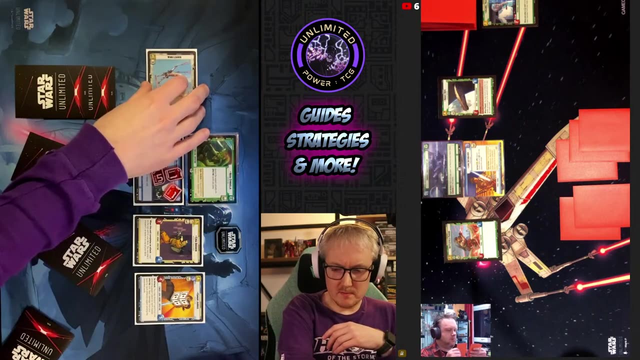 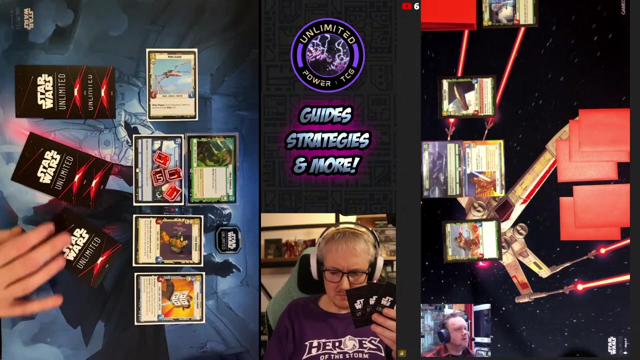 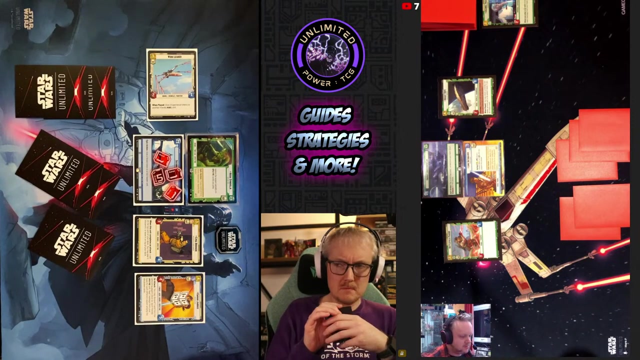 both to Kanan. That is much, much worse for me. But, yes, okay, fair enough, Right? Hmm, Puts him on 7 health, Yep, 6-7. Right, Alright, well, let's do the thing. 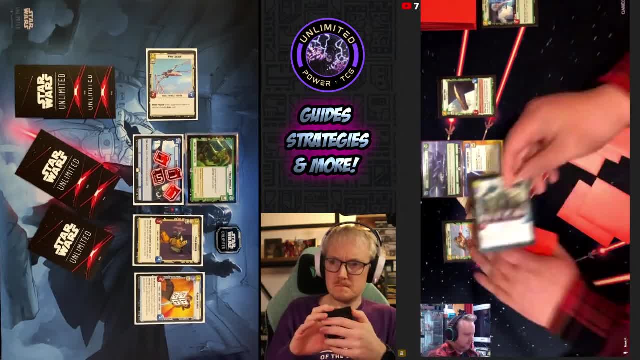 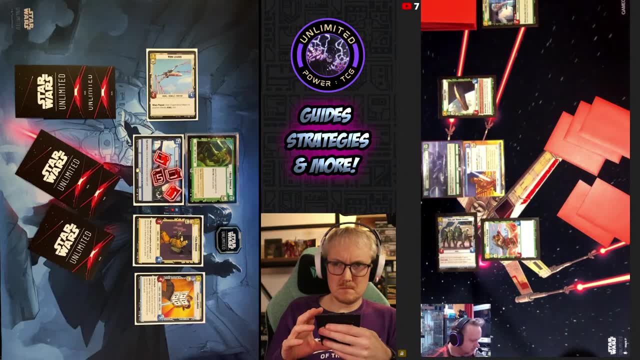 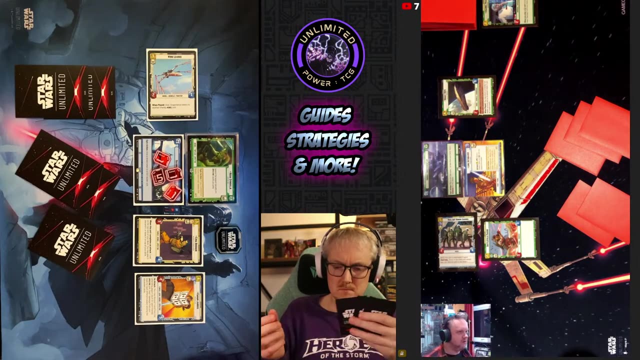 I will pay 5.. To play a Vigilant Honor Guard: 5 cost. Vigilant Heroic 4-6 Rebel who has Sentinel as long as he is undamaged, 4-6.. Okay, so I can still. 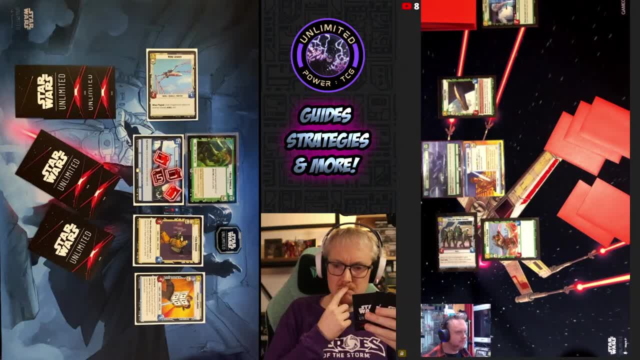 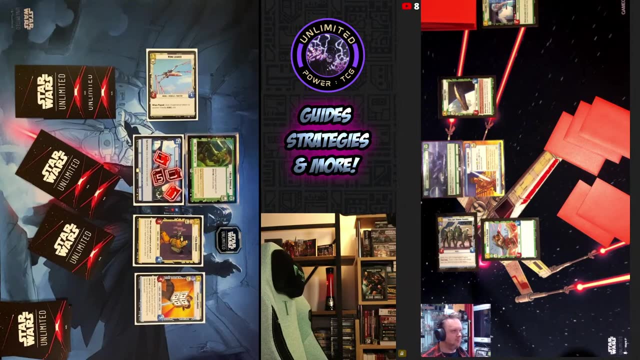 kill him straight away. Um, Hold on, I think I hear a kid crying. No worries, Let me just check. Yeah, do what you need to. I will not break out my joke, but my joke is filthy and is not suitable for stream. 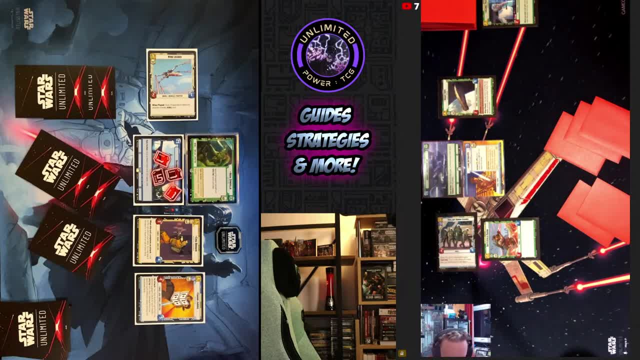 Hello, 7 people in chat: The Krushexer, Stephen Clancy and Philip Arago. As previously mentioned, there must be some of the people who have not yet said anything in chat who are watching us, So thank you, hello. 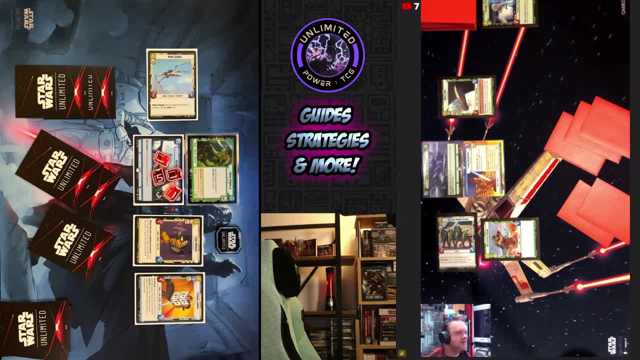 and welcome, if we've not already greeted you. Uh, Currently damage on base would appear to be in my favor, but at this point in the game it's still very definitely anyone's game, So we'll see how it goes. Unlimited power. 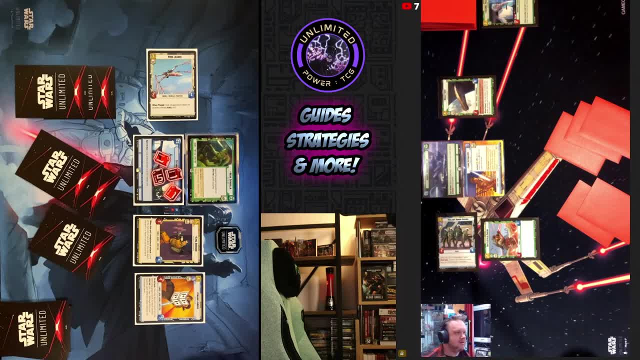 I do like that Vader mat. That Vader mat is very nice. Having said that, I thought I was settling with the X-Wing mat. but the X-Wing mat is also very nice indeed. I like the way it makes the little red laser blasts on the mat, kind of. 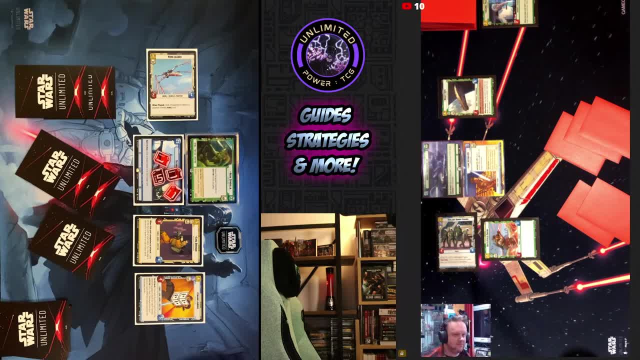 glow- or look like they're glowing on the stream camera Building some death company. I'm going to go back and look at the map. I'm going to go back and look at the map. I'm going to go back and look at the map. 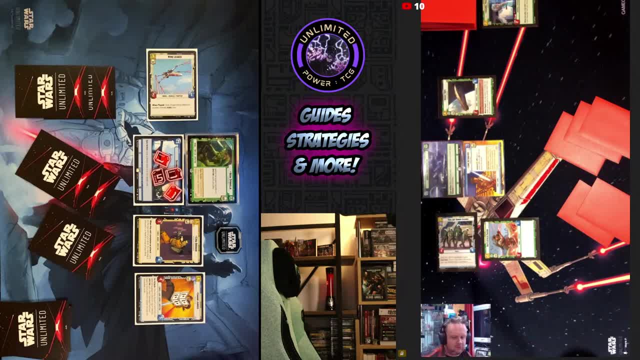 I'm going to look at the map. Jump pack, firstborn or other sort. How are you equipping them? if I may be so bold: Power fist, inferno pistol or something a little more interesting? perhaps I've got far too many death company. 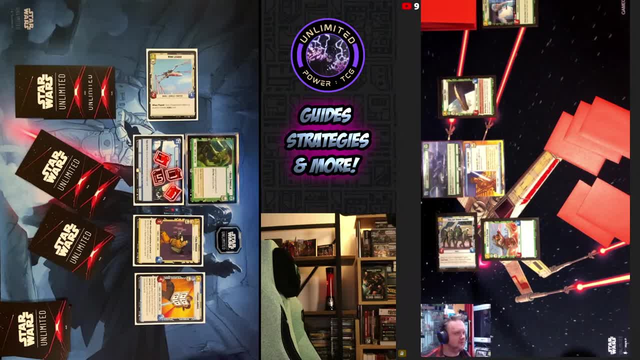 And I've broken their arms off and re-glued different arms on them many times, far too many times, over the years. I'm going to go back and look at the map. I'm going to go back and look at the map. I'm going to go back and look at the map. 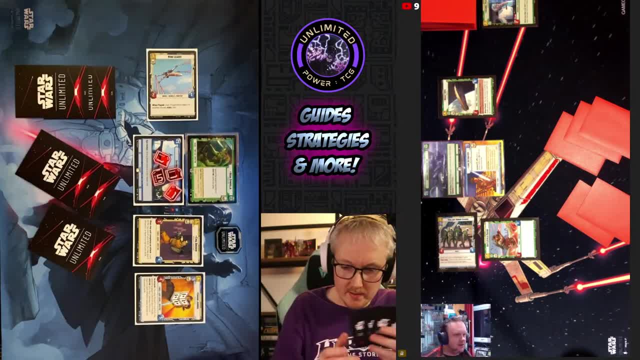 I'm sorry. you do what you've got to do. I'm sorry you do what you've got to do. Yes, I was going to play Right, so I've just played this Sentinel and is now in your action. I feel like I should kill it. 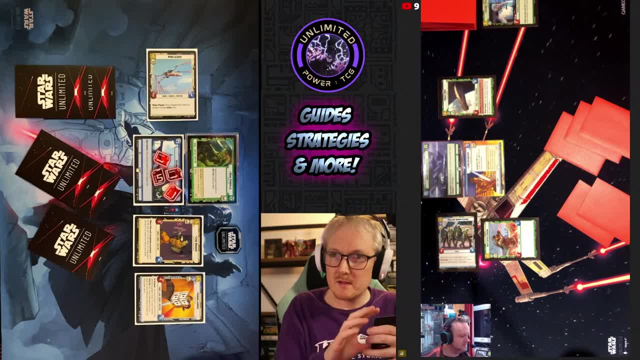 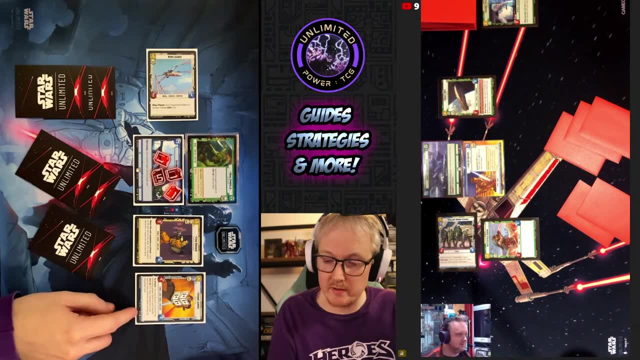 I feel like I should kill it. I mean, you don't have to. I know I can't though. I know I can't though, Because I've got six damage on Kanan. So I'm going to do a little bit of a. 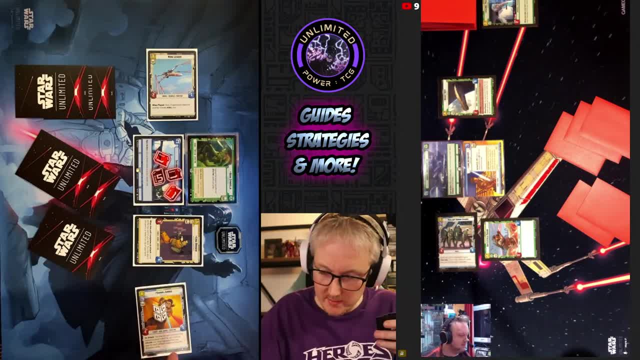 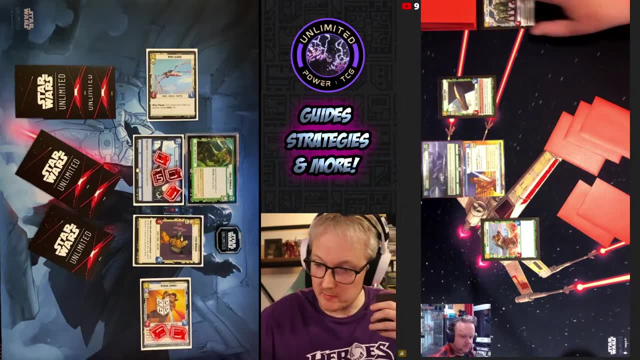 Yeah, let's kill it. So I'll attack with Kanan. Alright, You take four, I'm down to three. I'll just put three on him to see he's good. Well, I could just put the four on him actually. 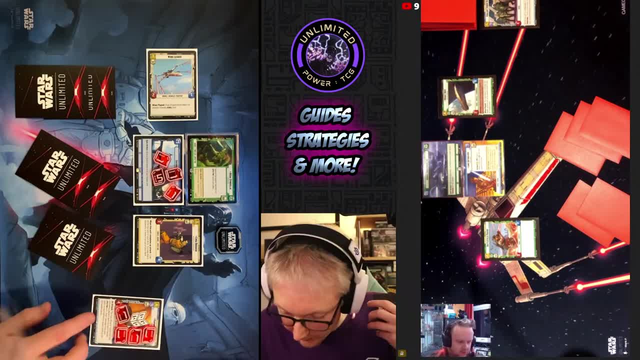 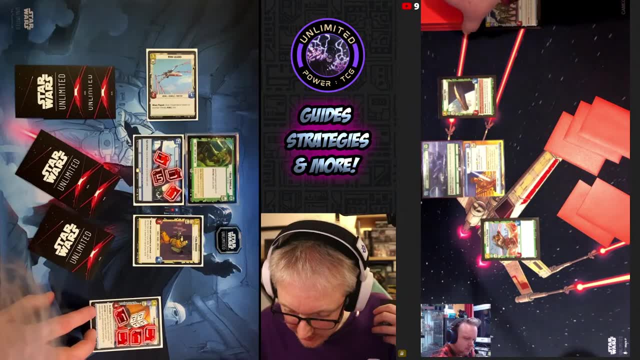 Path is a plaza pistol. Okay, interesting choice On attack: you may discard one card from the defending player's deck for each friendly spectre unit. So you need to discard two cards and tell me how many disproving aspects that is You have to. May means it's optional, so it's your choice. 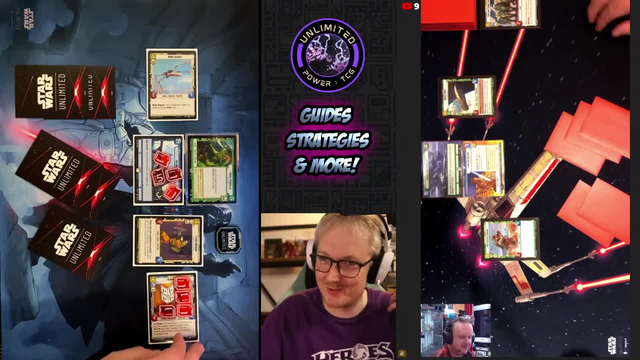 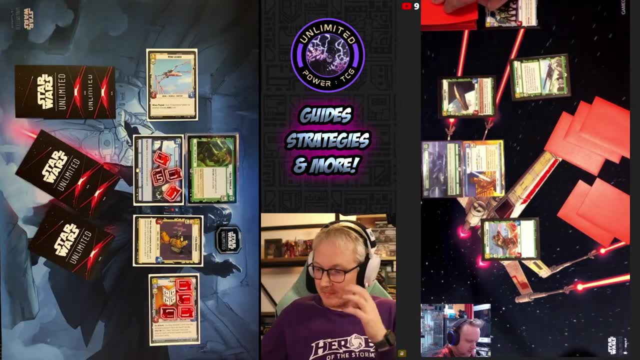 as to whether you do it or not, You're definitely discarding two cards and telling me how many aspects, unique aspects- there are Two aspects off the first card and off the second card a third aspect. So I heal three on my base. 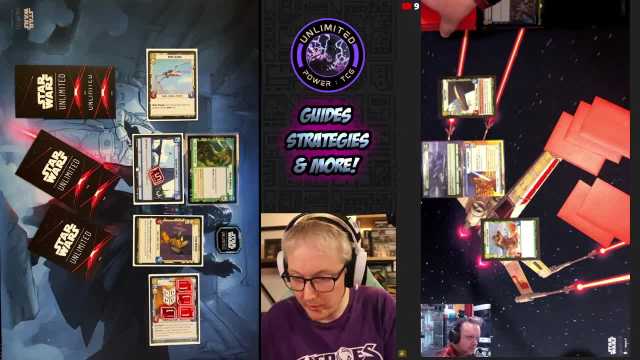 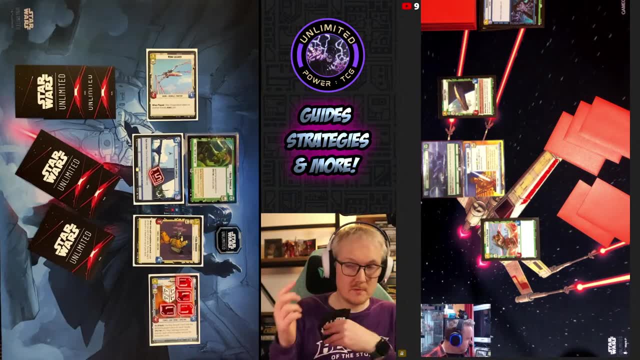 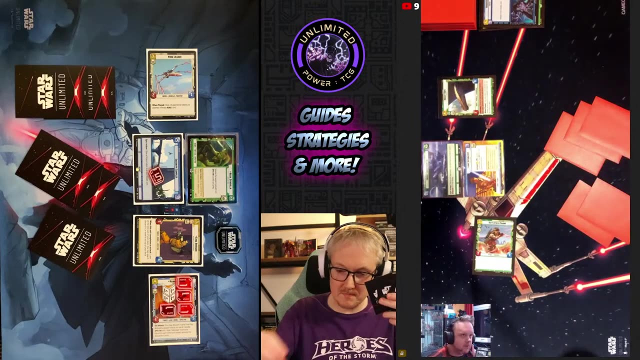 Alright, So Kanan is now a 6-3.. Mm-hmm. Okay, Right, Well, I think we're going to take advantage of this to kill Kanan with the Battlefield Marine. Epic mate, Cool. So he kills the Battlefield Marine. 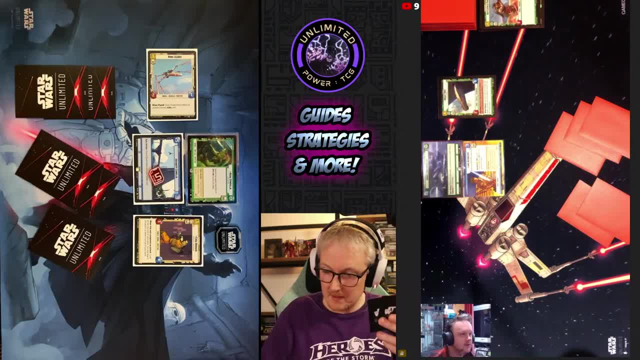 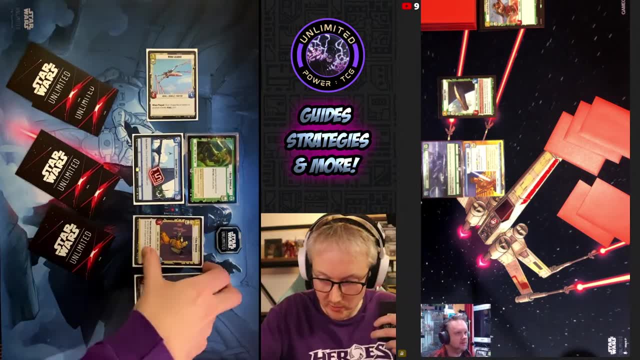 in his turn. Oh, absolutely, The Battlefield Marine's only piddly. Okay, I'll then spend two to give Ezra an Electro Staff. Oh yay, Attached to a non-vehicle unit, that gives him plus two, plus two. 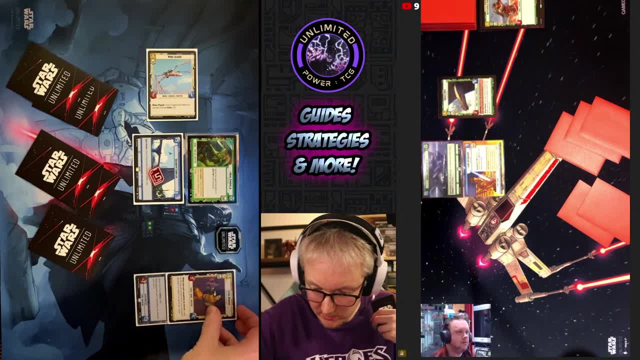 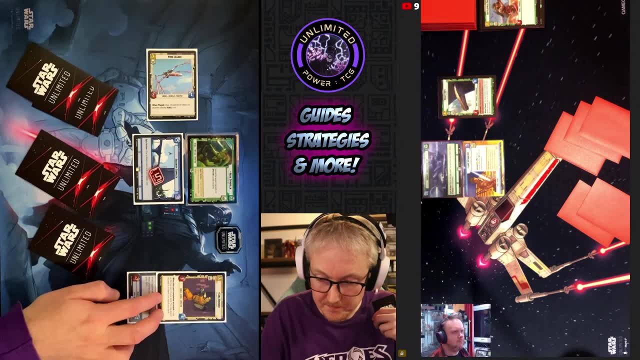 While attached, While this- While attached- Oh sorry, Attached- unit is defending The attacker, gets minus one, minus zero. Okay, Fair enough. So when you attack me, you lose one attack. basically Seems pretty tasty, Okay. 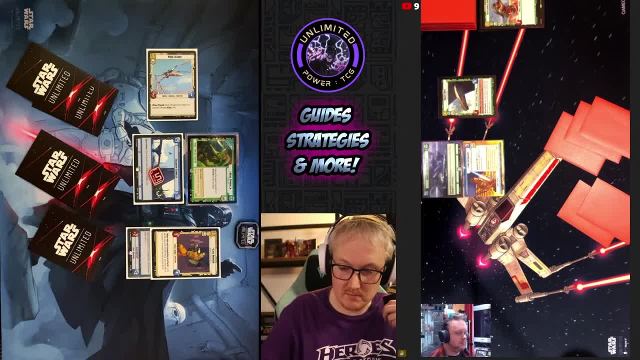 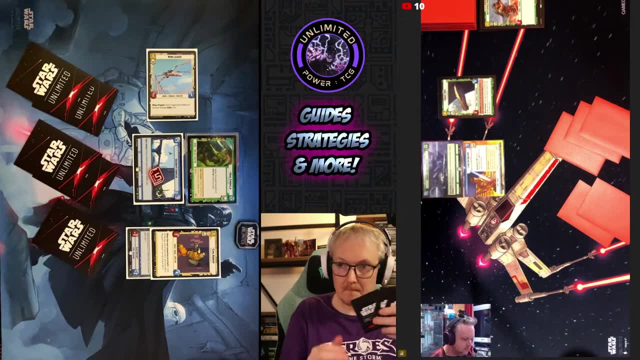 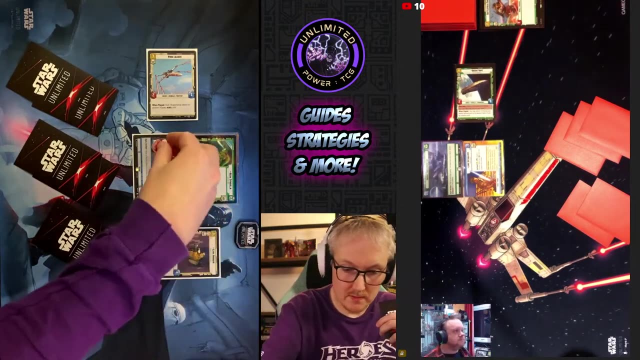 Okay, So he's a 5-6.. Yeah, Yep, Right, 5-6.. Fair enough, Cool. My Bright Hope is going to attack your base for two Perfect, And I guess Ezra's going to attack your base. 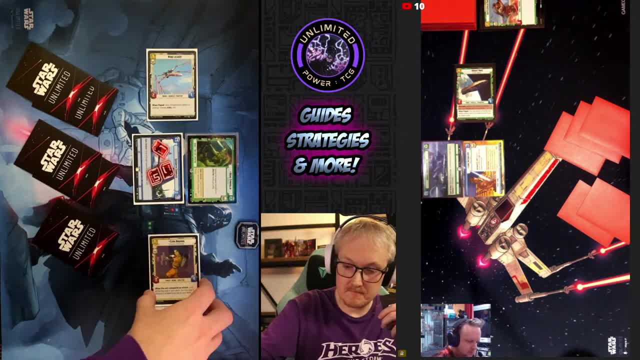 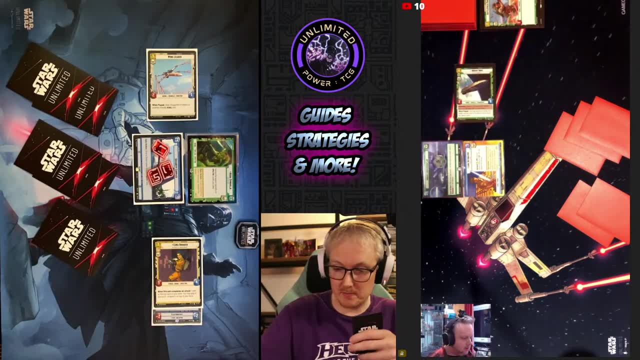 for five, Okay, And then I get to look at the top card of my deck And then I'll just put it back on the top because that seems fine. Rocking the Heroes of the Storm shirt. Great game, Abathur for life. 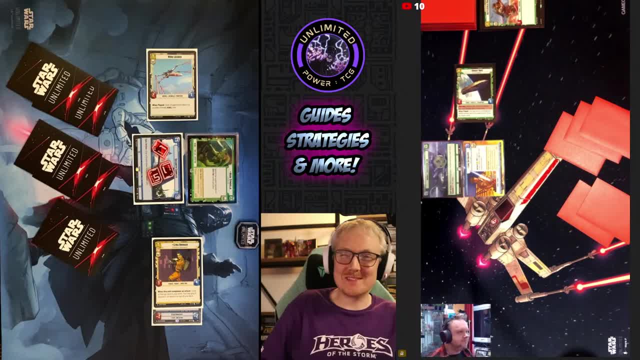 Cheers, Marius. Hey, Marius, Heroes of the Storm is like my guilty pleasure man. If you enjoy it, don't be guilty about it. No, but you know what I mean. It's the game that I always go back to, Marius. 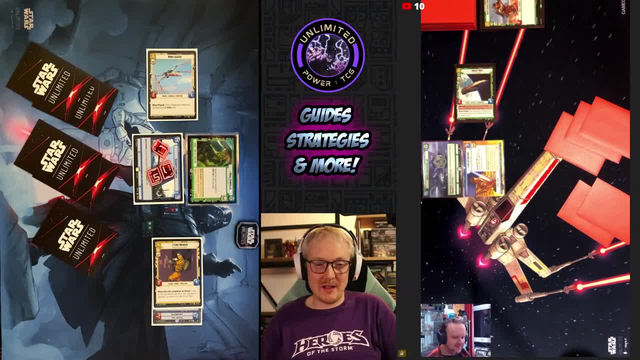 I need to get you added on a battle net. I play like one game like three times a week. Have you seen what they're doing in the next patch for WoW? No, I haven't been keeping up. So in the next patch for WoW. 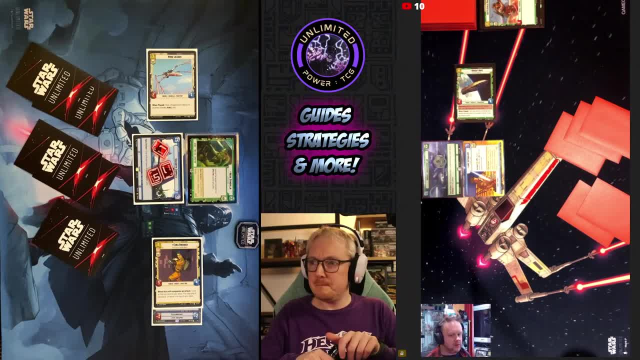 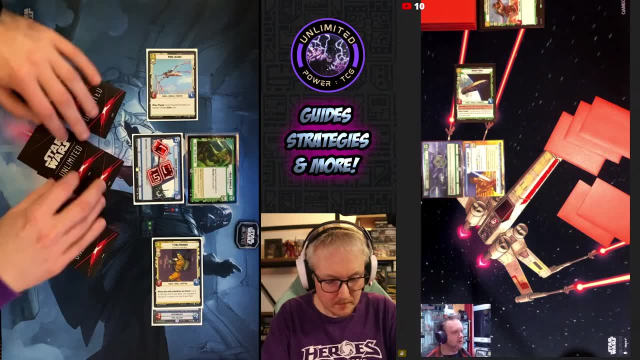 which is the patch before the War. Within the next expansion they are doing a time-limited event where you create a new character and level it from 1 to 70, all in Pandaria, and all the rewards and transmog stuff you earn during. 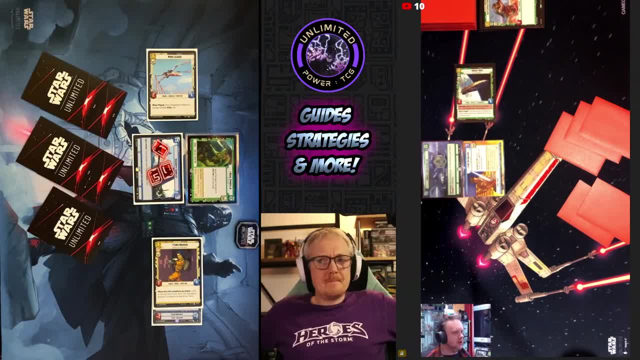 re-experiencing Pandaria from scratch all over again get transferred to your main account So you get a new character for later. Well, that's cool In terms of cosmetic rewards and toys and things like that. Oh cool, I did enjoy Pandaria. 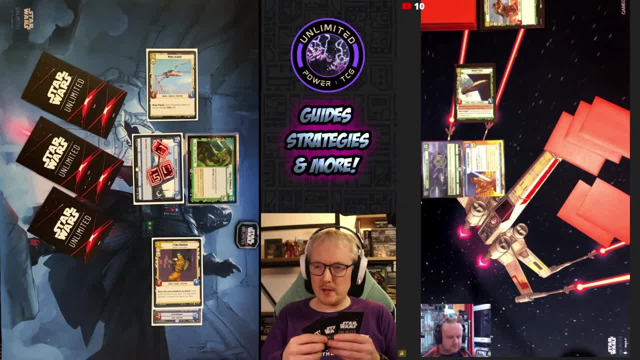 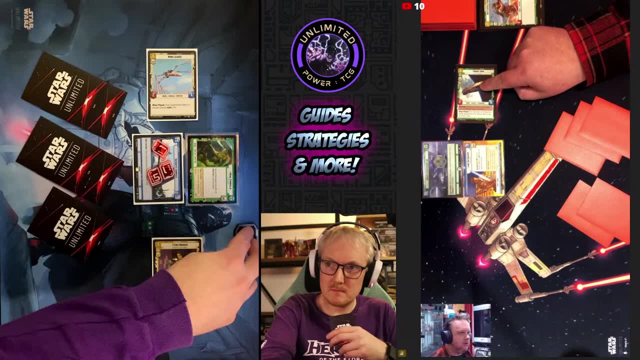 I love Pandaria. I think it's one of my favourite expansions, So it's your turn then. Anyway, yes, Have you got anything to do? Bright Hope has shot you for two. You have. Does Bright Hope have healing on it? No, 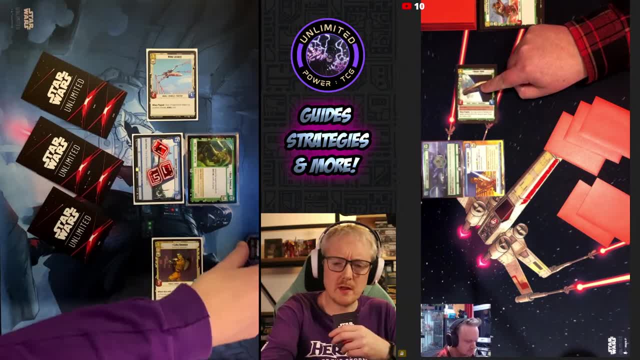 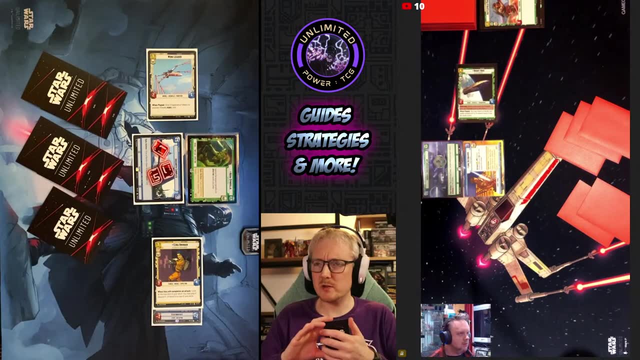 No, Oh, sorry. Okay, I thought it had to restore My bad. No, it's sentinel. Okay, so you shot me for two. I added the two. What's next Your action? I guess I'll take initiative again. 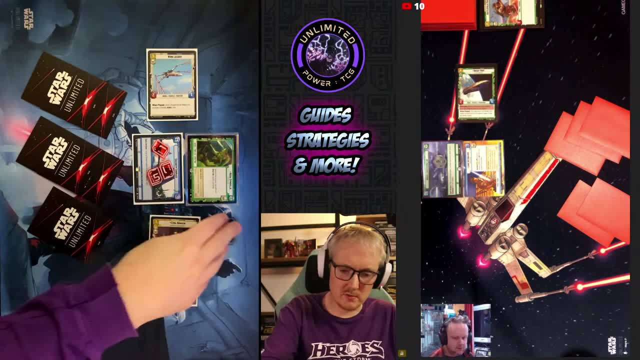 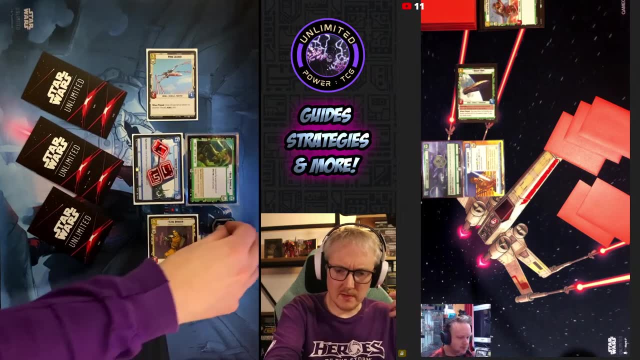 Sorry, I thought I was waiting for you to take initiative, but no, Okay, I'll take it again. You just did me for five, didn't you? Was that before or after the Oh, that was after the Bright Hope. 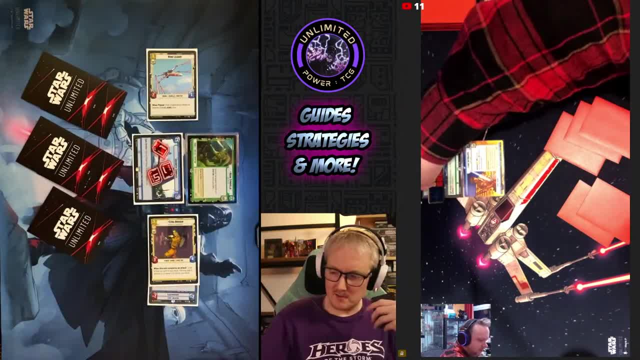 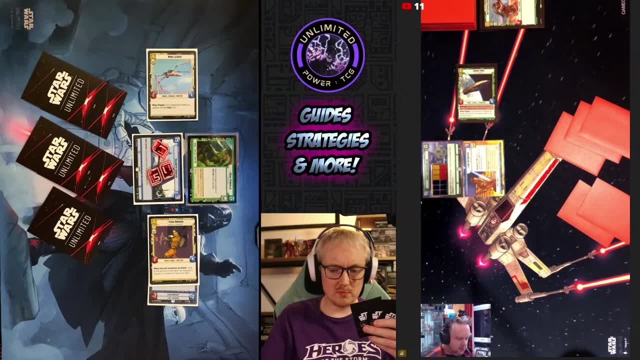 Yeah, perfect, Okay, sorry, I was waiting for you to take it. and then My initiative token is the Grand Admiral's rank insignia. Perfect, Okay, All right, So you pass and we move on. Yeah, next turn. 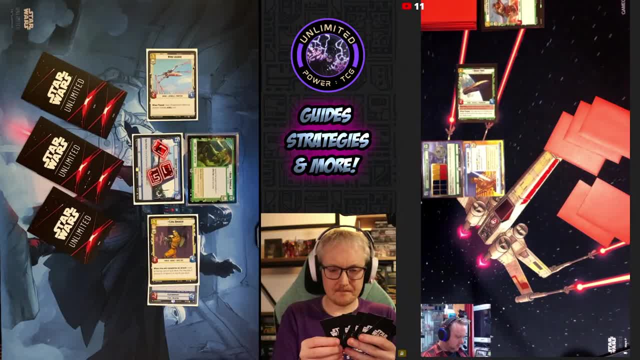 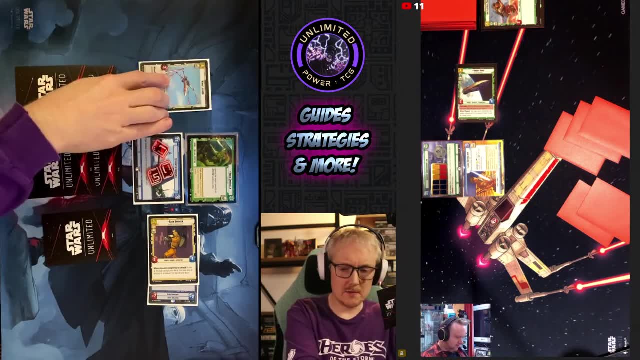 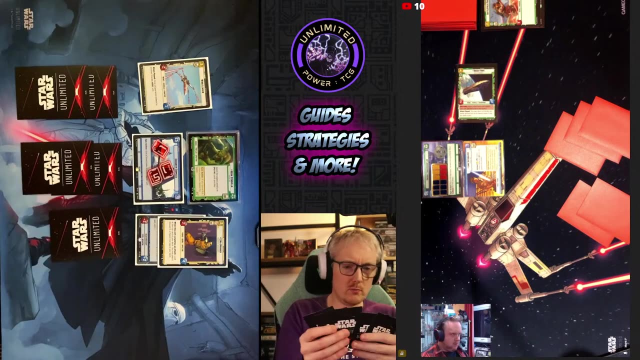 Okay, All right, This is what we wanted. Nice, Yeah, I got what I wanted there as well, actually. Okay, This'll be interesting. We'll see how this goes. Uh, I will. What's his attack rating? 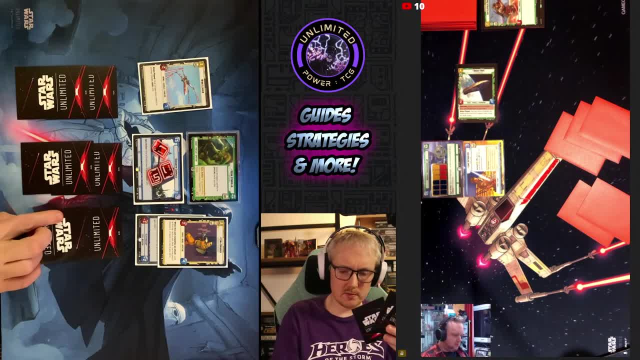 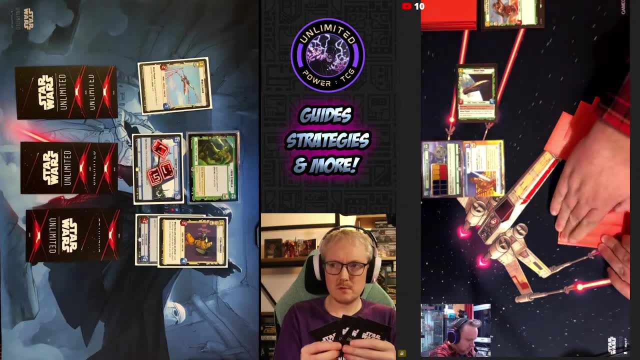 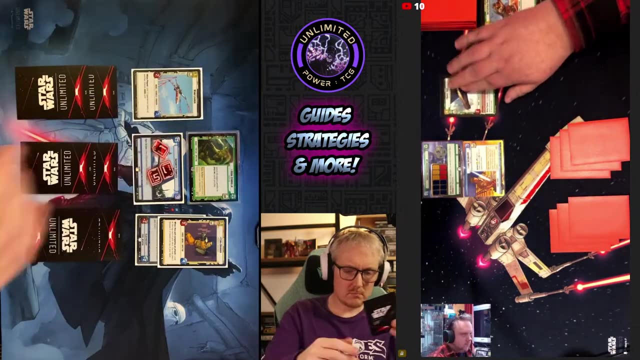 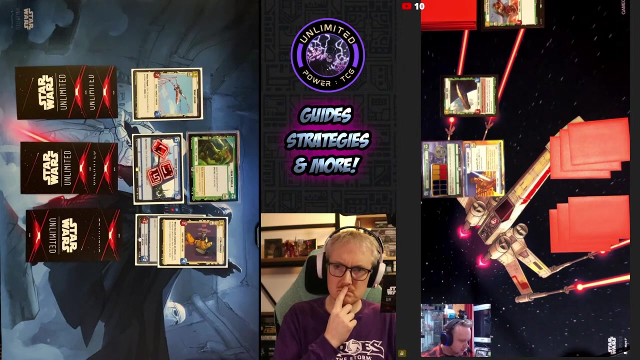 Five, six, This one, Okay, Six, yes, All right, let's resource that and ready up. Okay, Okay, Cool. What do I want to do first? I think I know what I want to do first. I want to. 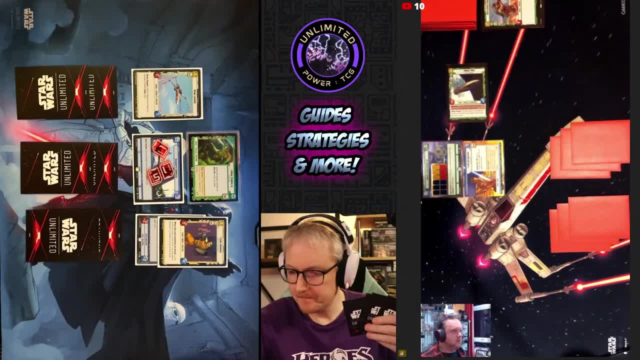 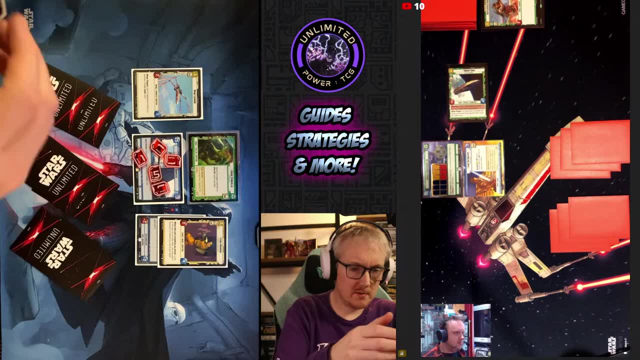 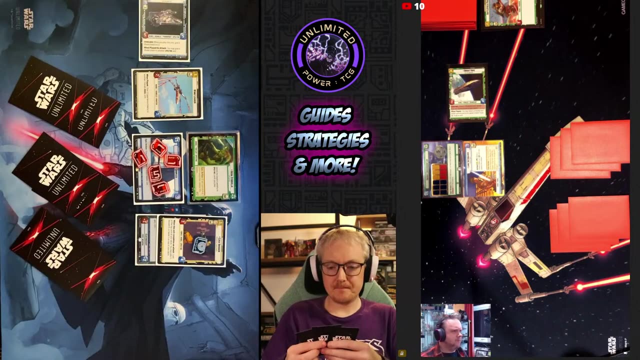 attack two to base with Bright Hope. Sure, Okay, I'm going to spend six Yep. Okay, When you arrive you may put a shield on another spectre unit. That will go on Ezra. It will Fair enough, No worries. 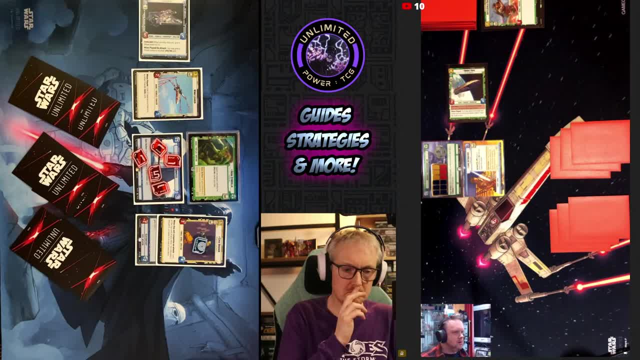 Uh, Five, six shielded, Minus one when defending. What order do I want to do this in? I figured you're going after him, so my vain attempt to keep him alive is to put a shield on him straight away. Okay. 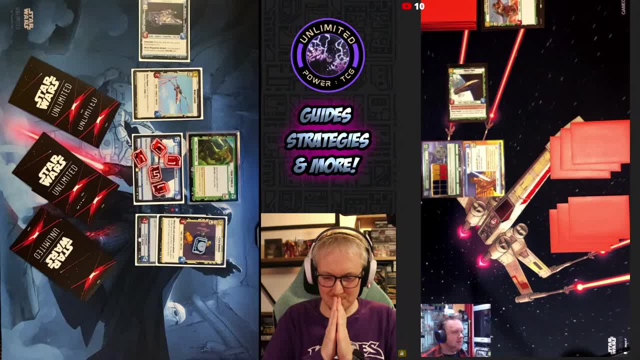 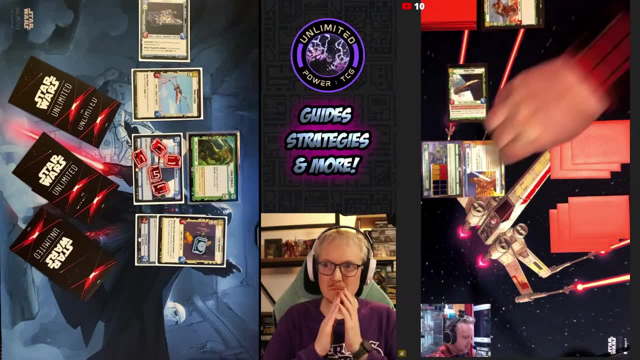 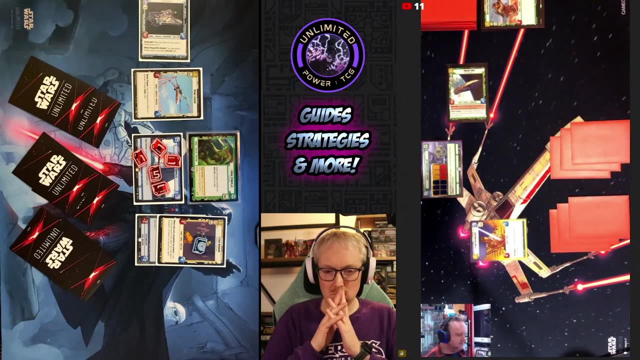 Six already, Yeah, Hmm, All right. Yeah, let's bring out Luke. All right, We are deploying Luke Skywalker, faithful friend, It's a four seven On attack. it gives a shield to anyone, isn't it? 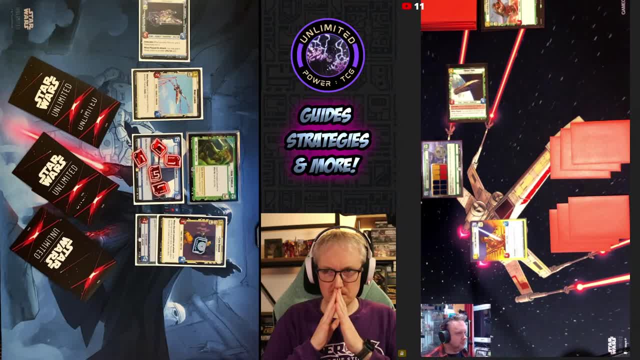 It's a four, seven A shield token, and there is, of course, no limits to the amount of shield tokens that can be on any given unit. Okay, let's go ahead and just hit him straight away for a five with Ezra. 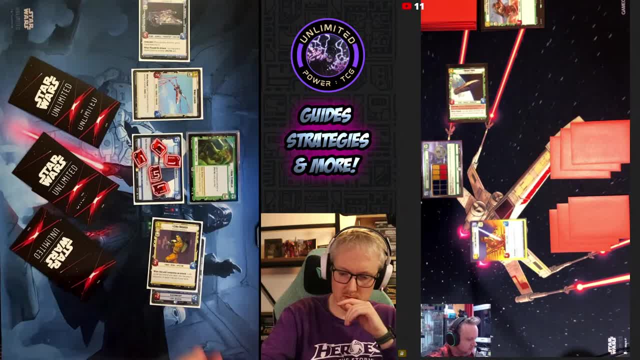 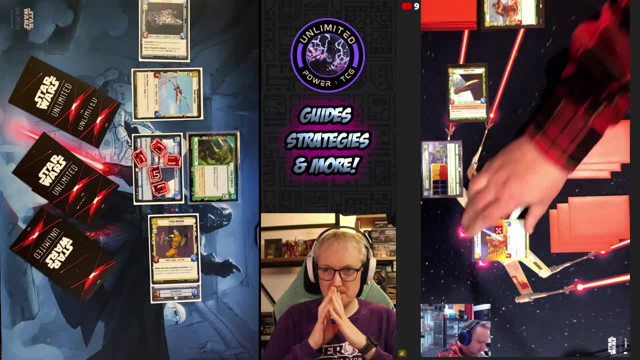 All right, you hit Luke for five And lose my shield And Luke pings off the shield. absolutely, That Is that. what you were expecting is what we call a result. So I'll pay six to play Obi-Wan Kenobi. 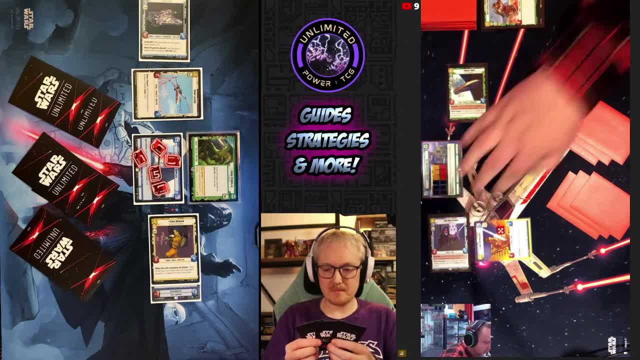 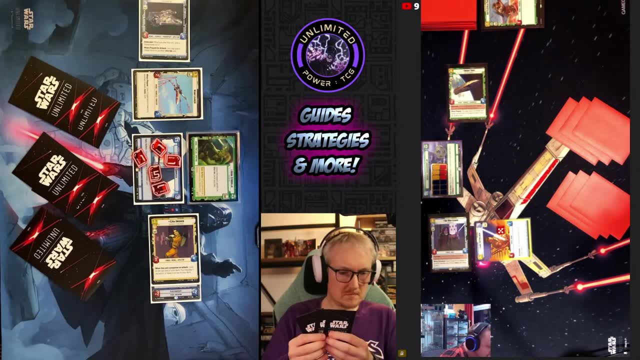 Ooh, very nice. Use a four, six sentinel: Vigilance and heroism. When defeated, give two experience tokens to another friendly unit. If that is a force unit, draw a card as well. Okay, I couldn't have killed him anyway. 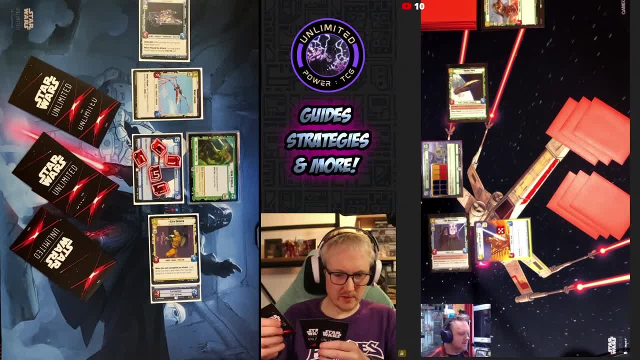 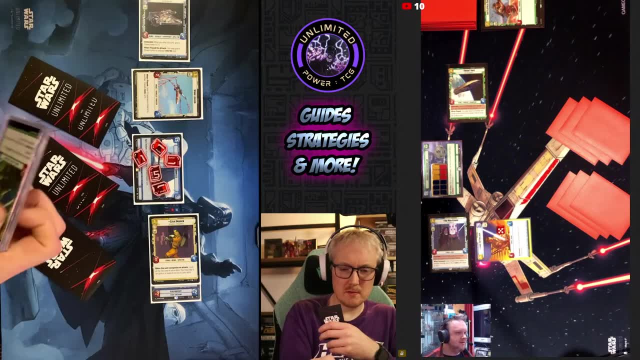 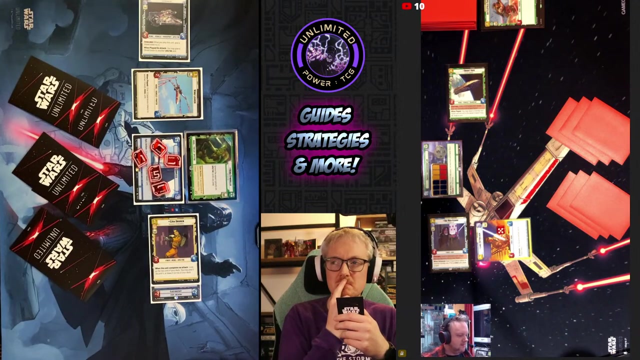 with Ezra, That's true, For whatever that's worth. And He does four, Hera does a six. Hmm, By Philip Hera she has to hit Obi-Wan, That's true. Is that the worst thing in the world? 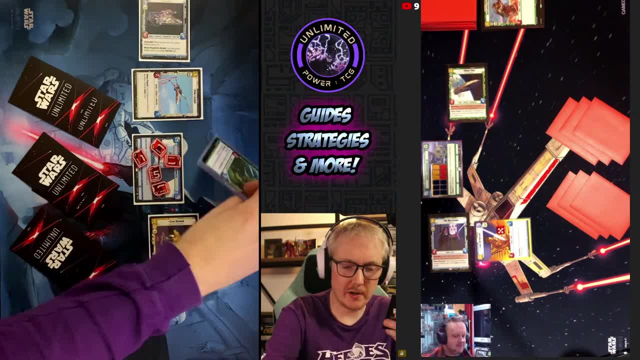 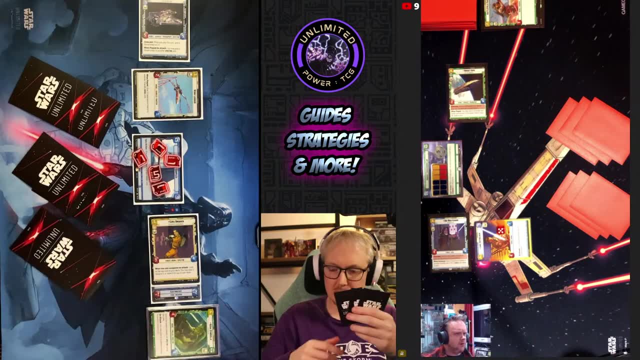 No, Okay, I'm gonna flip Hera over, Okay, So Hera deploys into the ground arena alongside Ezra. Yep, She's a four six And on attack, Gives an experience token to another unit. Yeah, that's pretty nasty, isn't it? 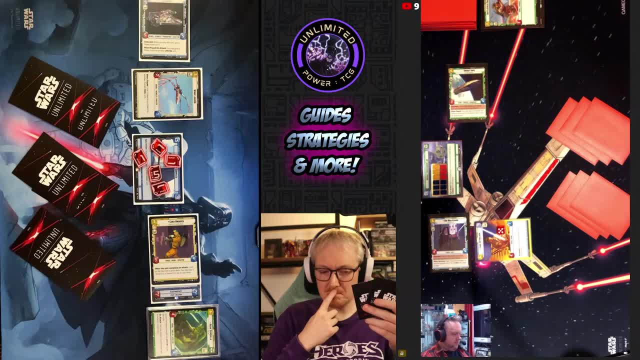 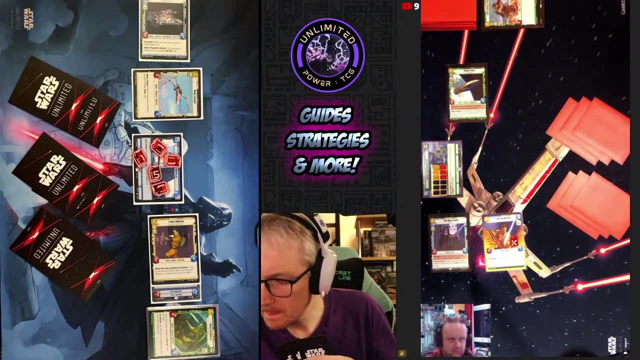 Okay, That'll build up unpleasantly. So Let's attack the base with Luke For four, Okay, And on attack, we will give a shield to another unit, which will be Obi-Wan. That's very nice. 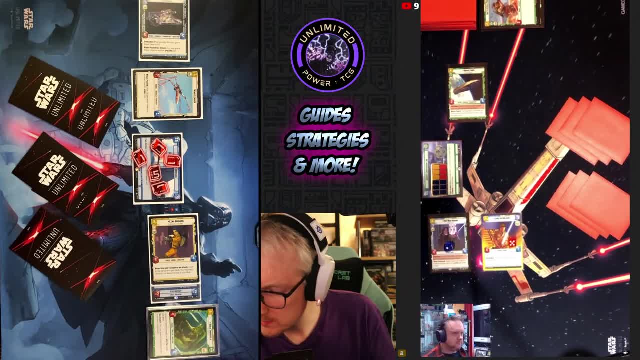 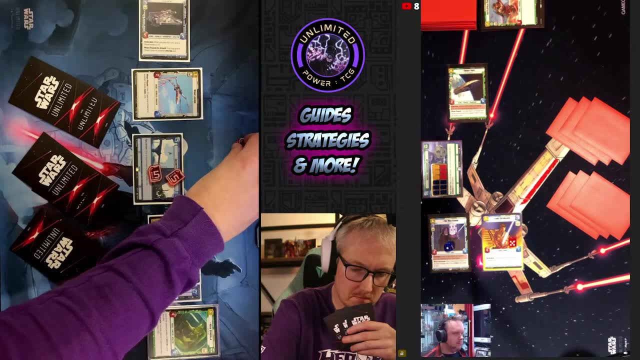 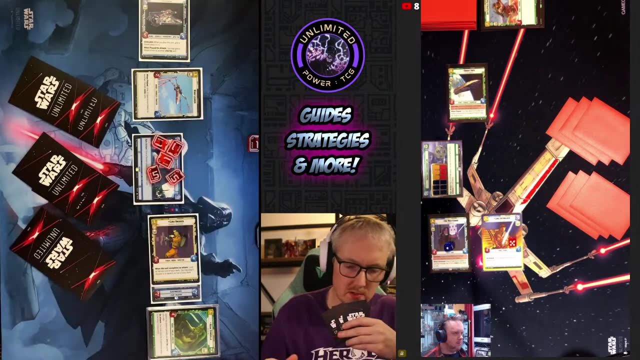 I cannot find a four. Do I have a five? Ah, there we go Some bad maths there. Nine up to thirteen, No worries, that makes more sense, Alright, What do you want to do now? Now I want to take the initiative. 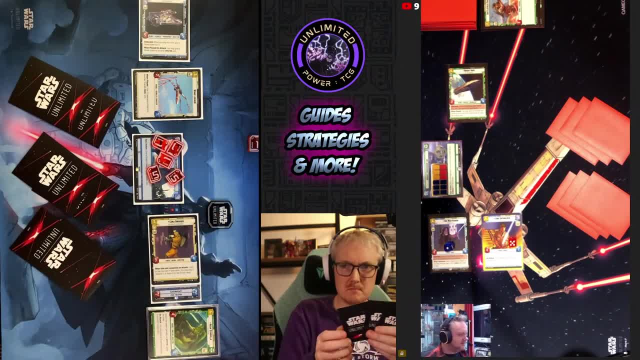 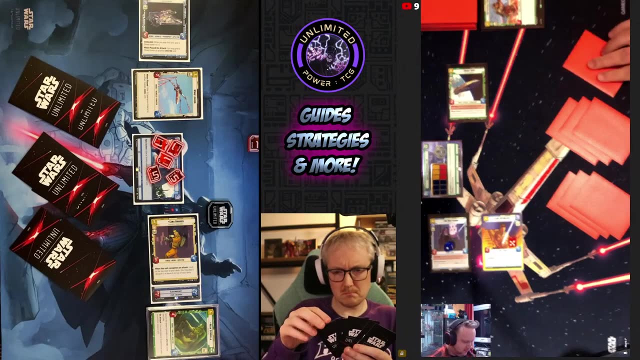 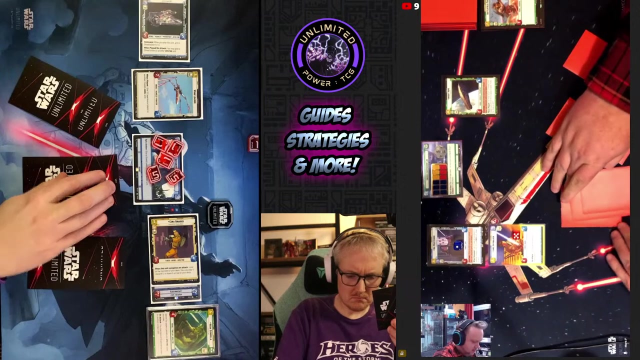 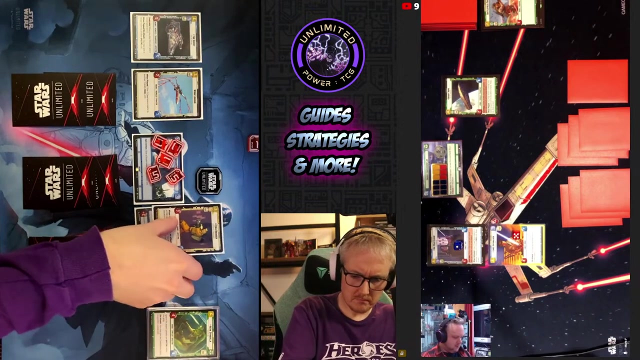 Okay, Interesting choice. Uh, I will pass. Okay, That's a nice card Oof. Well, yeah, that's resource you Not a lot of real thought involved in that. Okay, Off you go, sir. 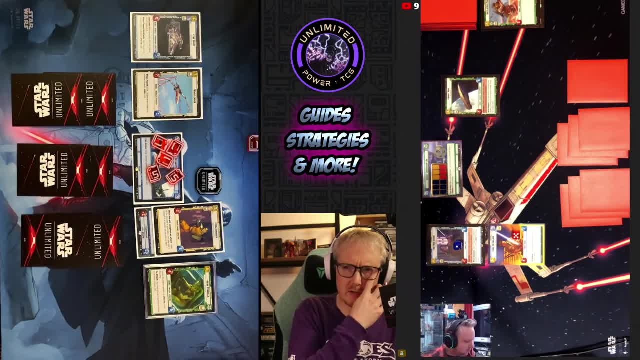 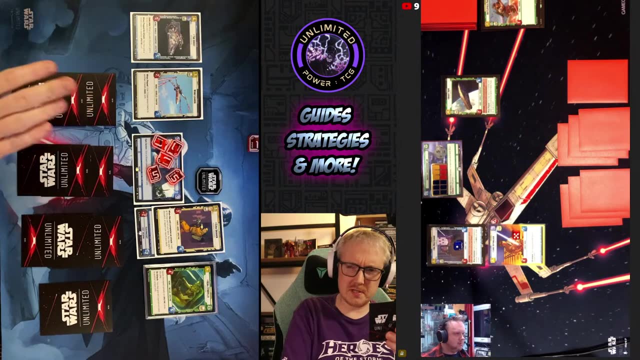 So your Luke has two hit points remaining. Is that right? That's correct. yes, So I will resource this card And I will. Does he count as an enemy unit? Yes, he is Okay, then I'll play all seven. 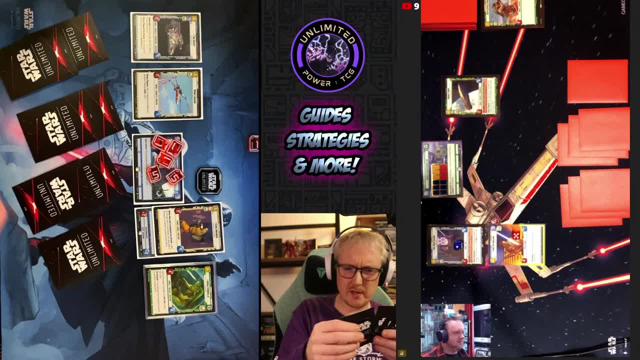 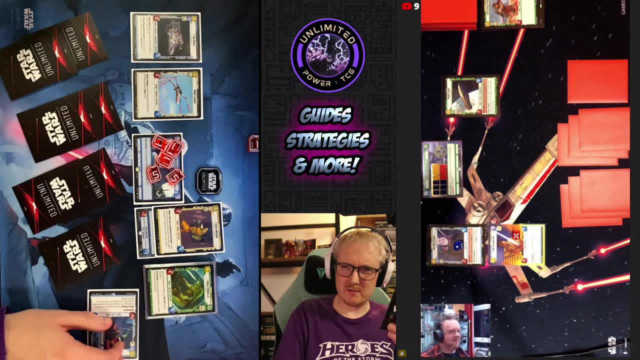 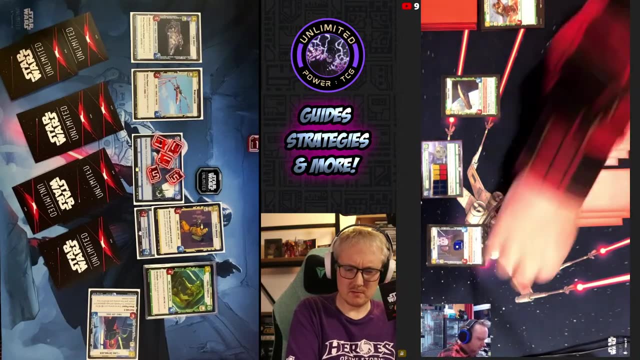 Okay, To bring in Luke Skywalker himself and give your Luke minus three, minus three, Alright, fair enough. Which kills him, right? Yes, that does indeed kill him, Okay, Alright, Very good. After he's dead, he goes. 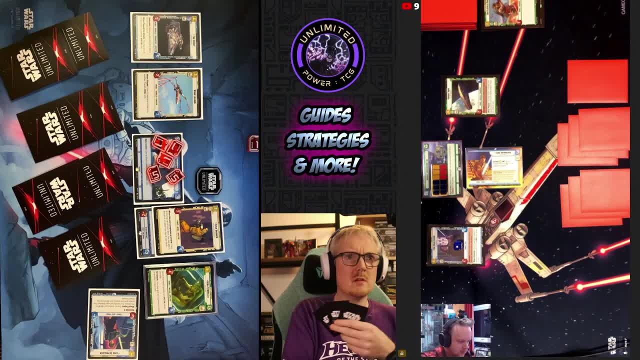 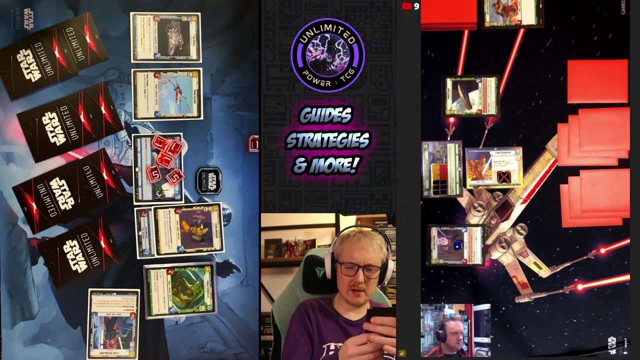 in exhausted And his epic action has been used. Okay, right, I'm not sure of the wisdom in that, Like maybe I should have hurt Obi-Wan, but No, it's fair. it's fair. Well, I will. 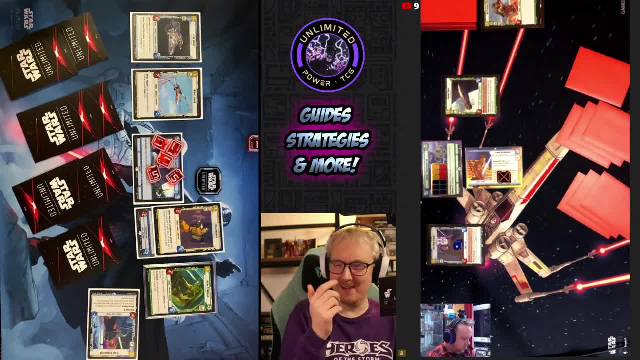 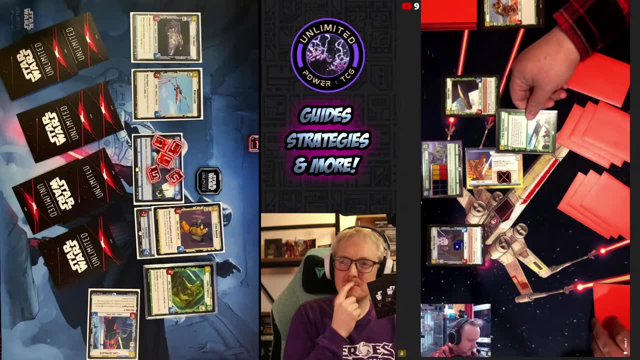 also pay seven And bring in your Luke. The card I'm playing is not Luke. The card I'm playing is something called Ewing Reinforcements. Oh, this is a cool card. So seven cost command heroism. Search the top ten cards of your deck. 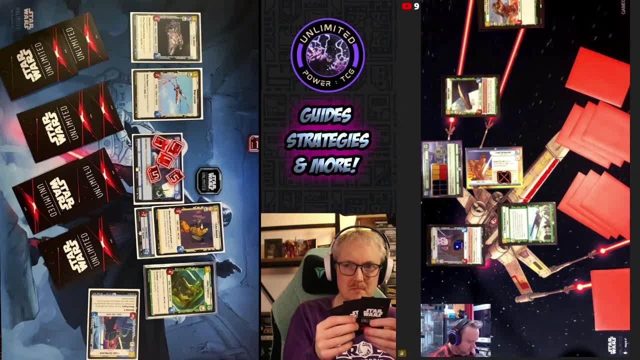 for up to three units, with a combined cost of seven, and put each of them into play for free. One, two, three, four, six, seven, eight, nine, ten. That's good. in my deck, I think, one copy of it. 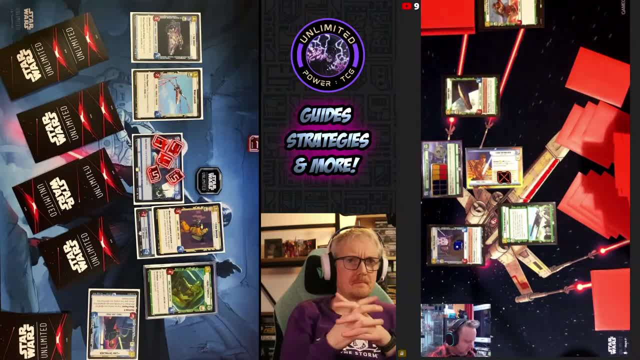 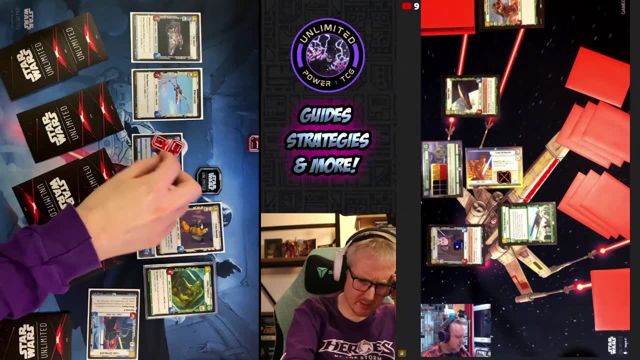 One, two, three, four, five, six, seven, eight, nine, ten. That's right. Good, What do we have? It has to be units. Yeah, it has to be units, It has to be units. so it can't be that. 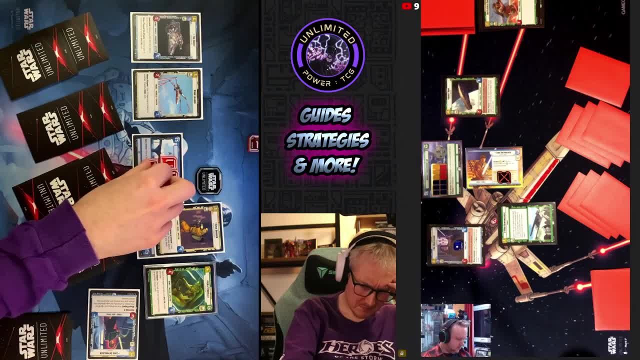 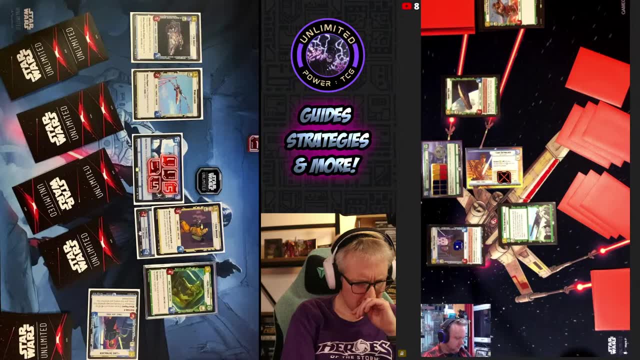 Can't be that. It can be those. It's not going to be that, Could be that, but it's going to be these and some combination of these. I've taken five damage to my base already. That would seem like a reasonable. 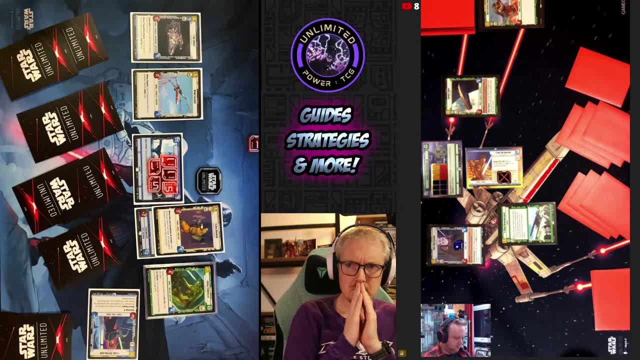 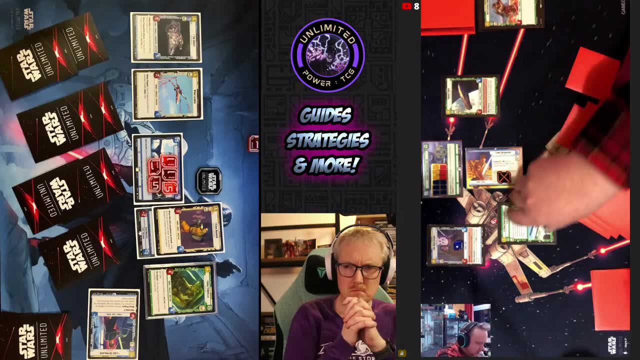 set of plays, I think. So let's put the other cards of the bottom three of your deck in a random order, so I'm going to shuffle the ones I don't play, which is fine. So your play A Colonel. 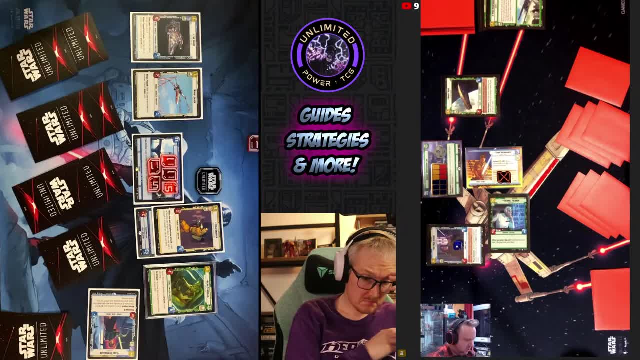 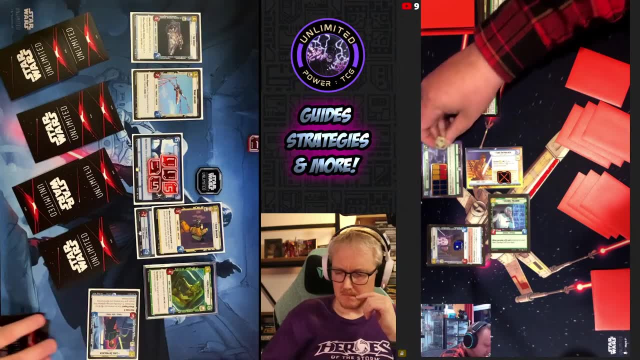 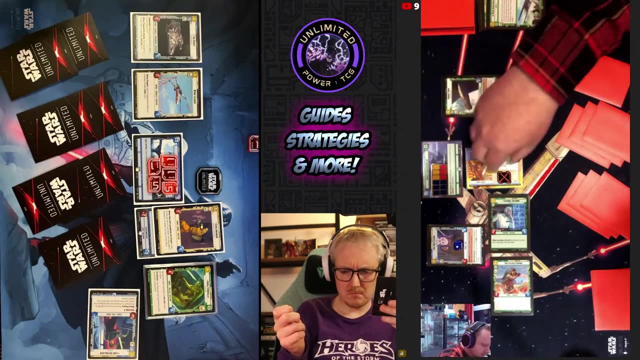 Yalarin, Which heals me for one down to four. Perfect, If I can find what the four is. There we go. I will play a Battlefield Marine, which is another green unit, so that will heal me for another one down to three. 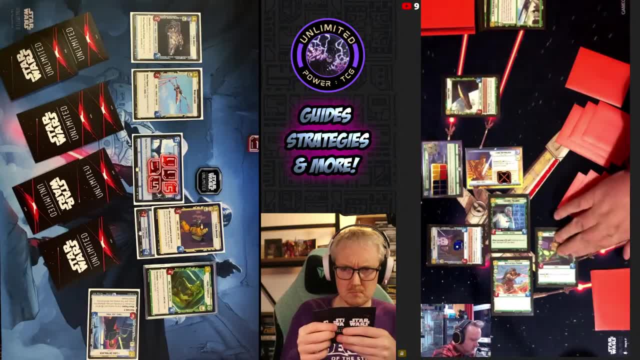 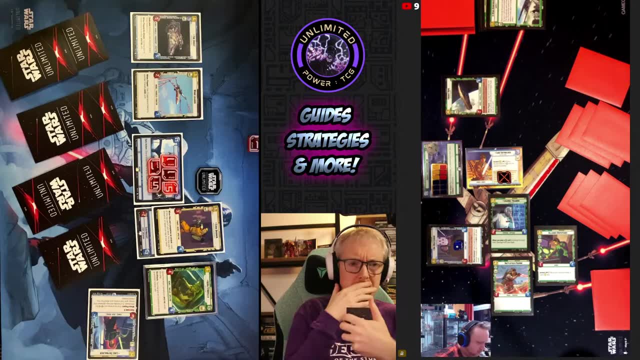 Yep, I will play an Alliance Dispatcher which I haven't seen yet. It's one cost one, two for an action. you get to play a unit from your hand and it costs one resource less, but it's another green unit, so that heals me for another one, Did I? 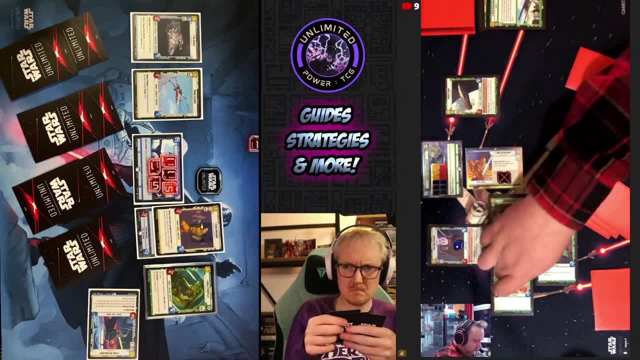 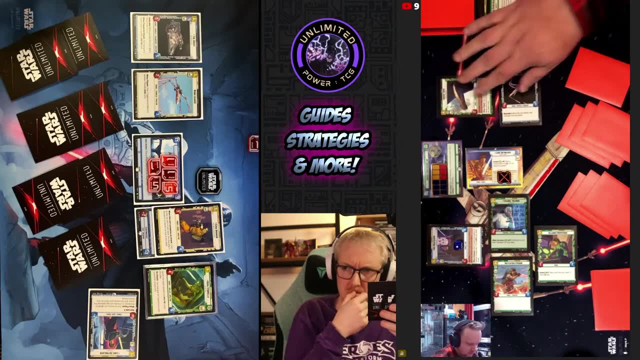 get two points of damage, That's two, four, five and for my final two resource points, I will play a Restored Arc 170, which is a 2-3 spaceship with restore one Perfect. The other cards that I have played. 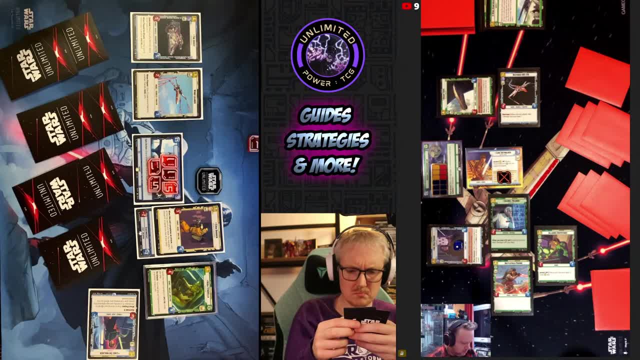 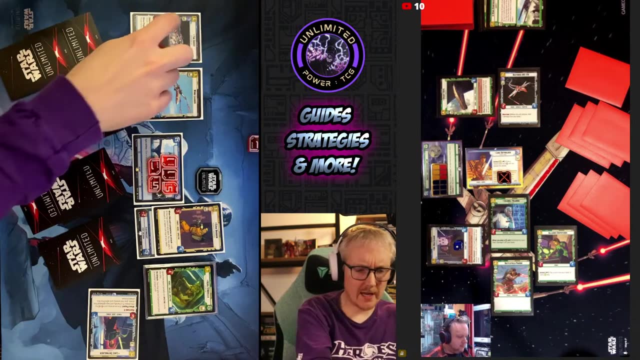 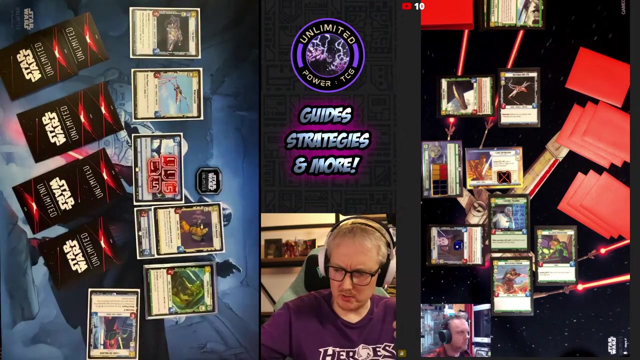 get shuffled And put to the bottom of my deck. And that's my action. Okay, I'm going to attack with a ghost. Okay, To hit your sentinel spaceship. for five Yep, I will take two damage on the ghost, Yep. 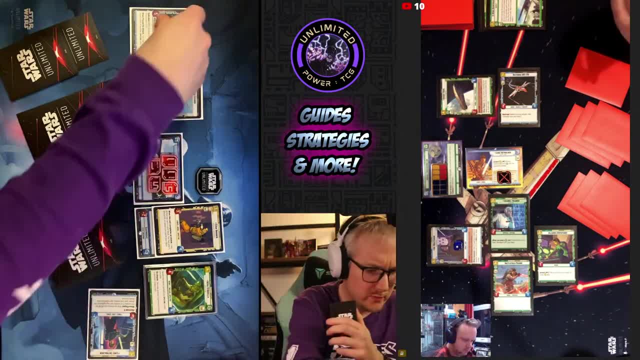 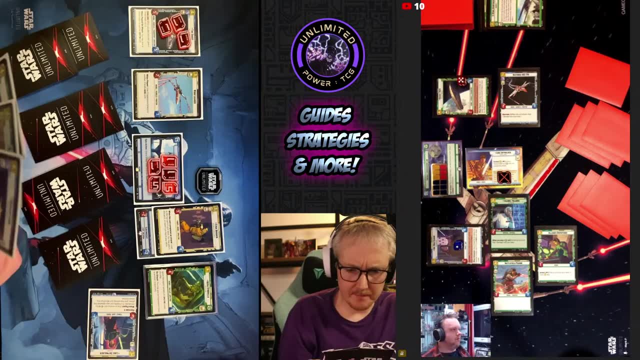 And this will go down to three Yep, But it will put you down to one Yep. Yep, I've got five taken. that's right. I can give a shield to another Spectre unit. I've never actually done this before, but I assume. 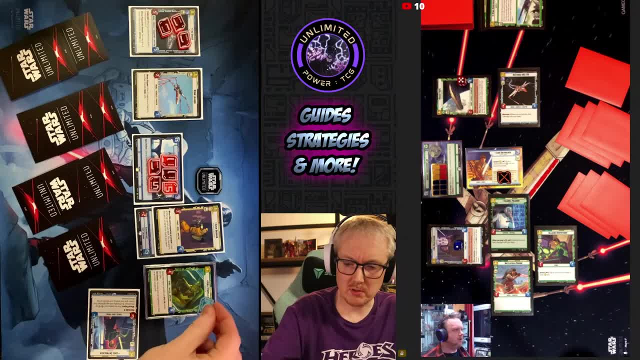 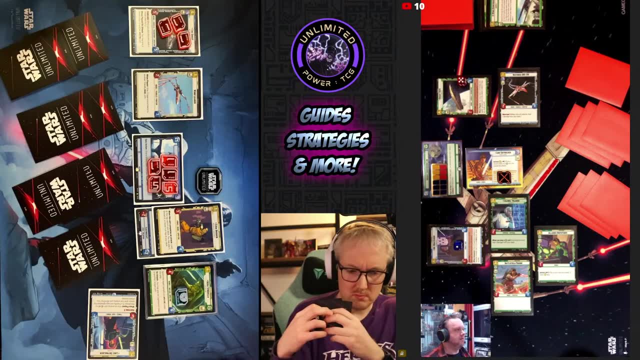 because my leader is Spectre. that's fine? Yeah, sure, Absolutely So I'll give her a shield token. Certainly, No worries. You do have to tap the ghost for doing that, though. Oh yeah, 100%, Should the ghost have been shielded? 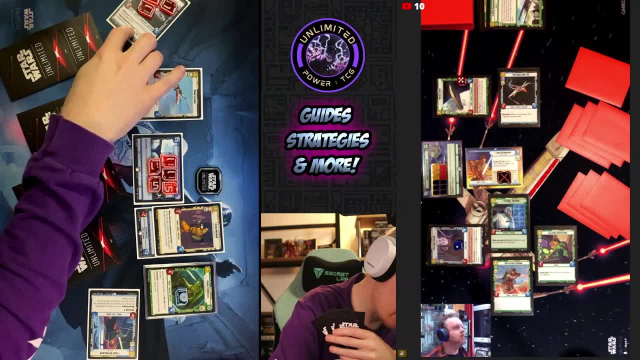 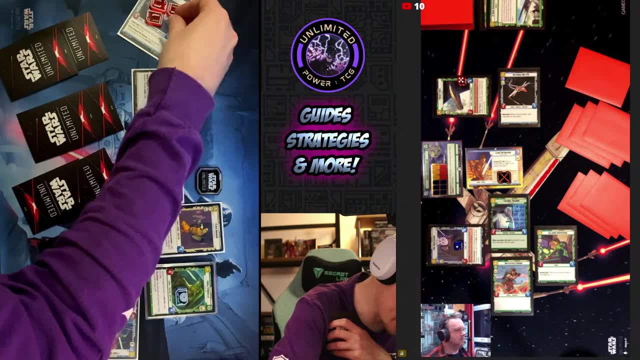 No, when you play it. Oh yeah, it gets a shield when it's played. Sorry, So it gets a shield, and it gives a shield every time you attack. Oh well, it's even better than I thought it was. 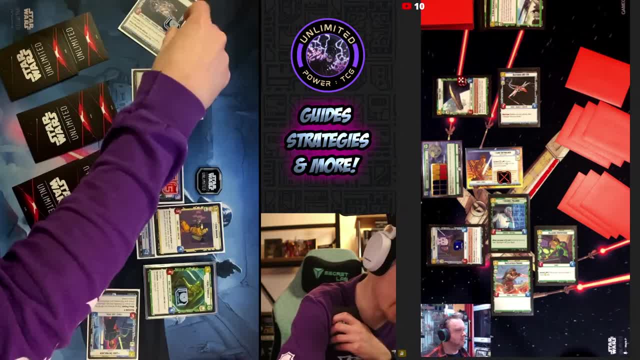 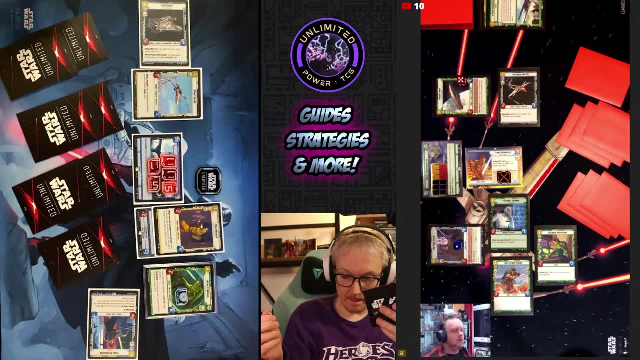 Sorry, I missed that. So it actually takes no damage from you this first attack. It just lost its shield. Yep, that makes sense. Thank you. Thank you, Keep me right. No worries, My pleasure. What else are we doing? We're doing that. we're doing that. 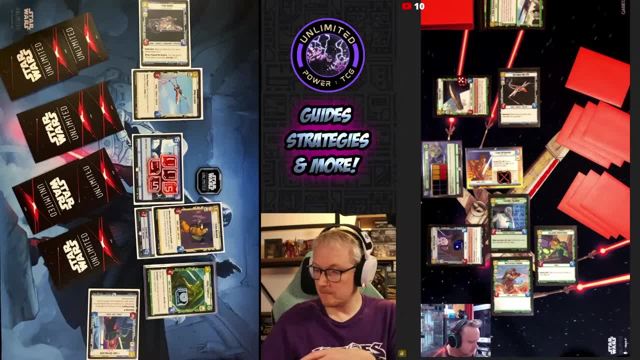 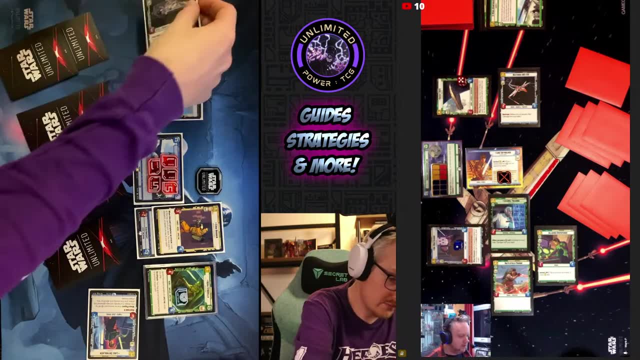 we're doing that, So I've got two things left to do stuff with. so I think I missed that when I played Tony, actually because I used the ghost against him as well. There you go, You learned. Yeah, you live and you learn. 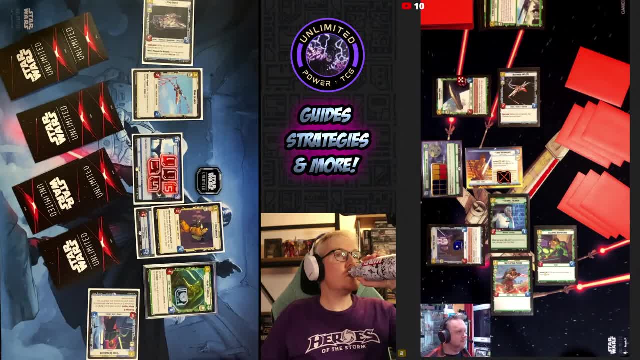 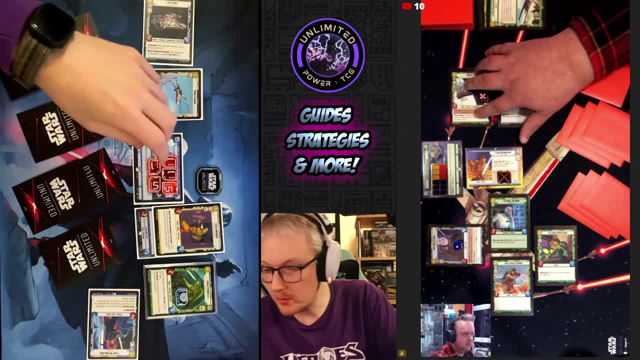 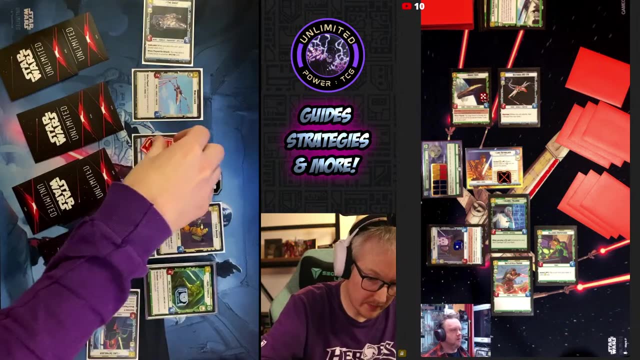 So your wing leader's going to kill my Bright Hope if it attacks it. so let's get the Bright Hope's damage in before it dies. So Bright Hope into your base for two, please. Sure. So 13,, that's 15,. so you've got. 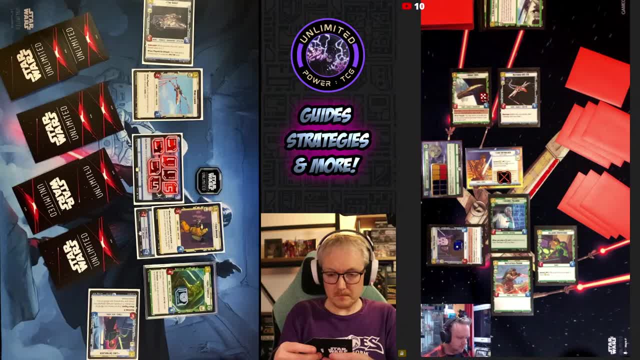 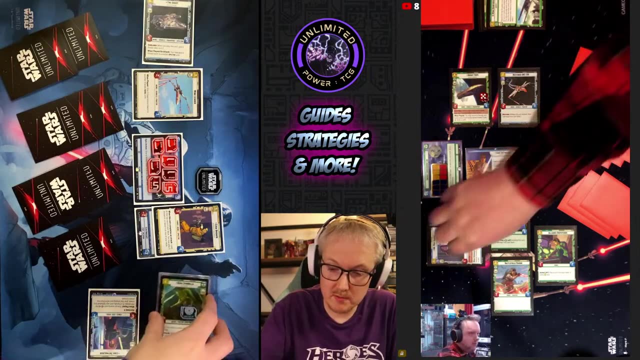 10 hit points. You have 10 left. yeah, No worries. Okay, Off you go. What's next? I think Hera attacks your bait. sorry, Hera attacks Obi-Wan Kenobi for four. Okay, Loses her shield. Stings off shields. 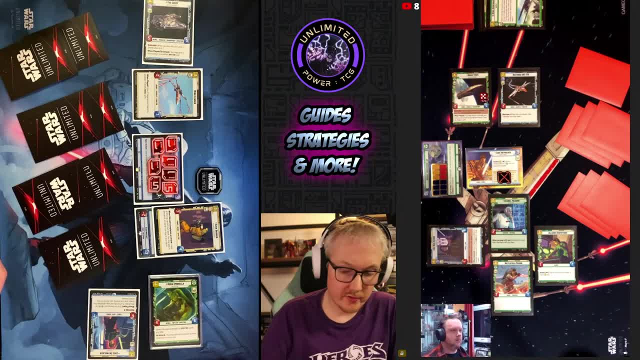 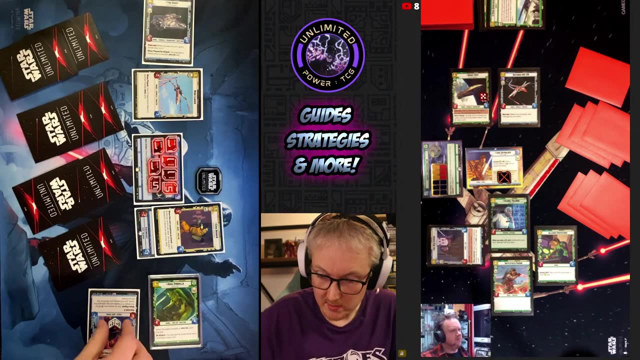 Yep. But in doing a good attack she gives a plus one plus one to. Let's give her a plus one plus one to Luke. Luke becomes a. Who do you say you can give the experience to? On attack you may give him. 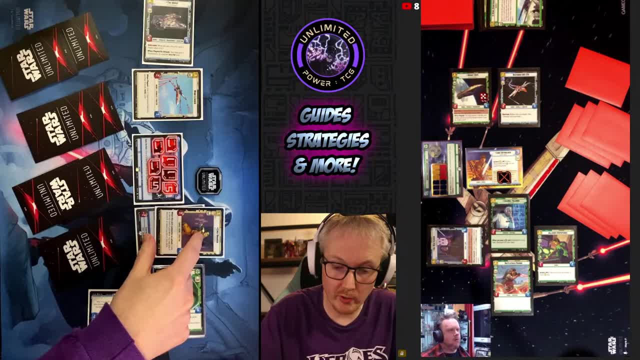 experience token to another unique unit. What does it mean by unique One that I've only got one of in play? Uh, a name. So you see there's a little star beside the name as a Bridger. Here is Syndulla and Luke Skywalker. 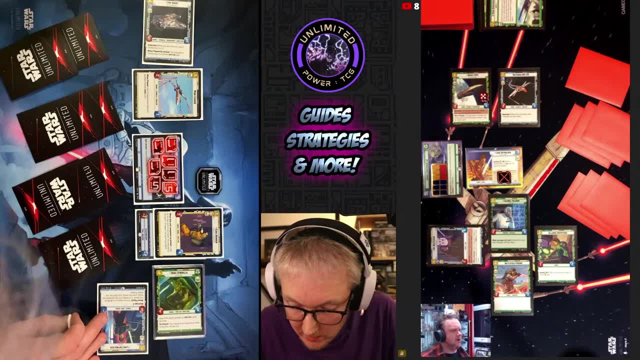 Yes, That means they're unique units. The ghost is a unique unit as well. Wing leader is not. I'm going to give it to Luke because he's got restore three and I feel like I'm going to need to be healing my base. 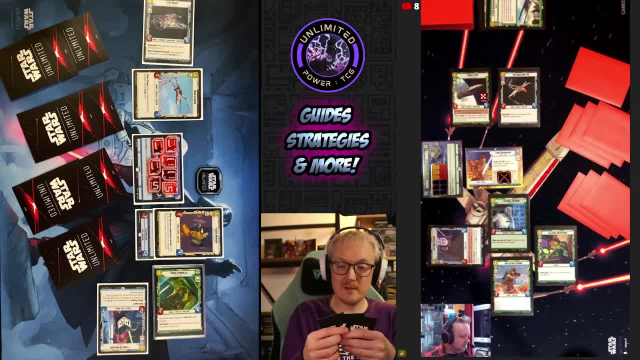 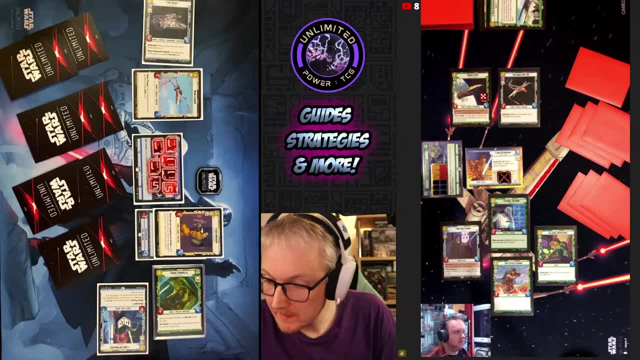 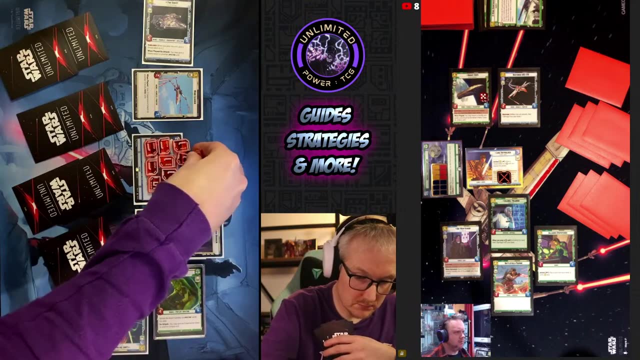 pretty soon. Fair enough, That makes sense. On that, let's hit your base for four with Obi-Wan, Sure. So that's 19 taken. I think No, it's a lot. It is a lot, Let's. Do you want to replace? 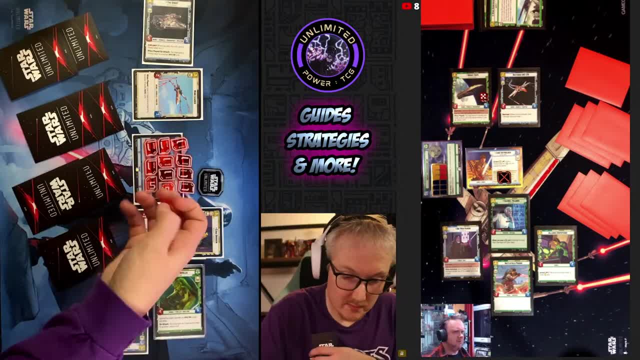 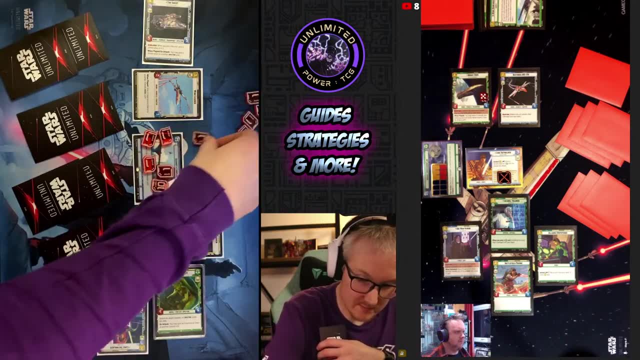 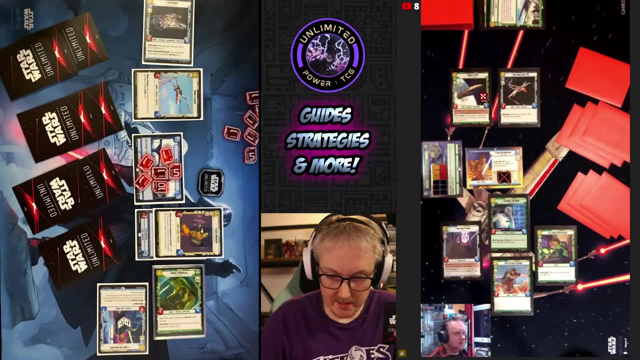 some of those with tens or fives. If I had one, yeah, There you go, 19.. So you want a ten and a five and four ones. Nice, Cool, Let's. um, I feel like I can't leave Obi-Wan alive again. 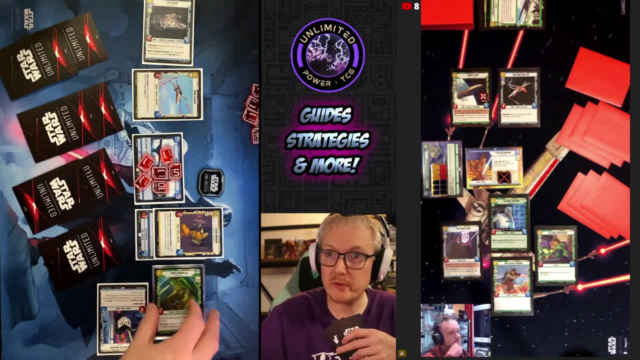 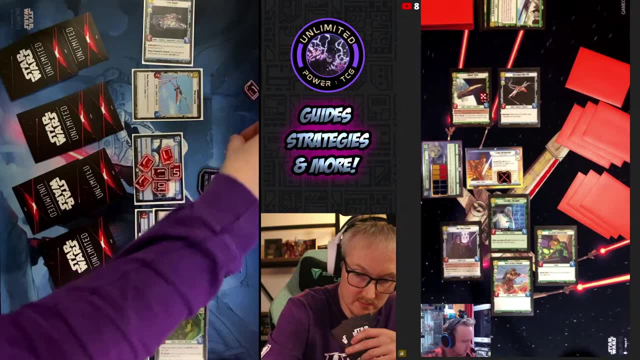 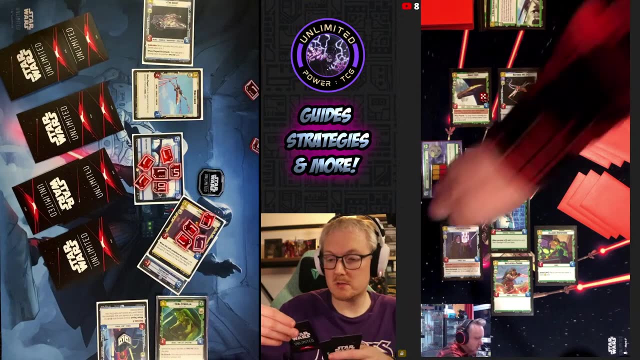 for another turn. so let's kill them with Ezra, and Ezra will take his four Yep, Alright. In doing so, I can look at the top card of my deck Yep, And I'm actually going to bury that card in. 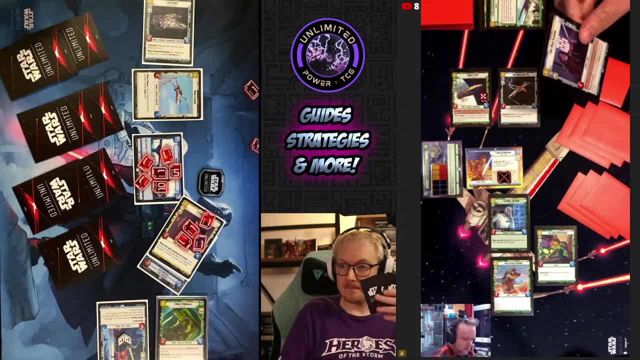 my discard pile, because that's not going to help me much. Obi-Wan dies. I give two experience tokens to another friendly unit. It will be the battlefield marine. It's not a force unit, so I don't get to draw a card. 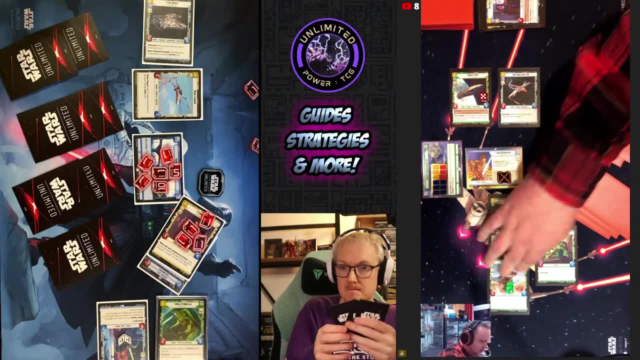 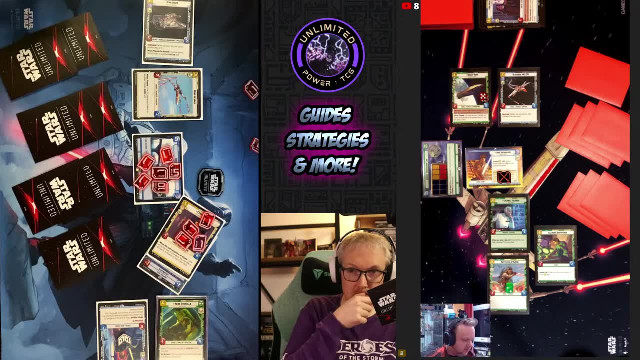 but I do get two experience points on that guy Mm-hmm, Which is great. Alright, Probably actually wins you the game. I think I will take the initiative, because all I need to do is six damage to you and I reckon I can. 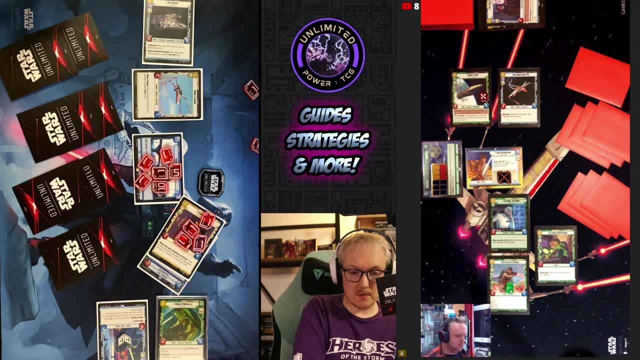 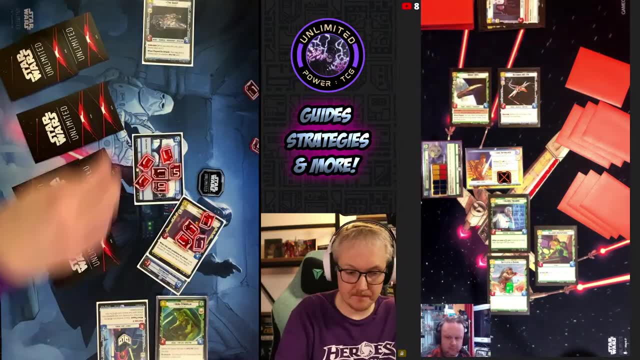 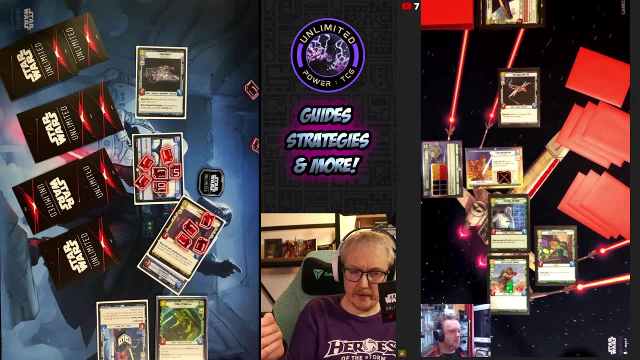 probably do that next turn before you can stop me. Okay, so I will attack your spaceship, Yep, Which will kill yours and kill mine, With my wing leader, Yep, And that would be me done. So draw two, Alright, No worries. 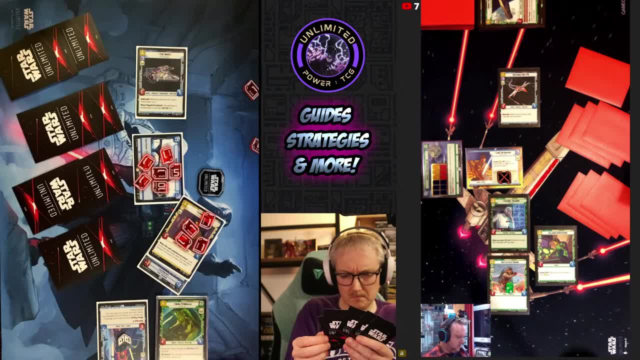 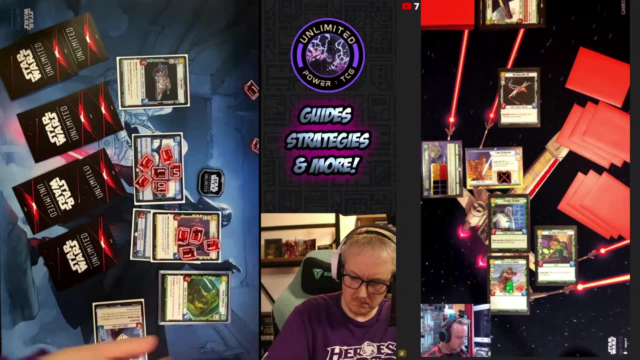 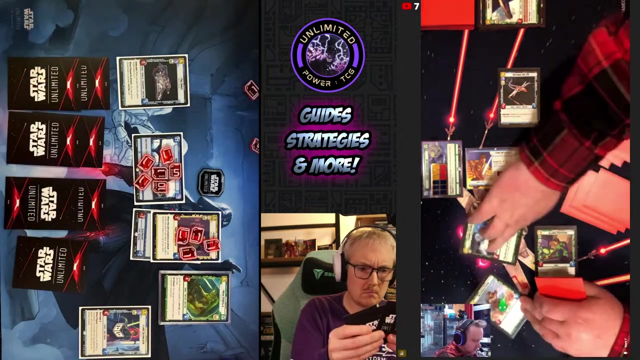 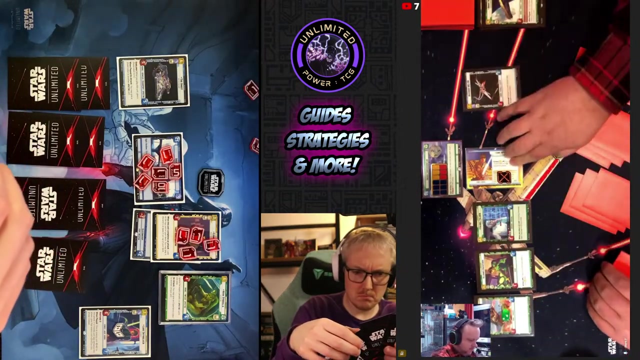 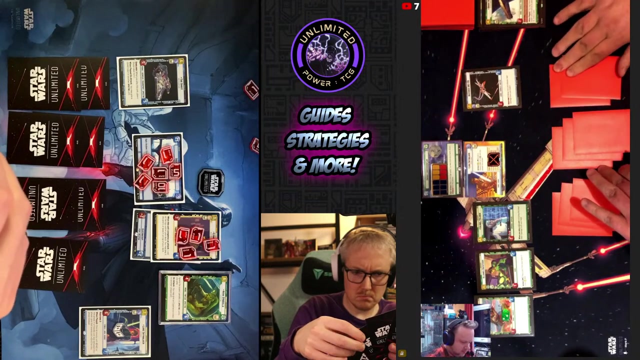 Here we go. Which way around do I want to do this? I think I'm going to have to be playing that, Which means Let's resource you And ready up. Okay, I have the initiative, so let's get the obvious. 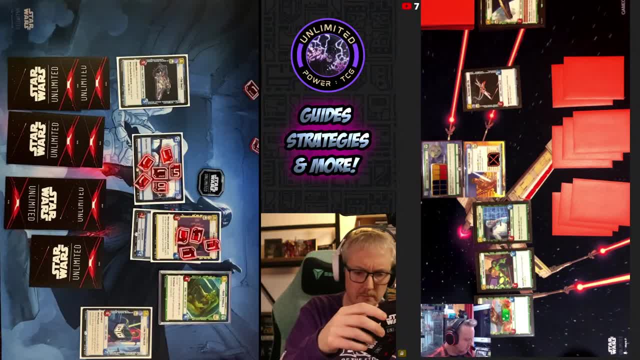 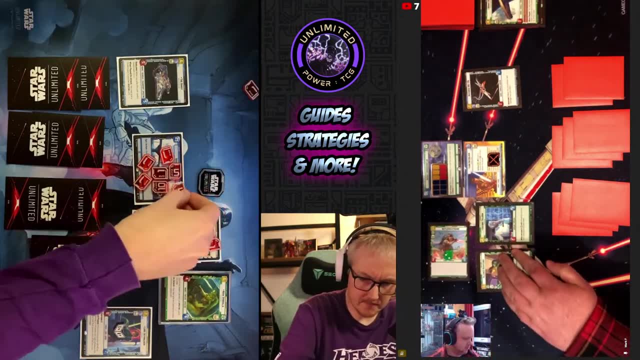 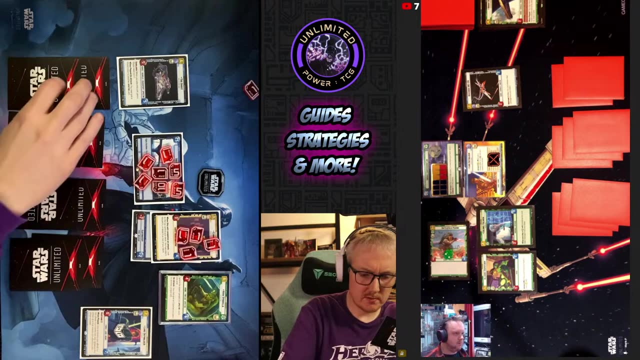 out the way. Mm-hmm, If you're ready? Yep, I'm ready. Alright, so battlefield, marine Five to your base. So that leaves me on one crit. Yep, Okay, I will play This as a resource, Mm-hmm. 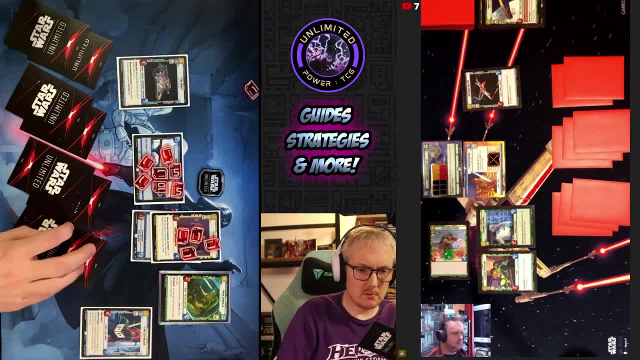 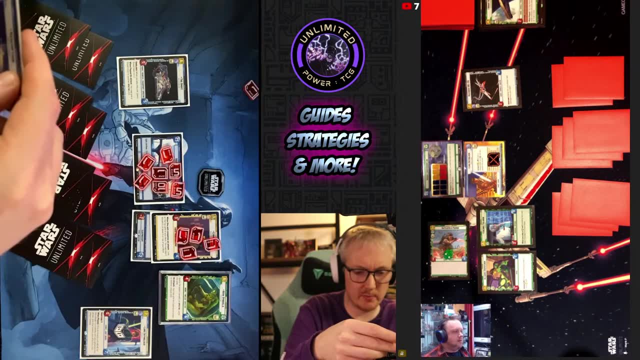 Then I'm going to do eight Yep To play a redemption Yep. It's a six-nine spaceship When played heals, a total of eight. damage from any number of units and or bases Deal that much damage to this unit. It doesn't have to be eight, It can be anything. 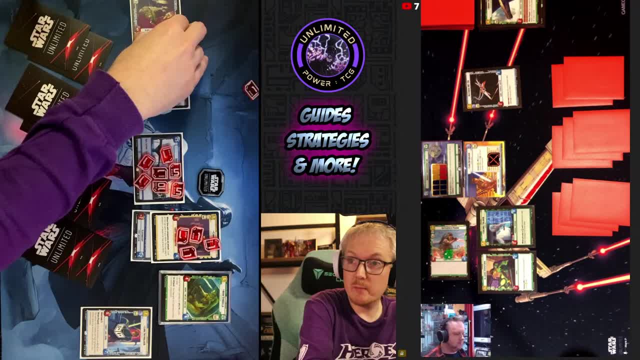 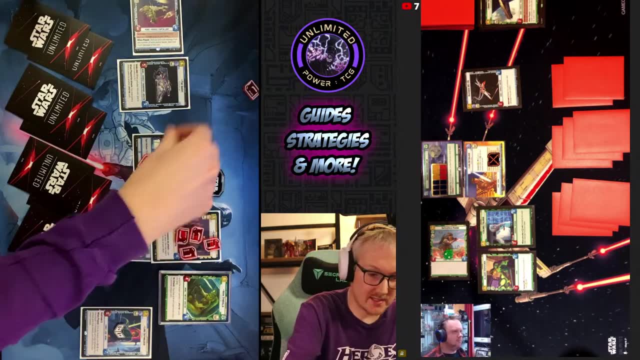 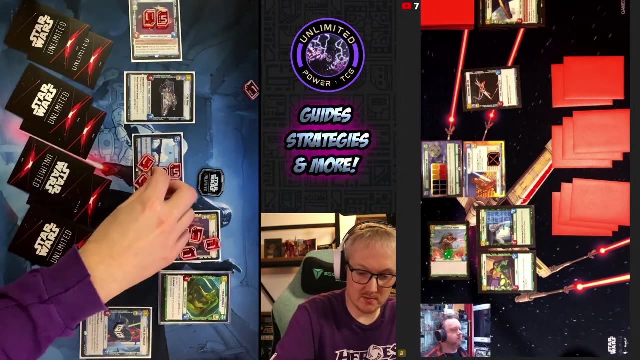 between zero to eight. So I am going to heal my base for six, Okay, And take the six damage over onto the redemption, Alright. So my base is Three health left, Which is one more health than your arc fighter will do. 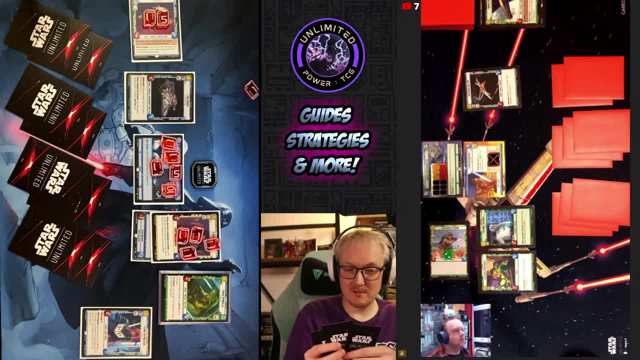 Yes, That's the plan here. So that's sixteen, seventeen, eighteen, So seven damage I need to deal Right. Well, that's mildly annoying, I must confess. Yeah, there's a good card to have at that point. 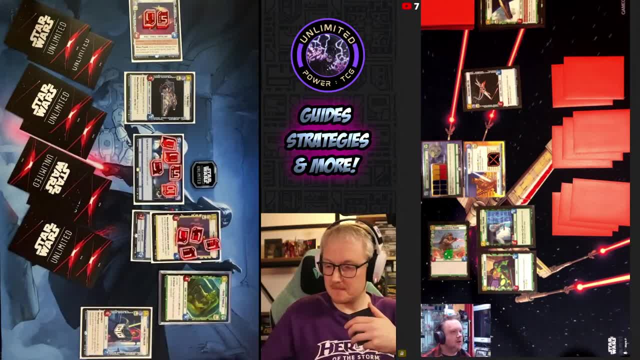 Hmm, It changes things up a little bit. Question is: is it going to make all the difference? I was concerned to take all eight damage on the base. to be honest, Yeah, Sorry, moving all eight over because I am low on life, So maybe this is a. 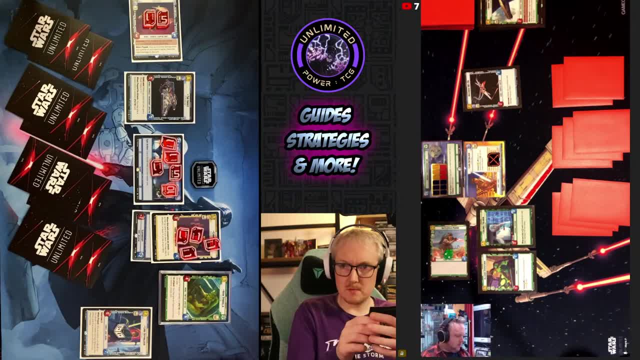 backfire, but we'll see. That means I'm not killing you this turn, This round at least One way or the other, And you can do a lot of damage to me This turn. So I need to be very careful in what I'm doing here. 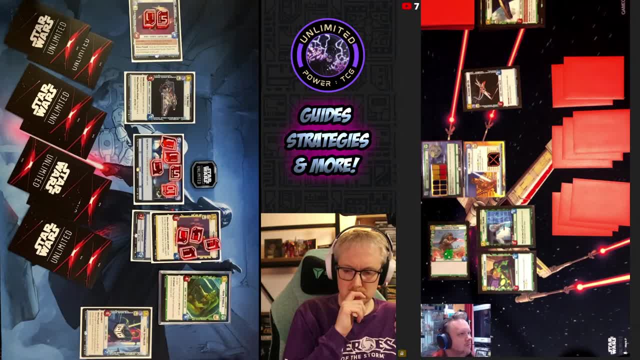 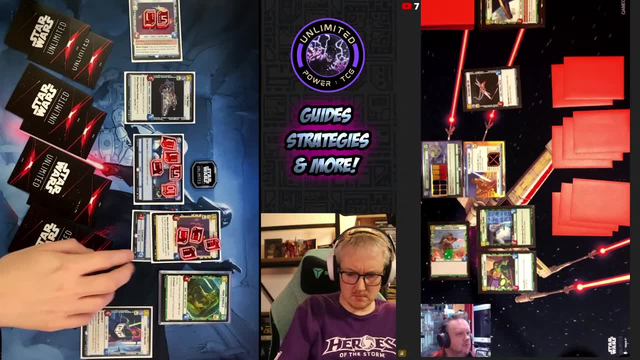 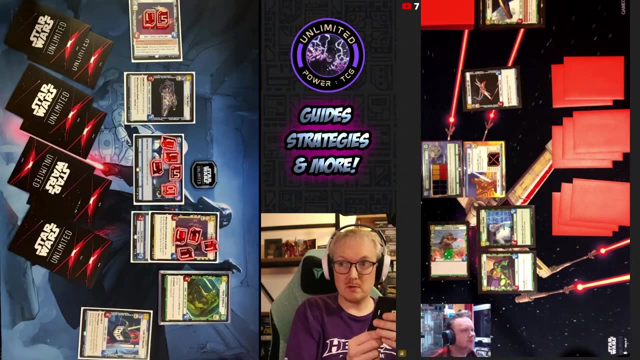 Right, What can you do with all that damage to me? Six health, Two health on Ezra, Seven, One on Luke. I could do seven, eleven, sixteen, twenty-one. actually, Ezra's doing five, Is that right? Yep, Ezra's doing five, Hera's doing. 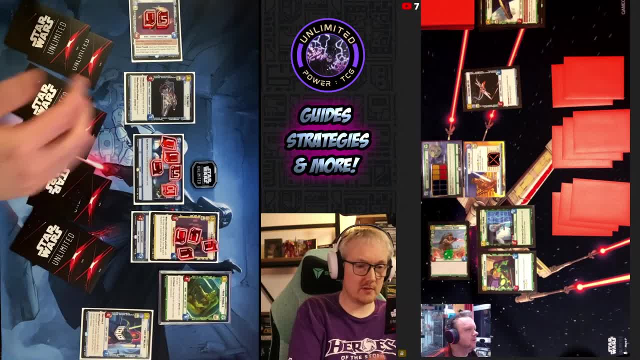 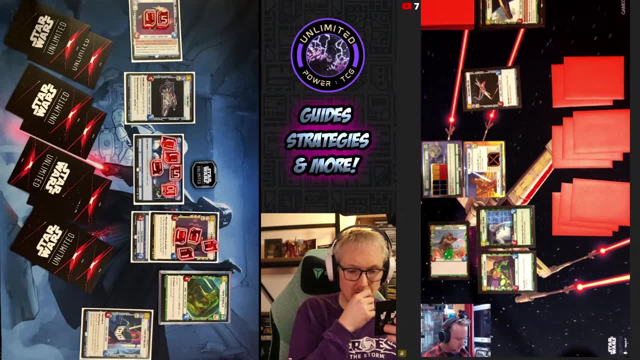 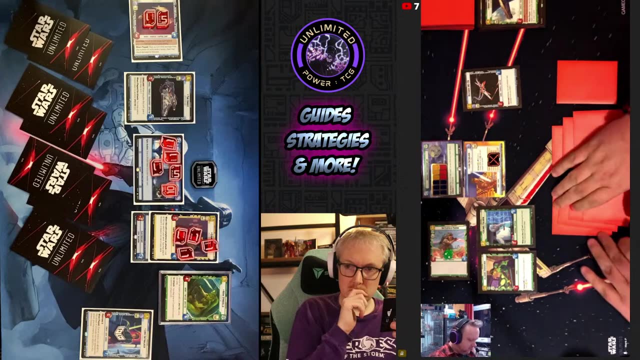 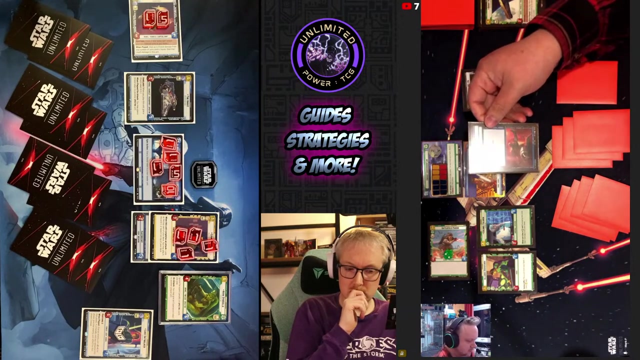 four. Luke's doing seven, The ghost is doing five, Right, Okay, Let's change this up And change my plans. We are going to pay four Uh-huh To play a takedown and kill the ghost with defeating a unit with five or less. 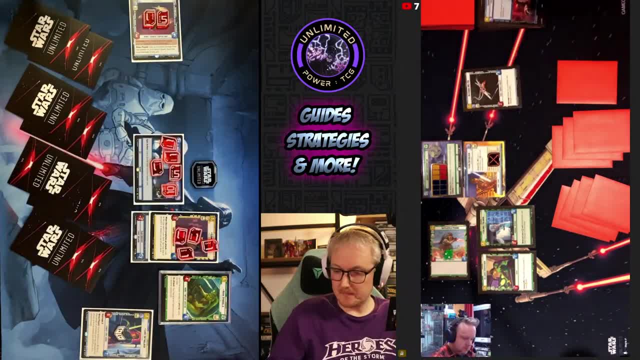 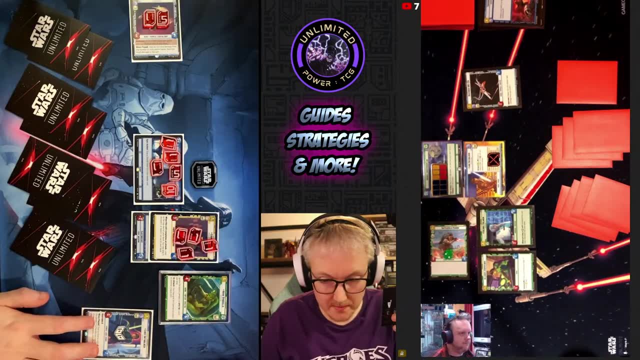 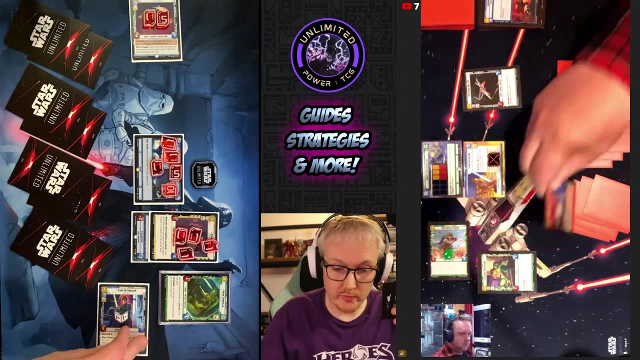 remaining hit points. Very nice, Okay, It scuppers me a little bit. I'm going to then use Luke to kill your Artlaren. Okay, And Luke is going to restore three to my base. Fair enough, Luke takes two. 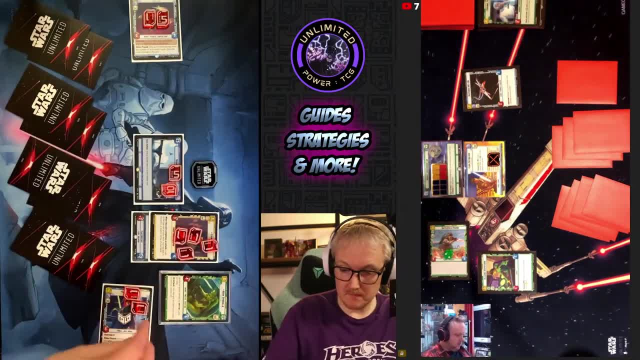 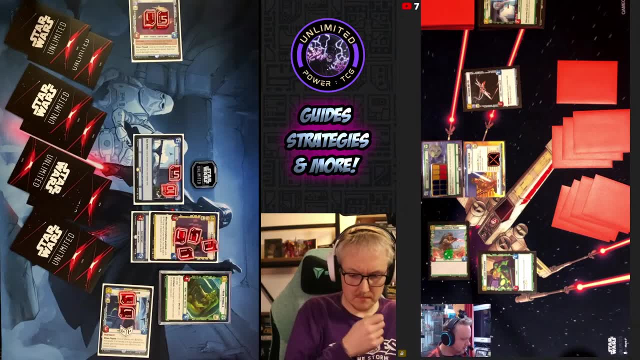 I should have thought about this a little bit better with what I resourced, because I could have done that slightly differently. That's aggravating. Still, that's the way it goes. Um, Hmm, Yeah, I've messed this one up. 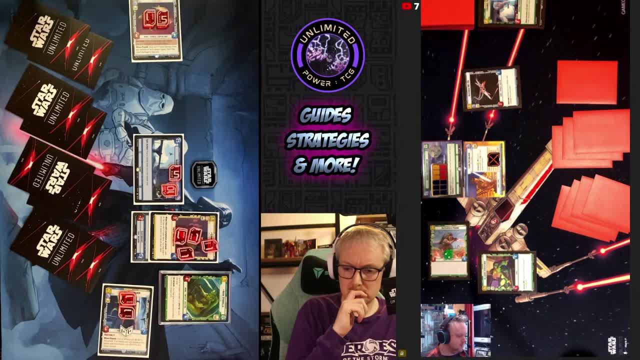 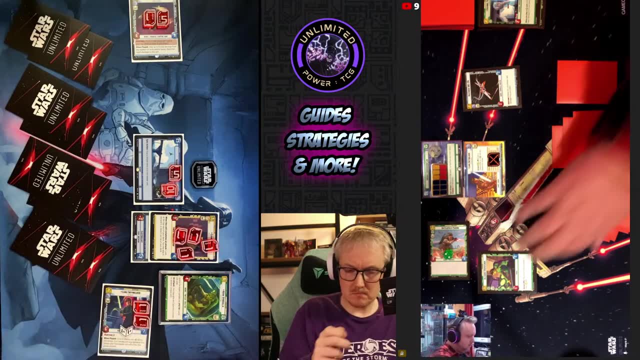 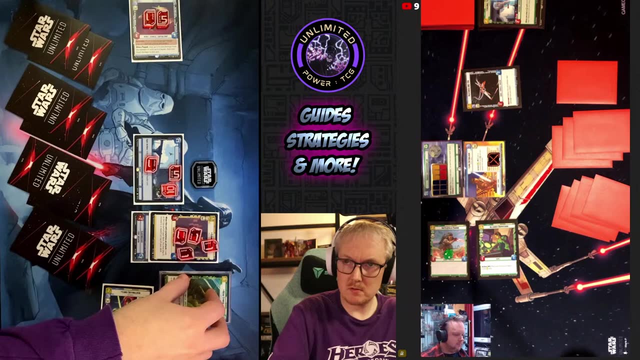 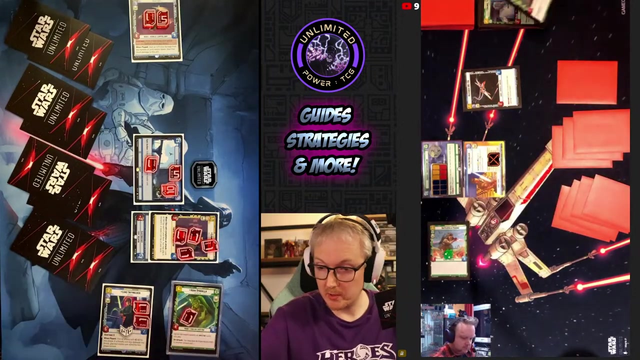 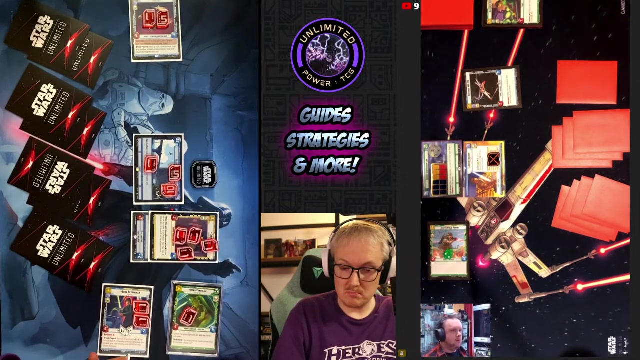 Okay, So I'm going to use Hara to kill the dispatcher. Alright, Let's do one to base with the Alliance Dispatcher. Okay, I'm going to use Hara to kill the dispatcher. Okay, And take one damage, And take one damage. 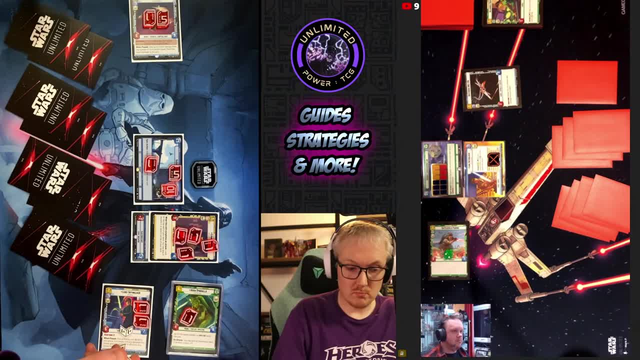 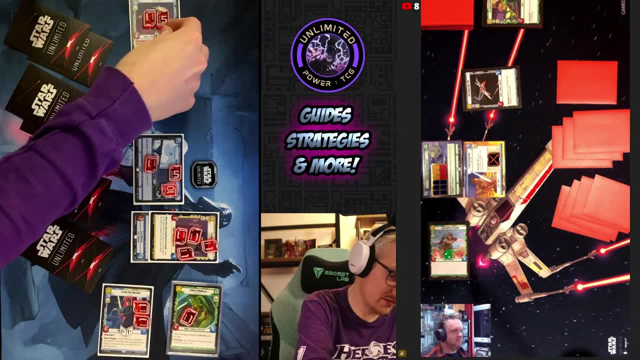 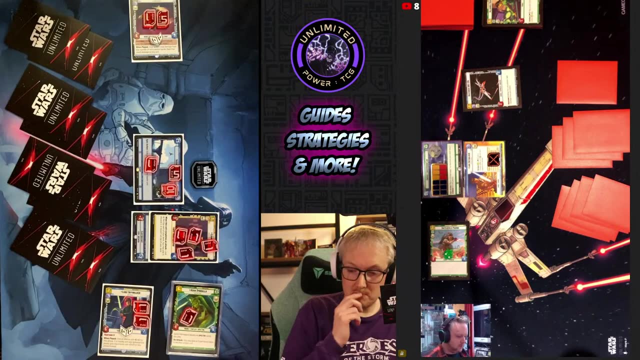 And I'm going to use her to kill the dispatcher. Everybody's holding their breath. My big flying ship. Okay, That's Sentinel. And then you're shot. It is, Um, Hmm, Oh, sorry. Sorry, I got that. 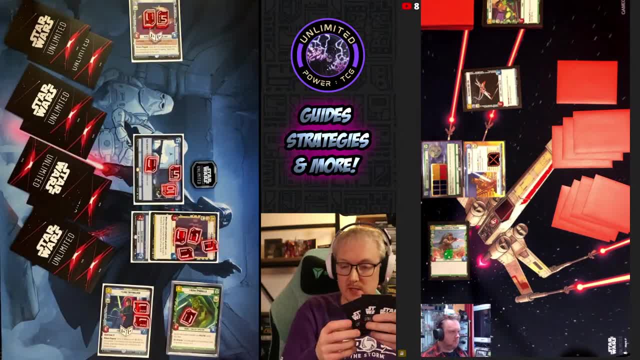 No, that's right. Yeah, that's right. Sorry, it's the ghost that gives the shield when you attack. Sorry, Yes, Yeah, Another reason why I killed the ghost. Um, Oh, this is annoying. Oh, I'm going to. 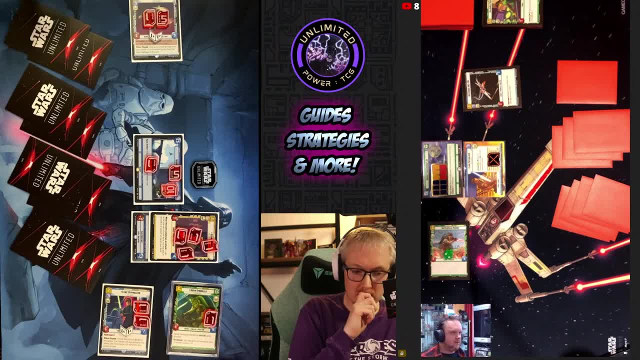 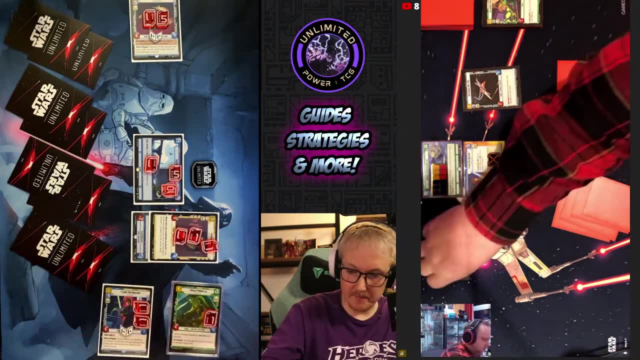 take the initiative. You are, I am Okay, then I'm going to use Ezra to kill your battlefield marine. He's going to die for that. Alright, straight trade. I do still get to look at the top card of my deck. 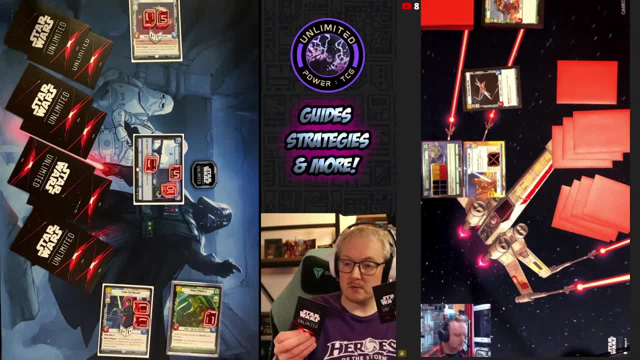 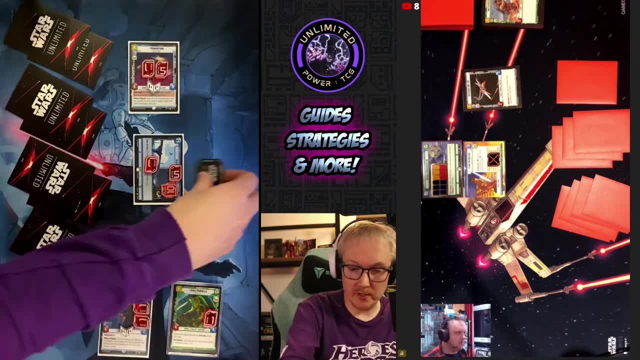 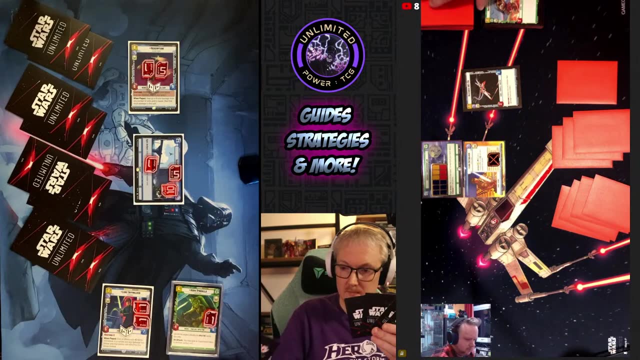 Of course, And I'll put it back there. I'll put it back there, Alright. Okay, so you've got initiative. I have taken initiative. yep, I assume you probably pass at this point. Yeah, two cards. 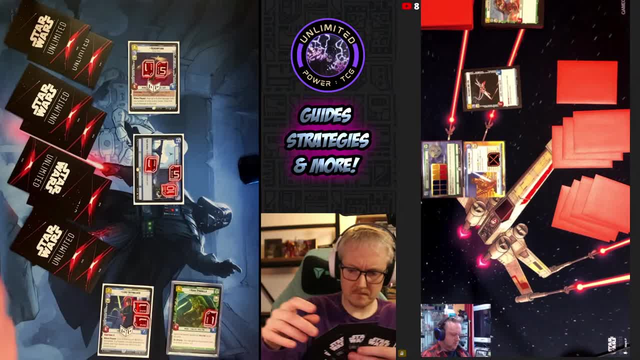 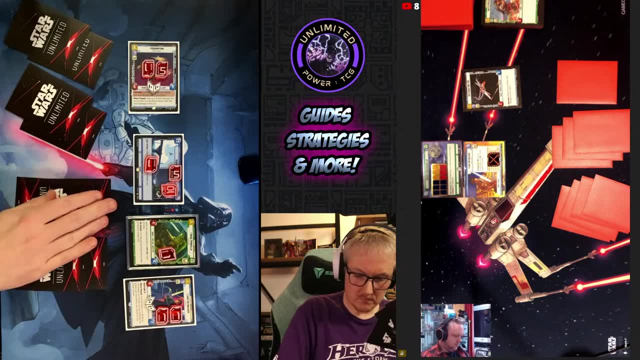 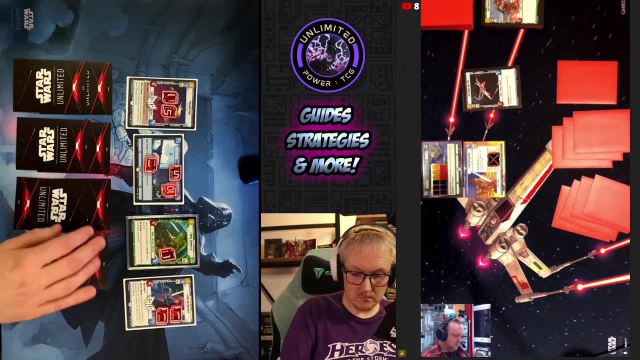 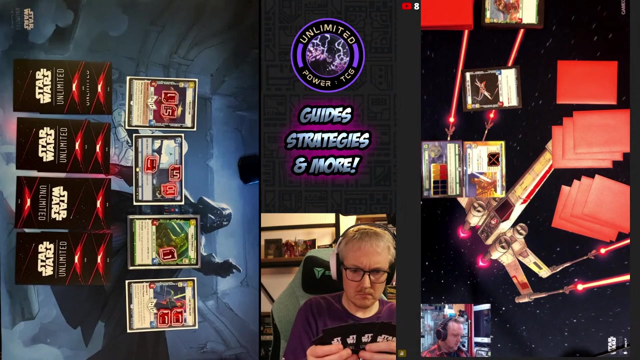 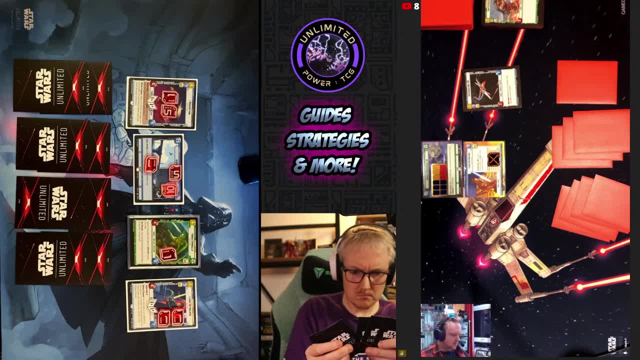 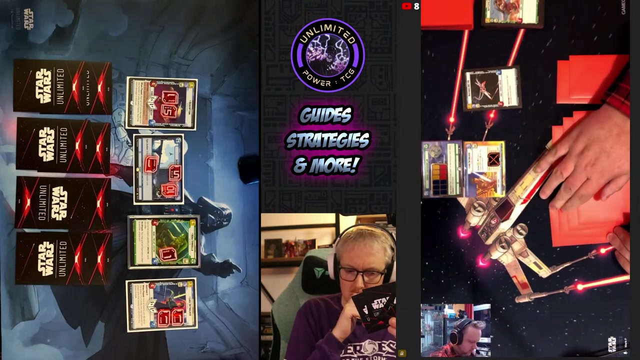 Um, That's a lot of damage coming my way, Hmm, Hmm, Hmm, I'm gonna have to prevent it, I think. So Let's play this down. Let's ready up Everything that I've exhausted, which is not a lot. 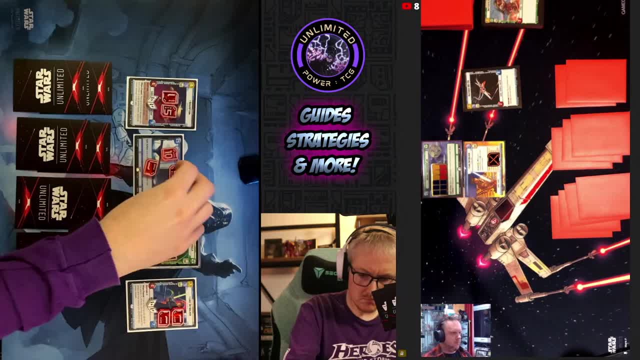 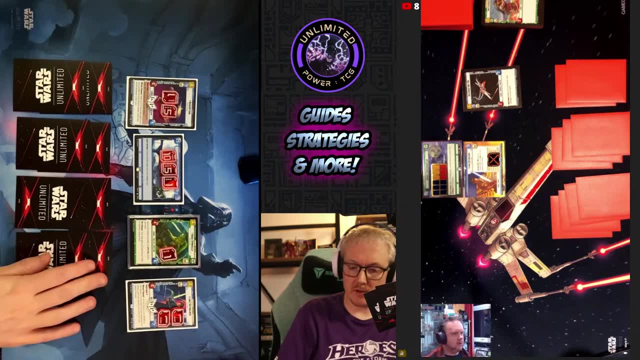 Which is not a lot, And I'm ready WHEN YOU are. Uh Well, you took initiative, so Have you played a resource? Yes, May type, I've played a resource, sorry, So you're on nine Eight. 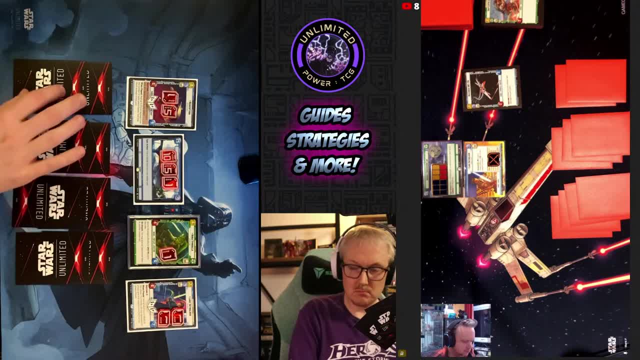 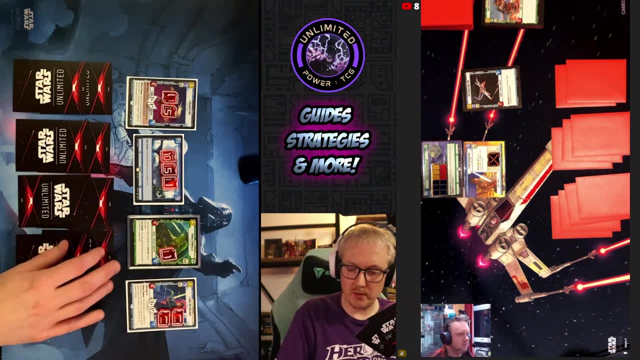 Eight. Did I miss a turn? I'm on nine. Oh, maybe I'm waiting. Do I not play the resource when it's my turn? No, you play it now, before the turn starts. All right, my bad, I'll play my turn. 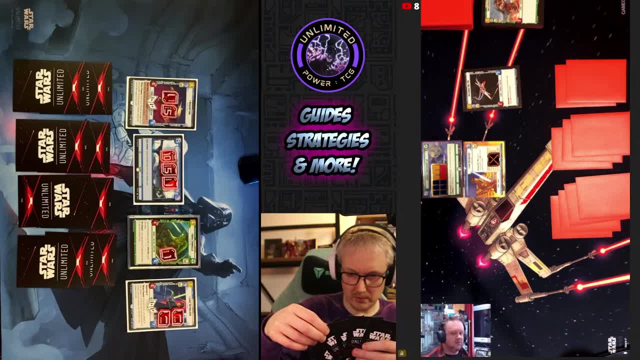 I noticed you did that last turn, which is why I'm prompting at you now. I want to go up to nine, Two, four, eight, Yeah, okay, Sure, Yeah. this might be the last time I'm playing a resource on this deck. 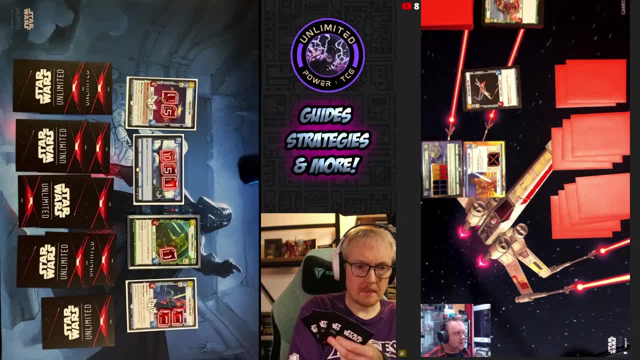 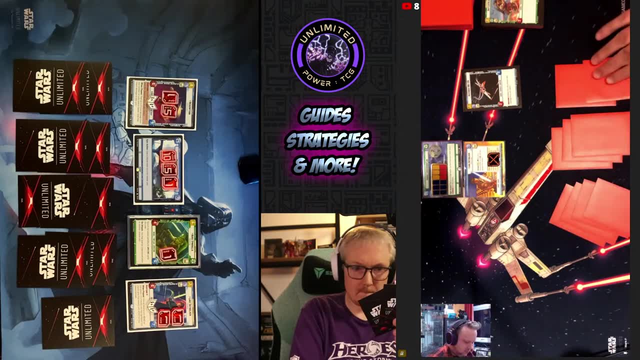 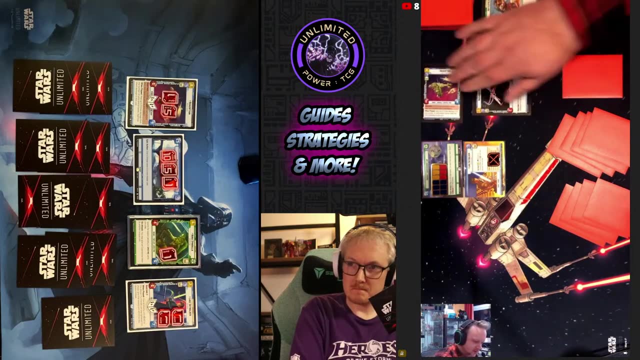 Yeah, okay, cool, All right. Okay, I have the initiative, I will pay eight. Oh, here comes someone, big Of your finest resources, to play a spaceship you might be familiar with. It's called the Redemption. It's Sentinel. 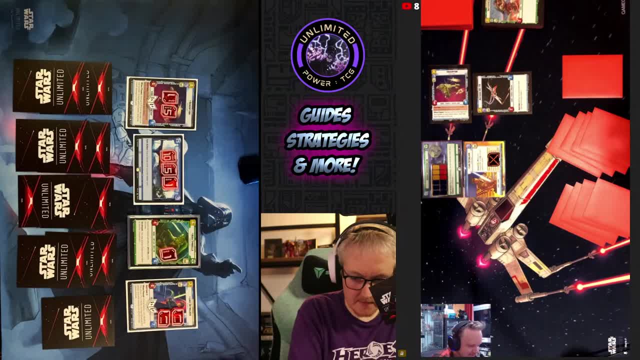 Same as yours, mate. Yeah, With a bunch of healers, I'm going to heal two, because I've only taken two damage. Okay, you're going to move the two onto the spaceship, are you? I am, which leaves the spaceship with seven health remaining. 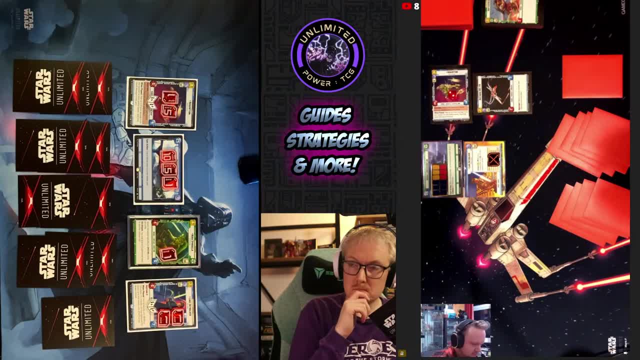 Oh no, you've got the thing, haven't you? No, let's not do that. I'll leave one health there and take one onto the spaceship, so it's got eight health remaining. That makes more sense. Yeah, because I would have just installed. 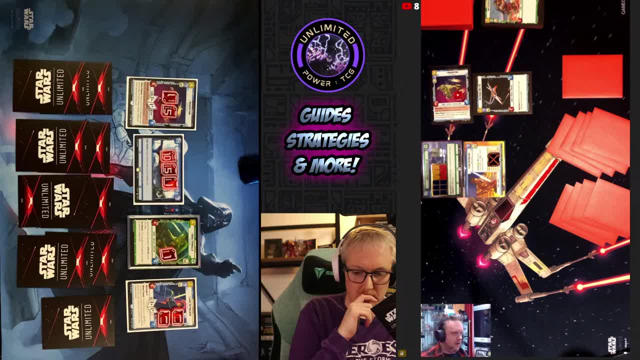 I recently killed it, Although you can give it an experience token with Hera anyway. Fine, we're not going to heal any. Leave my base on two damage. Okay, So your arc is doing two Yep And it restores one, And I have ten on this guy minus six. so if I kill you, I still have two health. 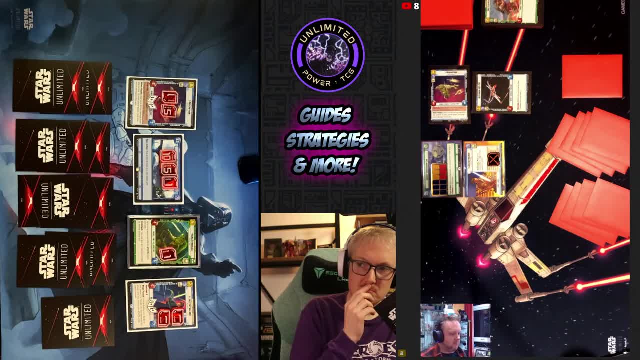 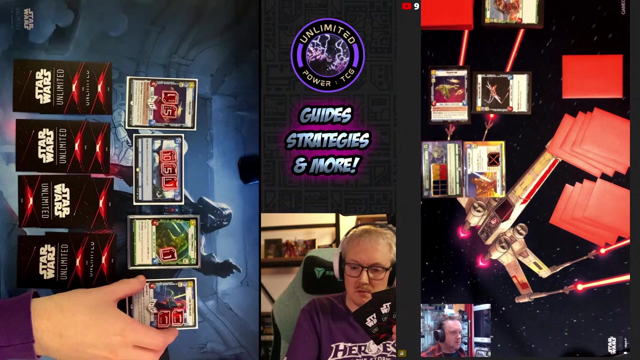 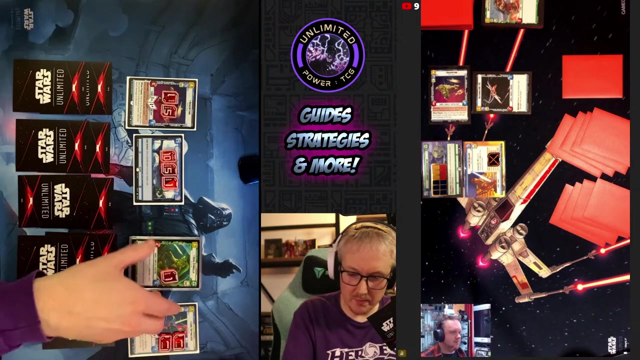 Oh, but I can't attack you, That's right. You can only attack the redemption, because it's sentinel. Okay, So Let's, Let's Swing. This is tricky, Let's swing. You're base with Hera for four. 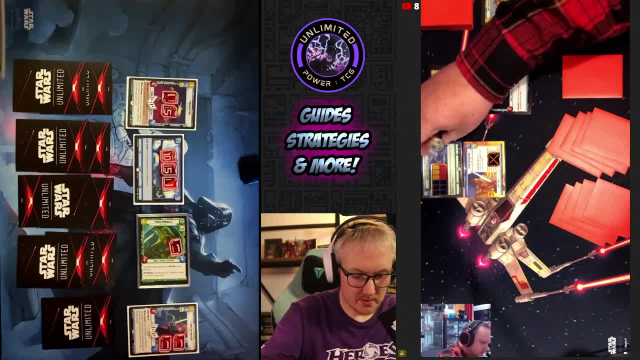 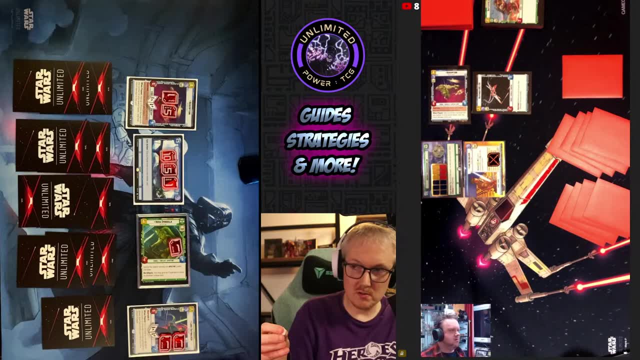 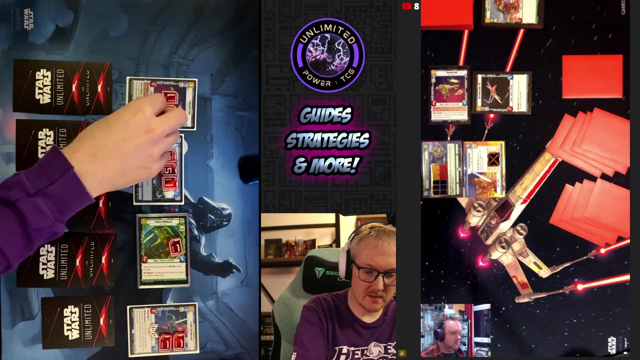 Mm-hmm, Let's give a plus one plus one, two, Luke, I assume. Oh no, it might be redemption. I'm thinking the redemption To keep it alive that bit easier. Yeah, let's put it on the redemption. 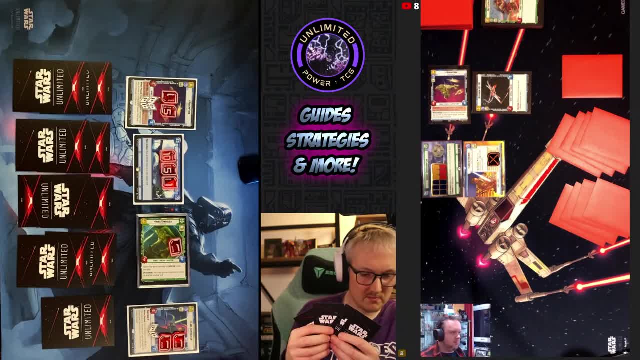 So it's an eight Six at the moment. Yeah, sorry, eight four at the moment. I've taken six, got 11 total health. Yeah, Okay, cool, All right. Oh sorry, it's got 11 total health. so it's an eight five at the moment. 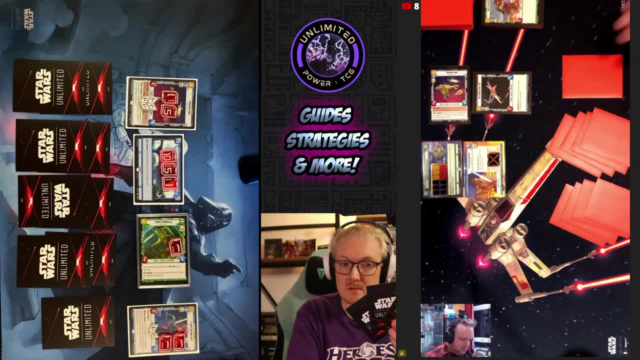 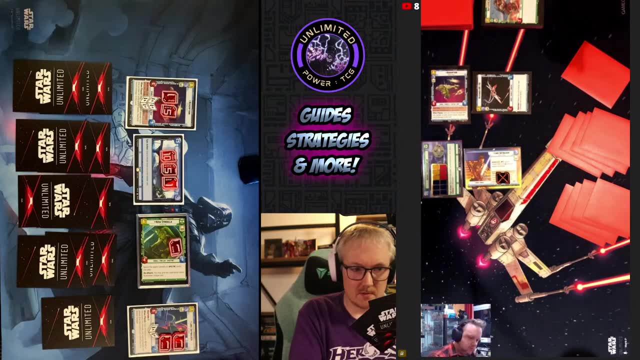 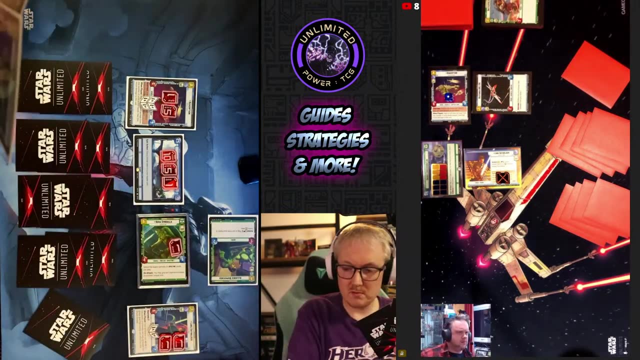 Yep, that makes sense. All right, Okay, I will pay my last resource and tap Luke to give the redemption shield. Nice, Okay, so I'll pay one resource to put in an alliance dispatcher. Yep, Yep, I will. I will retain the initiative. 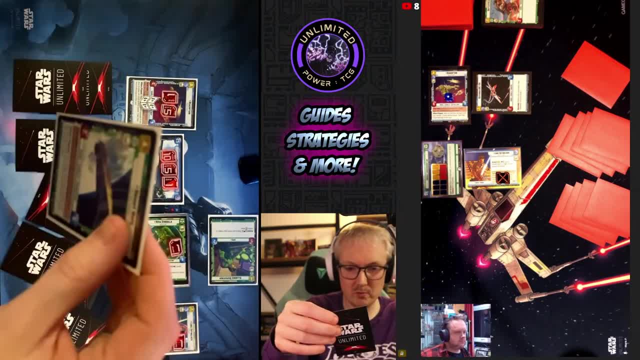 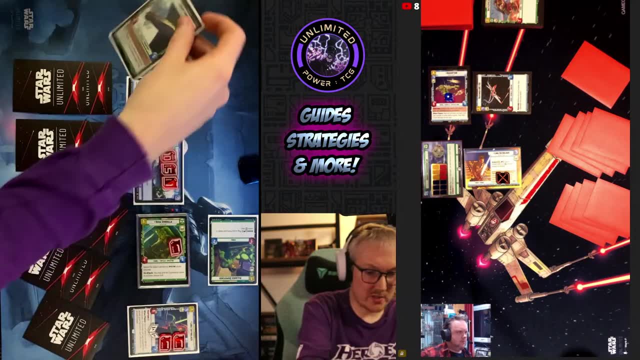 Okay, I'll pay four resources to play. a bright hope. When played, you may return a friendly non-leader ground unit to its hand If you do draw a card. Yep, I don't think there's any point. I don't think there's much point. 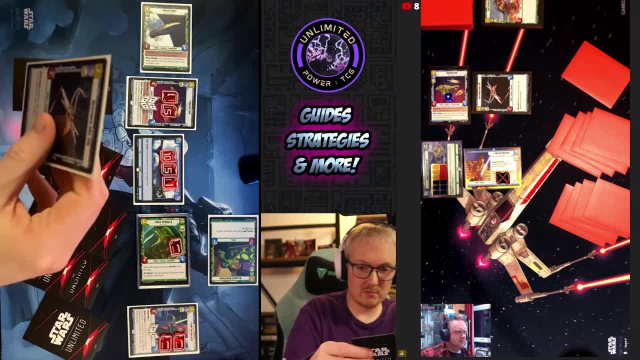 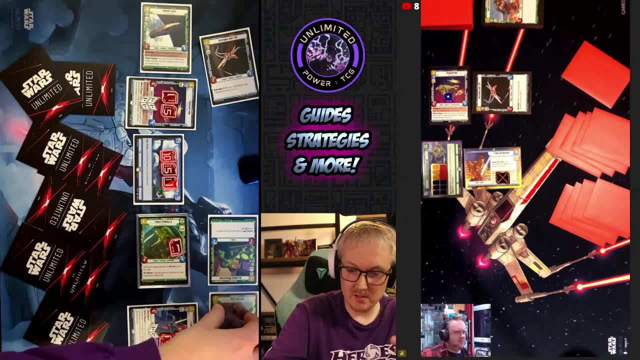 I'll play two more to put a restored arc- Yep 70- into play- Yep. And then I'll play one more to put Bail Organa into play- Yep, Okay. And then I guess I'll swing at your base And then I'll heal my base with Luke for seven. 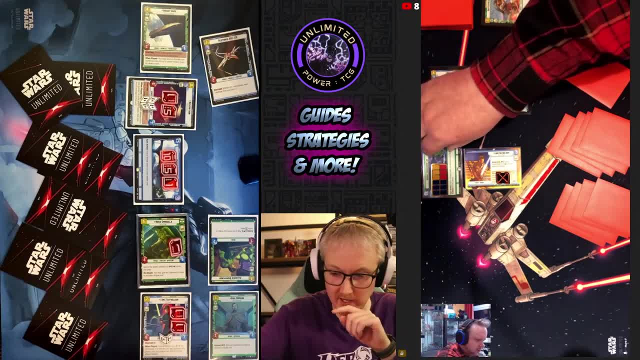 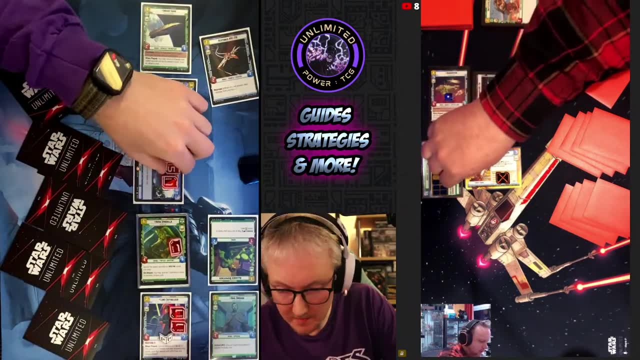 Seven And I'll heal my base for three. Can I Hold on Restore three? Can I heal other units? No Restore by its definition is only the base. So I'll go down to just 13 damage on my base. 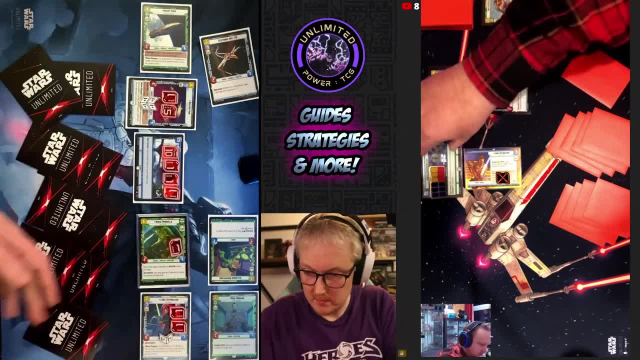 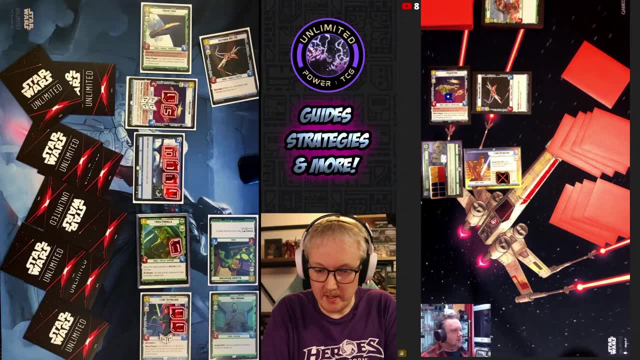 I'm back up to 12. health: Oh great, You took board control pretty effectively at that point, didn't you? Okay, Cool, Okay, Okay, I'm done pass. So all right, here we go again. We might not get much time in for a best of three at this. 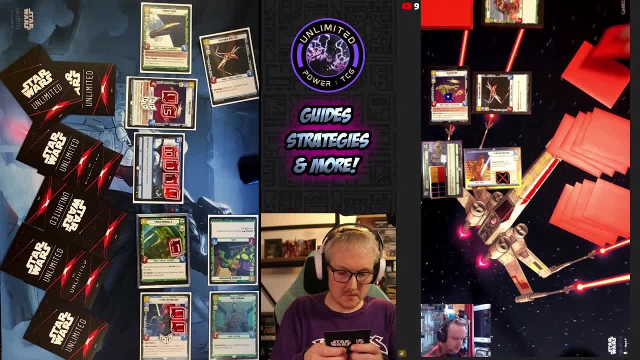 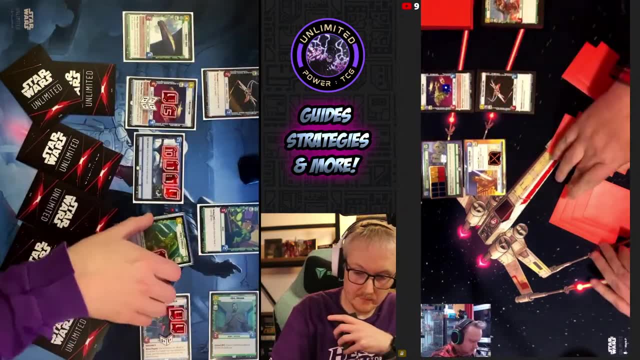 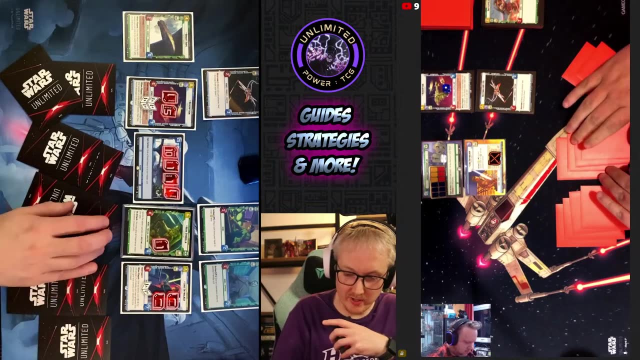 Uh, I'm going to resource that and let's ready up Okay. Sometimes, though, when the games get long like this, it's the best type of game. Yeah, it can be, Cause I mean I was down at one hit. 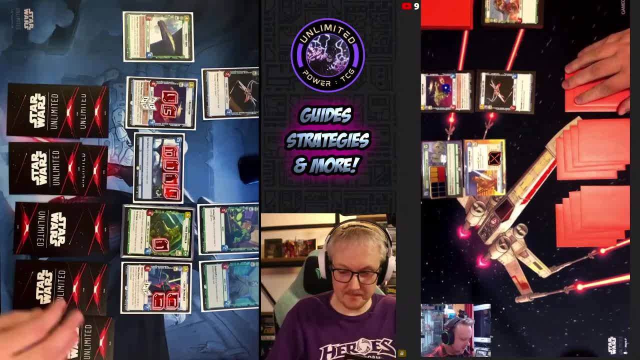 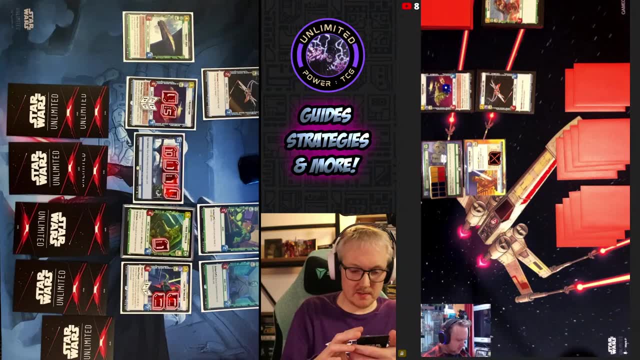 I was down at one point, right, Yep, You were very, very close to death. You managed to pull it back very, very effectively. We'll give you that. Yeah, I'm not going to resource up the thing this time. 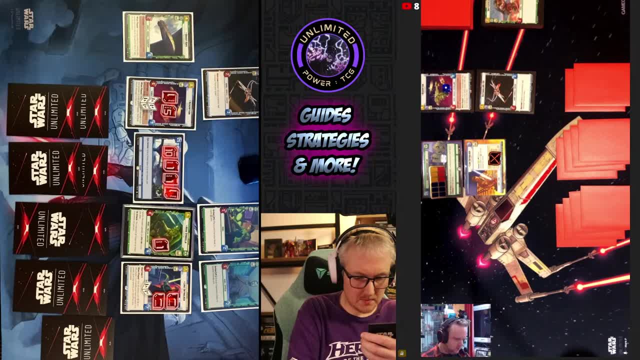 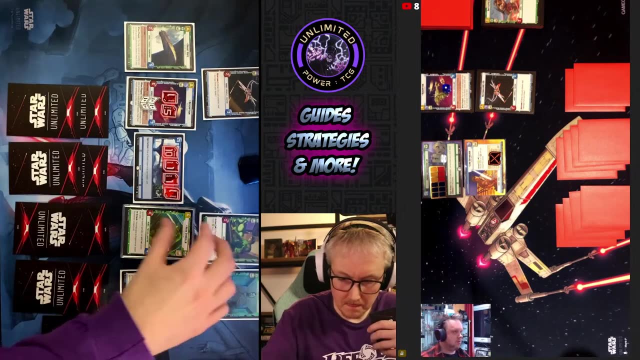 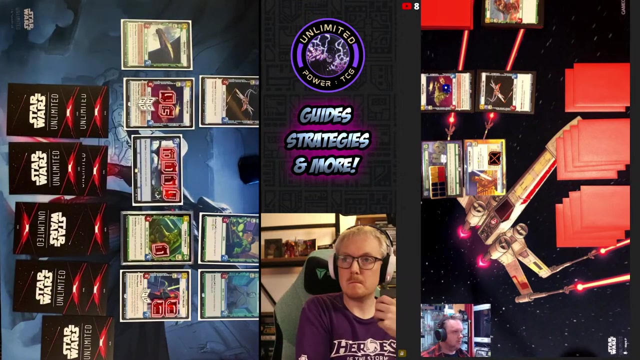 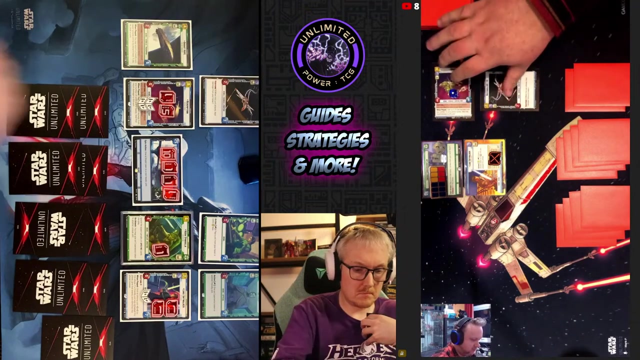 I've got 10.. You're not resourcing, Fair enough, Right? So, um, we can do that. We can do that, Which will ping shields off. Um, you're right, Let's kill the bright hope with my redemption and lose a shield. 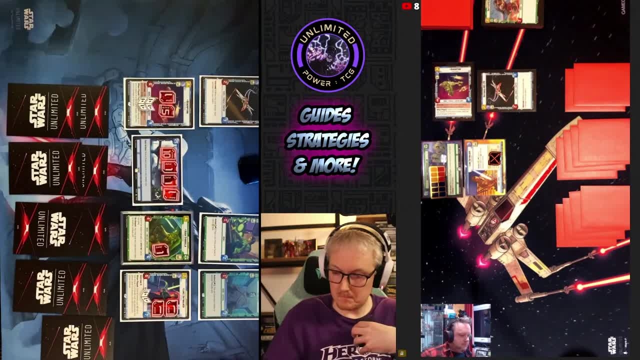 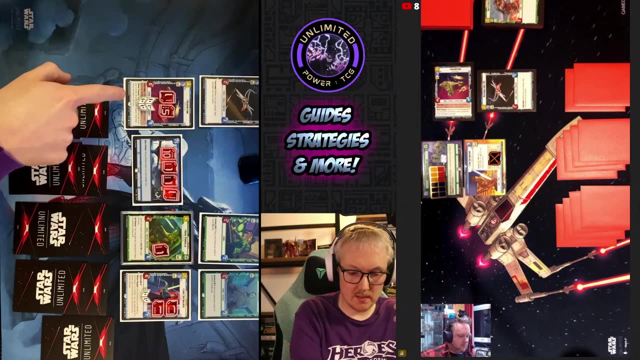 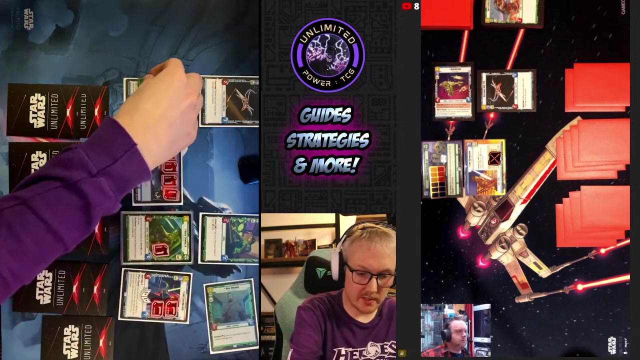 Okay, Yes, Yeah, Okay, Thanks Bye. your bright hope has 9 health. my redemption has 9 health. I'm going to tap bail to give an experience token to another user unit. I'm going to give it to my redemption. great, wonderful. 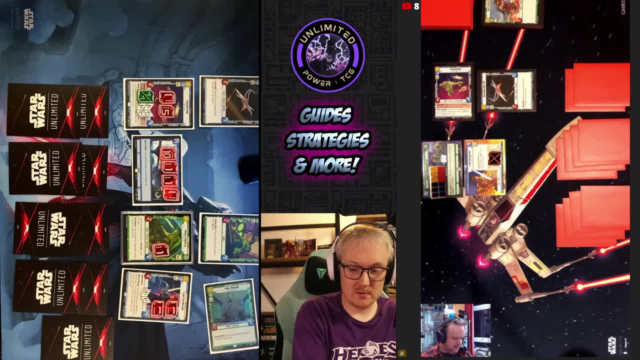 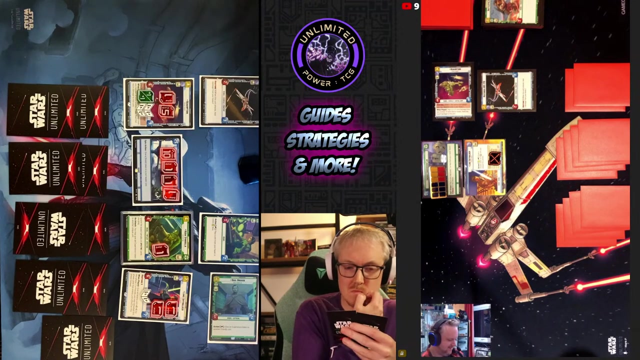 so it's got 9 damage. now it has that makes it 12. so it's got 6 health remaining. so it would die as well. I'm going to make a very risky play now. I'm going to pass. I'm not passing, I'm going to attack your base. 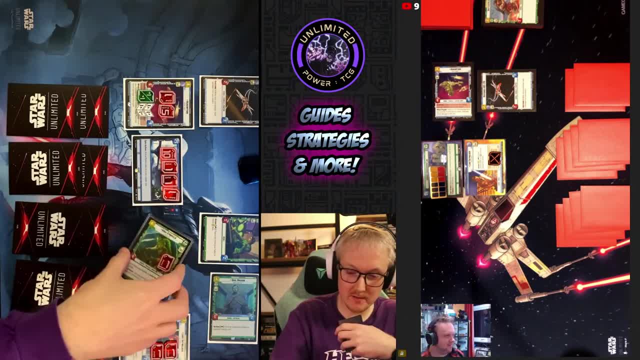 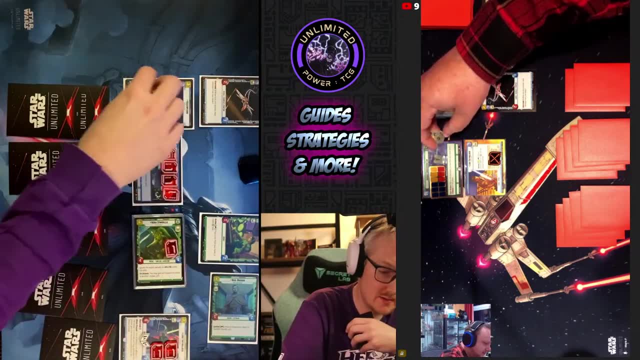 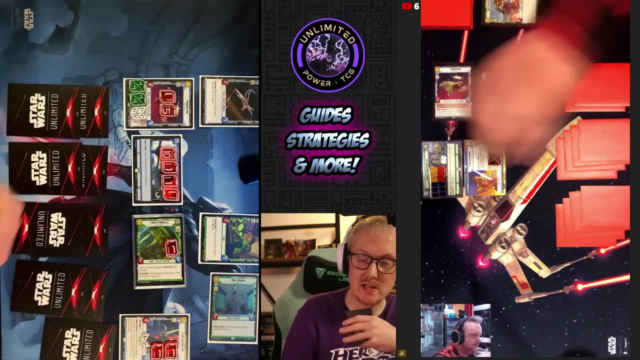 with Hera for 4. I'm going to give my bright hope a plus 1 plus 1. sorry, my redemption. another plus 1?? so it now has it would be 13 minus 6. so it's got 7 health remaining now 7 health. 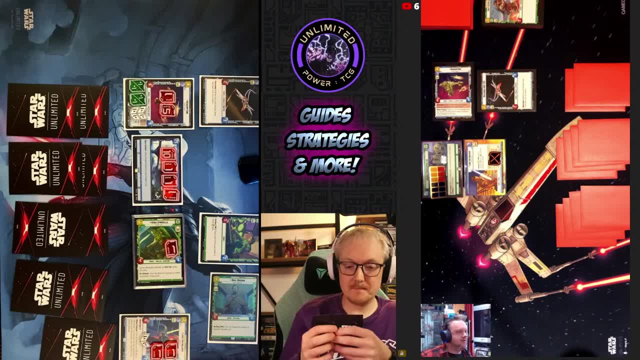 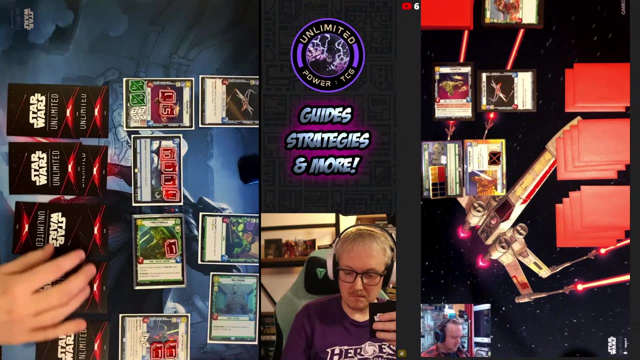 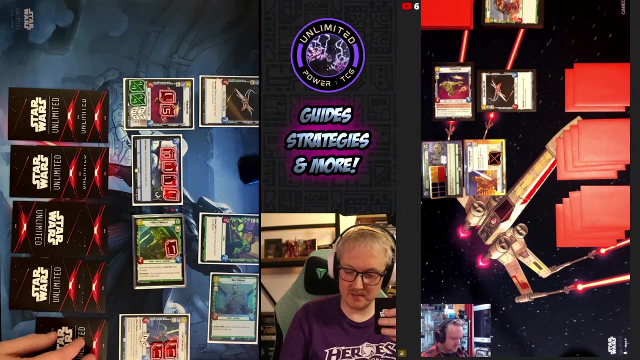 so it won't die to my redemption. correct, right? how badly do I want to play this. this is when you need that shitty moment of glory card that no one ever puts in their deck, doesn't it? moment of peace, moment of peace. I do consider running some zero cost cards. 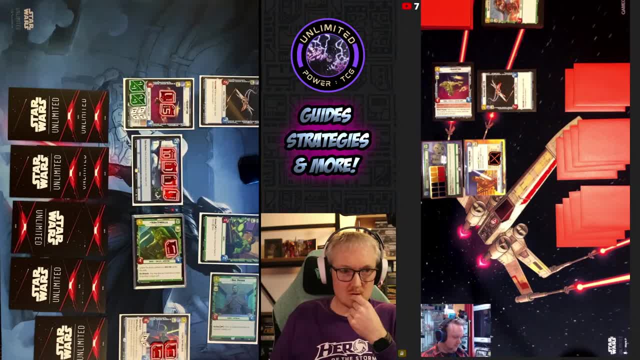 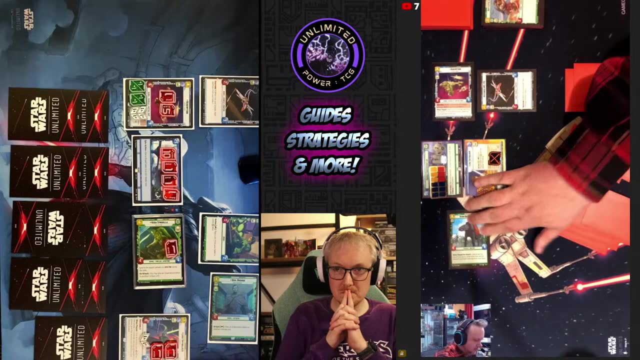 I just don't ever seem to find a famous space. I don't think you've got too much there, really, so I'm going to have to play in another arena, I think? alright, let's pay 8 to bring down a reinforcement walker in the ground arena. 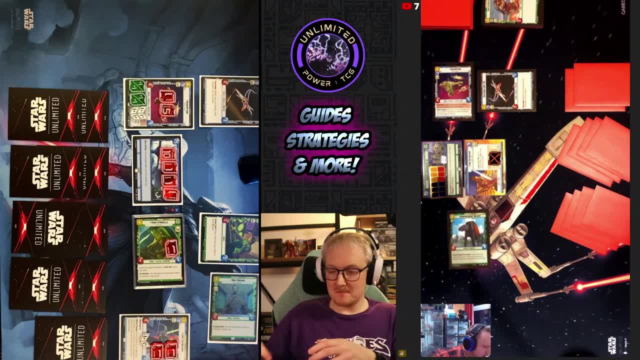 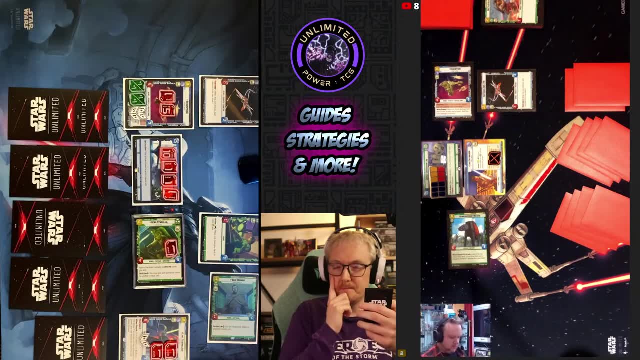 this is a 6-9 when played. look at the top card of your deck. either draw it or discard it to heal 3 damage from your base. yep, so I will leave that on the top. it's a 6-9. it's a 6-9. 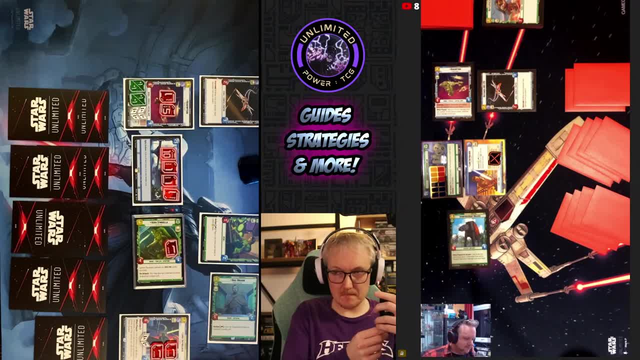 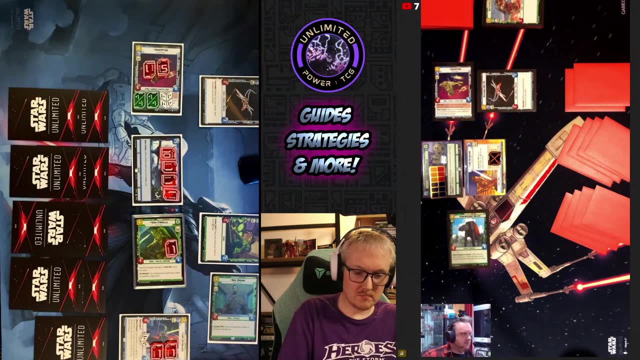 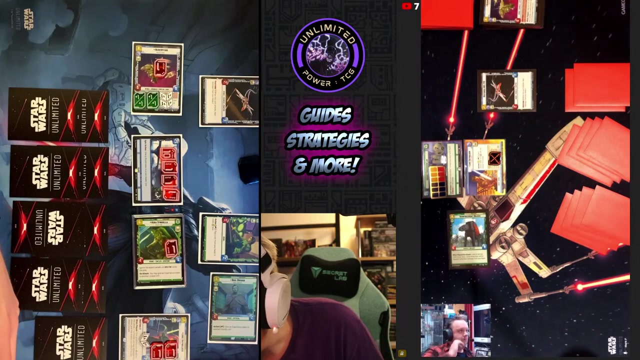 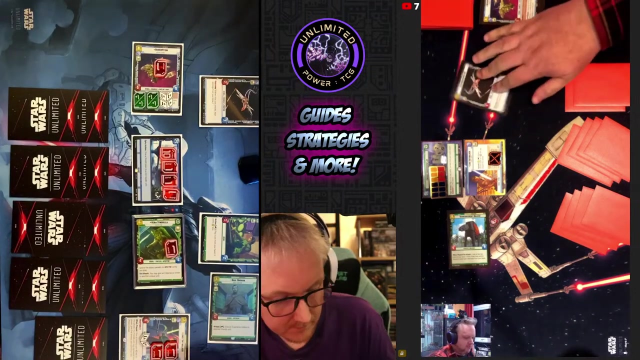 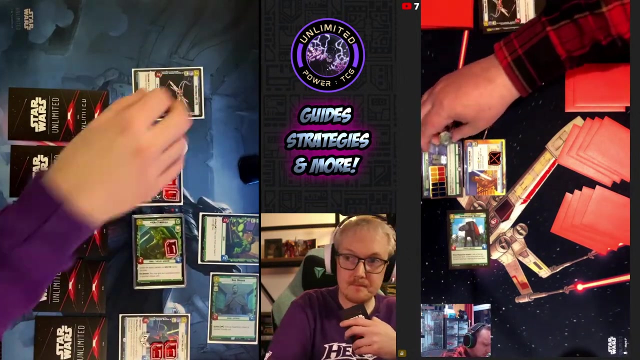 ok, let's, let's see. well, kill your redemption, yep, and take 6 damage in return. so I just leave one on him for one hit point. it's what he's got. ah sure, no worries, not a problem, right, I will attack your redemption with the restored Ark, killing both and healing my base for one. 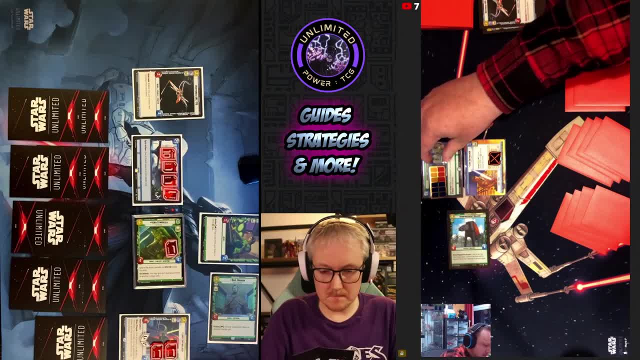 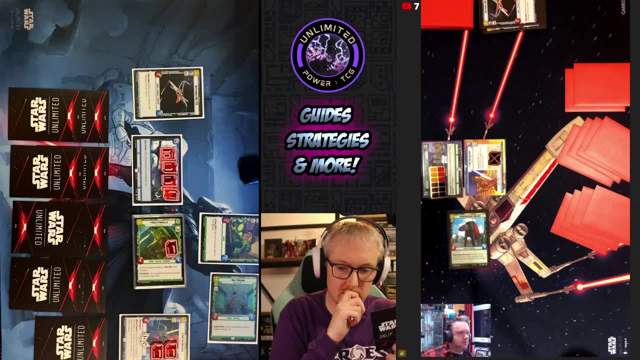 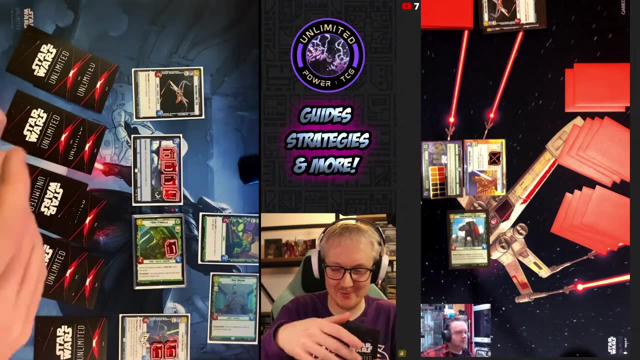 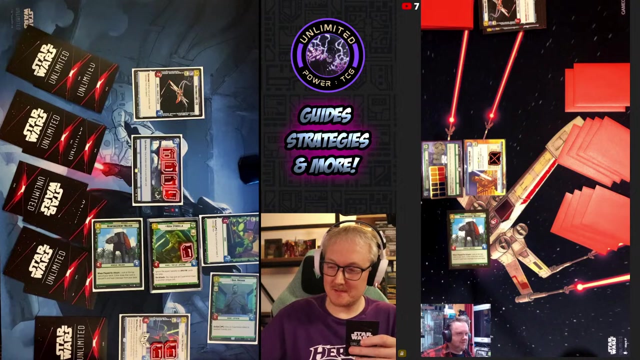 Okay, I'll play my. Is there any point in tapping the spectrum? You do only No, I'm going to play 8 as well. Yep, to play Enforcement Walker. Oh, okay, So I can look at my top card. Yep, I don't need this, so I'm going to. 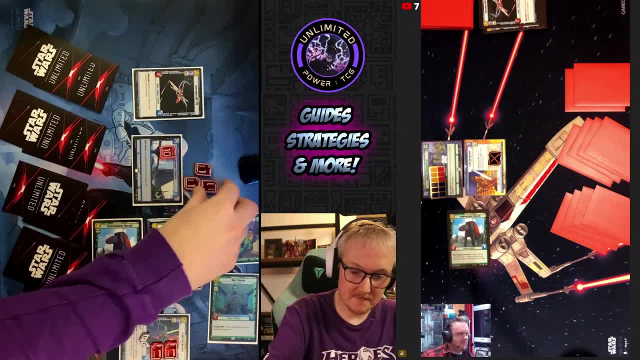 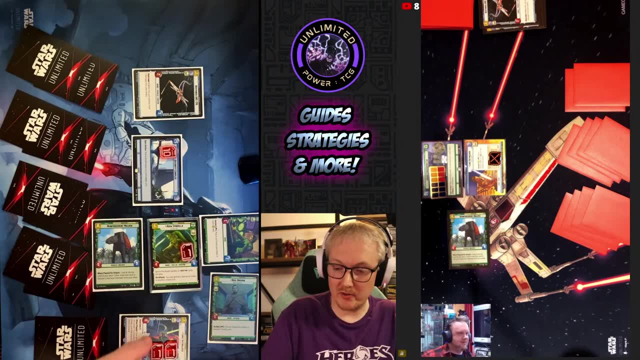 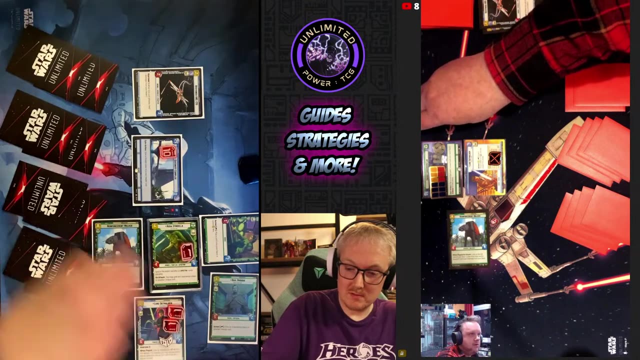 discard it and heal my base for 3 A resupply, fair enough, Oh, this is very slowly going your way. And then I will attack your base with Luke for 7, Okay, Which it puts me up to 23, And then you can do 1 damage. 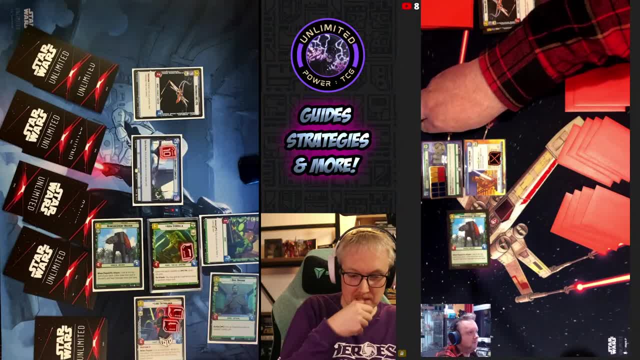 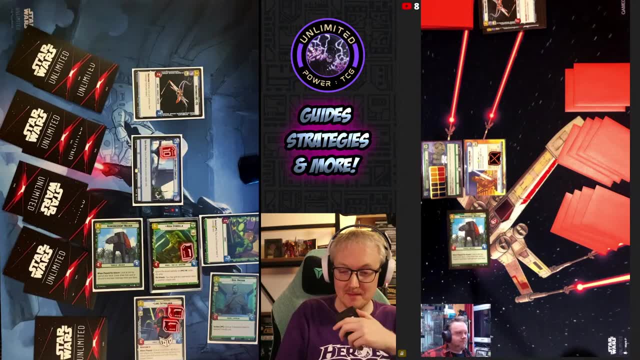 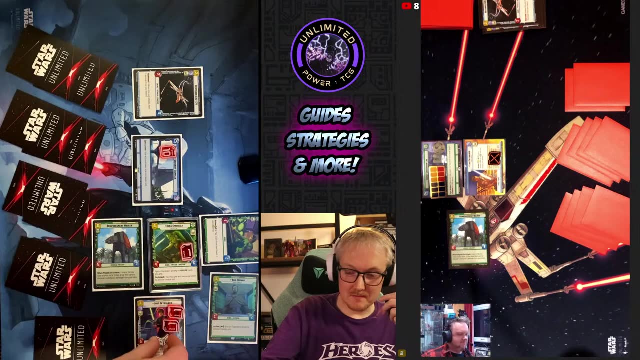 with the Alliance Dispatcher and 2 damage with the Restored Arc, which will win you the game. Gretz, you've got it, We got it, You've got it. What a swing man. Yeah, Very good. I literally couldn't have. I got that Redemption at just the right time, man. 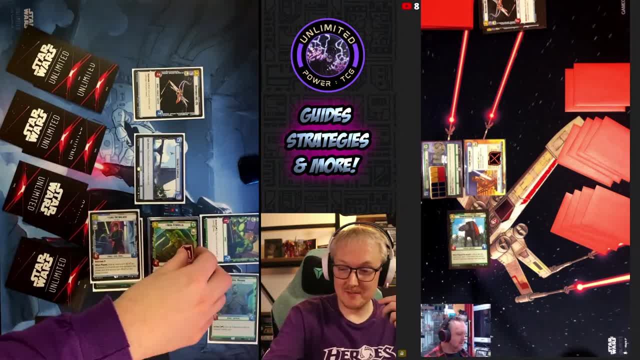 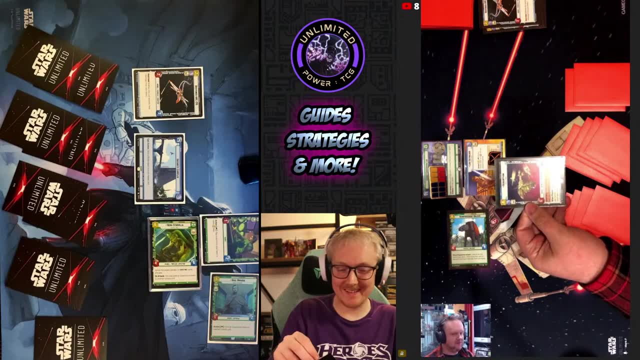 You're absolutely on a knife edge there, yeah, So what I was trying to decide, though, is whether or not I play the Reinforcement Walker or wait for you to kill my Redemption and then play 8 resources to play another Redemption, But I wouldn't have thought that would have made enough damage. 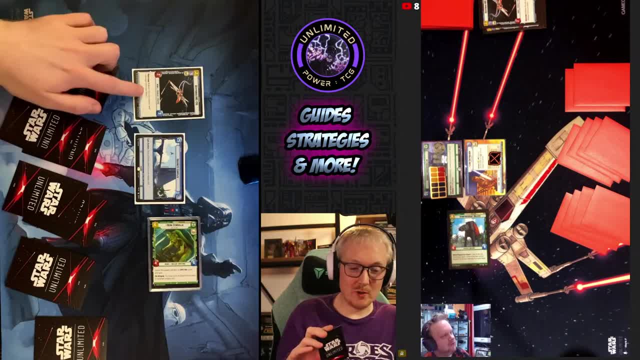 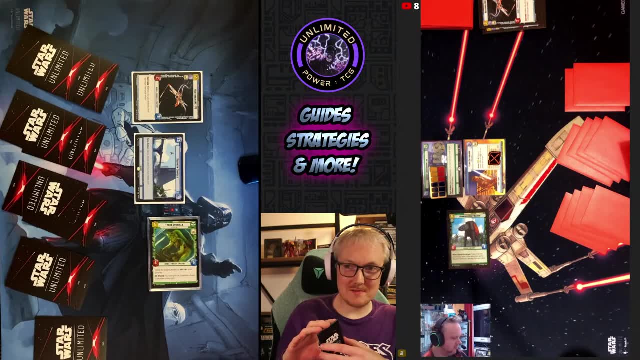 Maybe it would have made the difference, because you wouldn't have been able to do 2 more damage with the Restored Arc, so And I could have healed by playing it. So maybe playing the Redemption would have been the better. We can do that if you want. 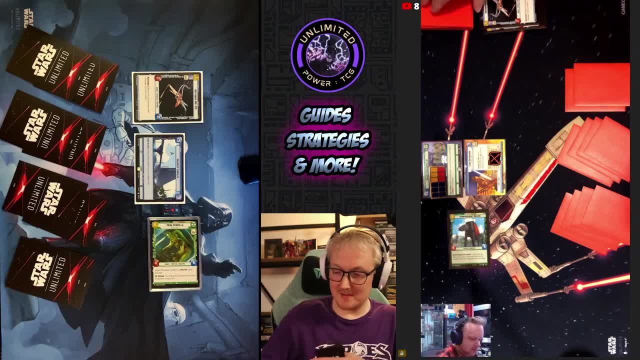 We can continue the game. No, no, no, it's all good, We've made a decision, it's fine. The reason I left my card at the top that I did was because I was preparing to kill Luke. the following turn with this lovely little card here. 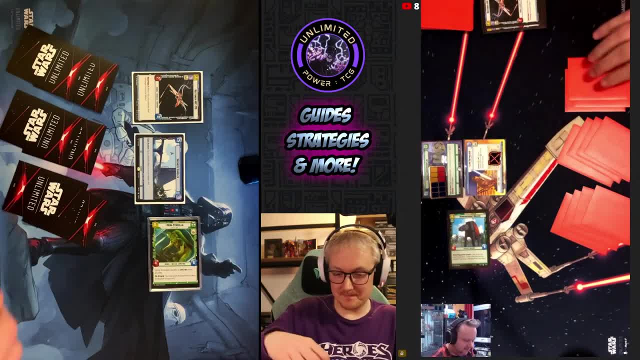 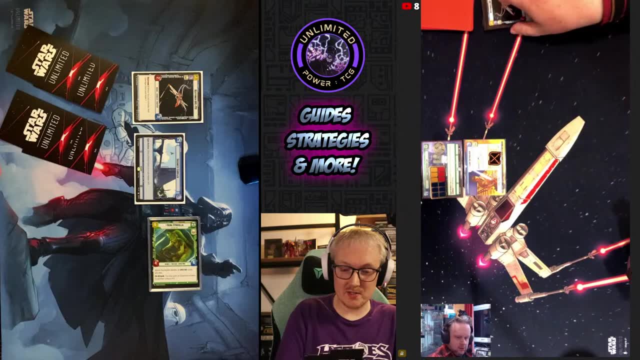 Oh, with a nice sick little Vanquish. Yeah, so Cool. No, you just sent it out there with the amount of damage that you were doing. so props to you. Yeah, You're taking this to the tournament tomorrow, are you? Yeah, that's right. 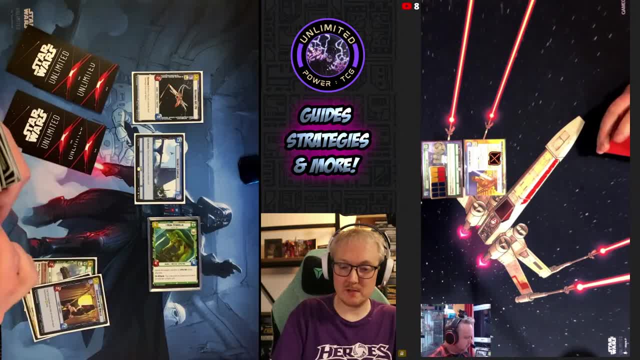 Cool. Do you have time for another game, or are you trying to get an early night's bed? Yeah, sure, let's do it. I am making an early start tomorrow, but it's fine, we can do it. It's going to be a long day. 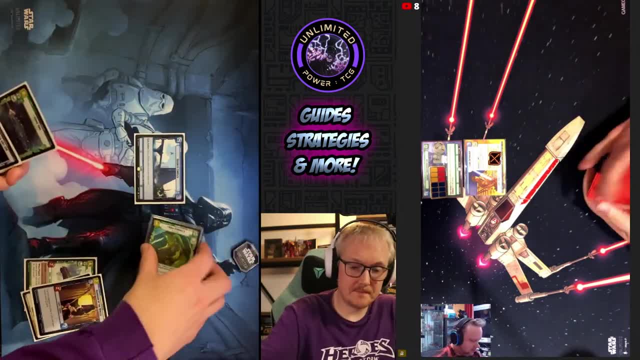 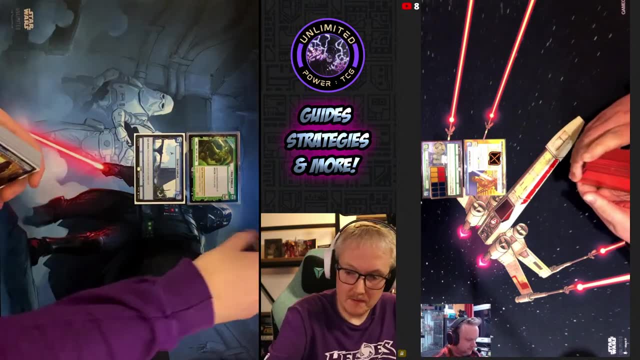 How many games do you play at the tournament then? If So, They're starting checking at 9. It's an hour and a half drive. Oh, wow, okay, The tournament starts at 10, and then, if you make the top cut to go through to the final. 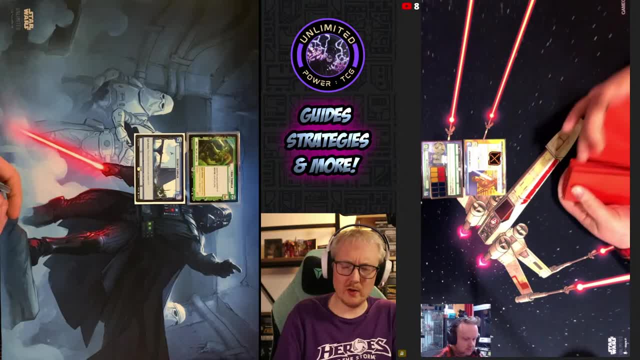 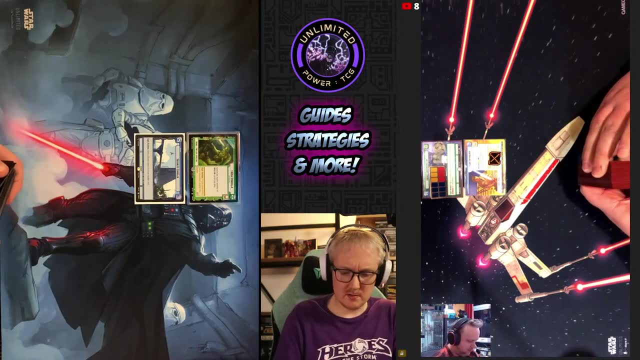 You'll be playing until about 8pm. Wow, so you must play a lot. You might not make the top cut, though I might not win, But Yeah, So it's like best of three at the event. Yes, 55 minute rounds, best of three. 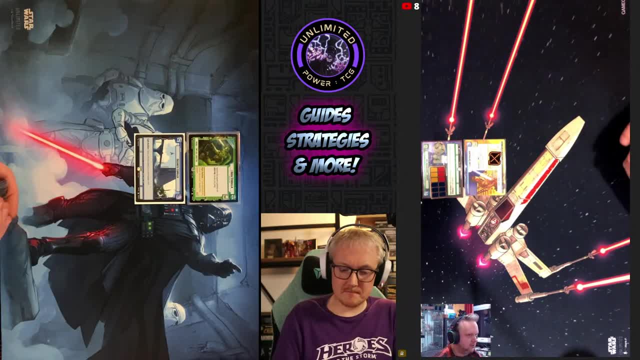 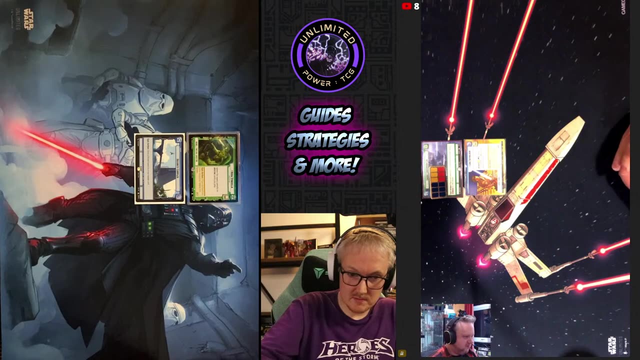 Okay, Alright, let's see, It's a long game. I was going to say that was quite a long game. Well, I think any other card except that redemption on that pool and you won the game. Well, there we go, I will, because I lost. I get to choose whether to take the initiative or give it away. 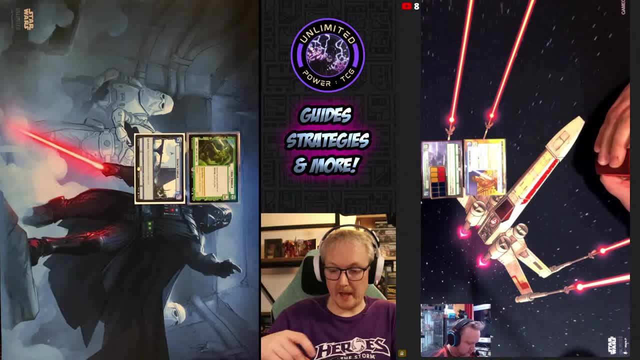 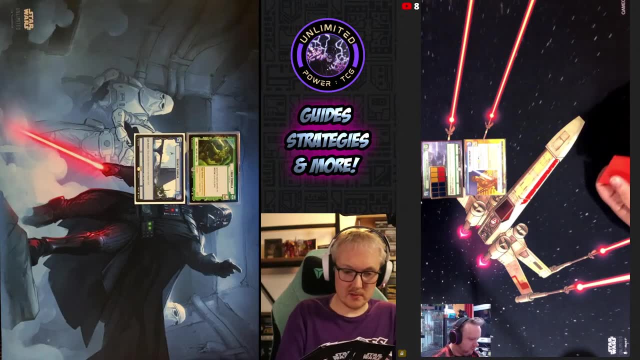 I will choose to start the game with the initiative. Alright, I probably only have time for one more. Yeah, sure, So let's see if you can win it and then even it up at one game each, Or if it ends in a draw. yeah, ooooh. 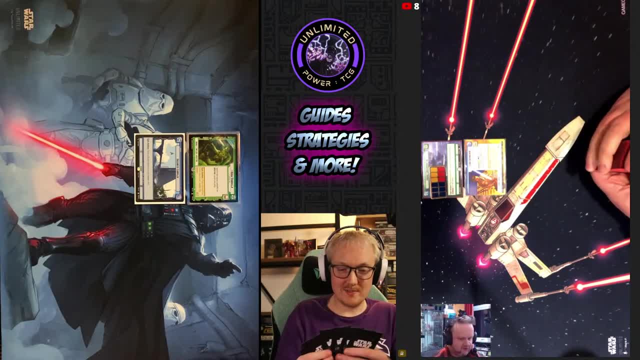 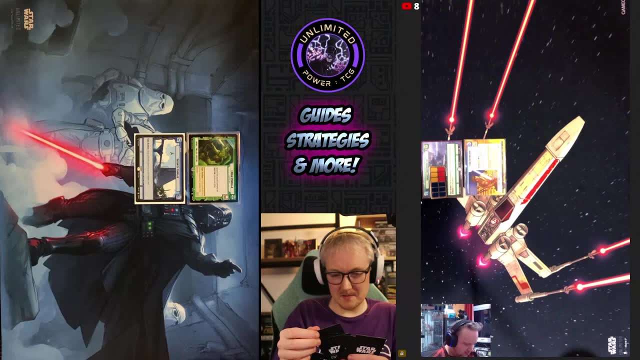 Well then, everyone will have to tune in for next week's stream. Unresolved attention. yeah, Cheers, Phil. That was a very close game. that was absolutely on a knife edge there. you're absolutely right. I made some bad decisions there that cost me the game. 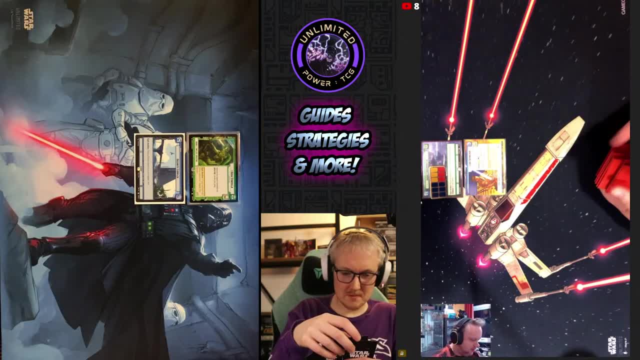 I could have done things differently with hindsight. Okay, So this resulted in me wasting resources when I could have spent them. I also made no use of the ECL, which is a shame. 1,, 2,, 3,, 4,, 5, 6. 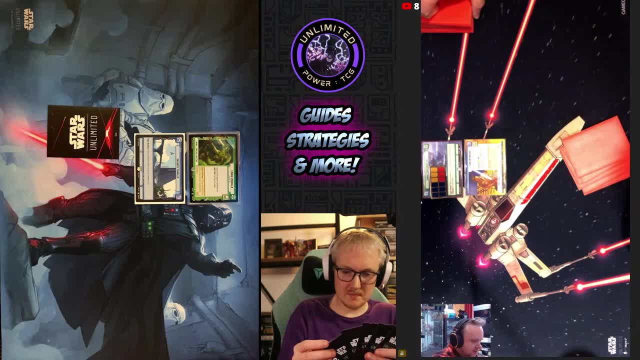 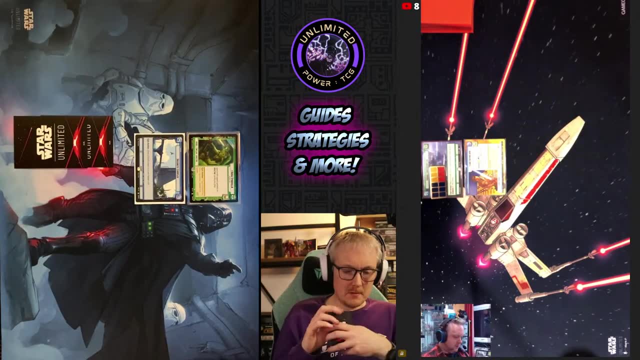 Oh, you never used your ECL, did you forget? or you just didn't have a? The right opportunity at the time didn't quite crop up, Okay, Which I've noticed a few times with this deck. Okay, This is not the best starting hand in the world, so 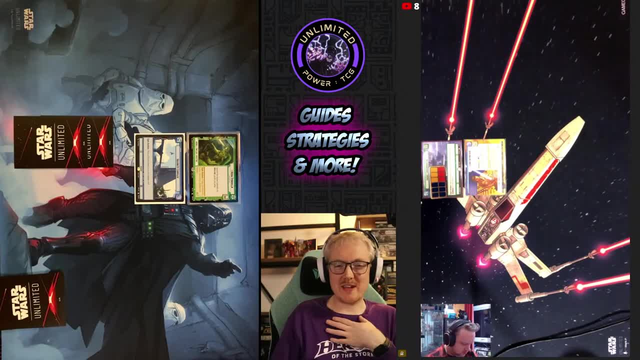 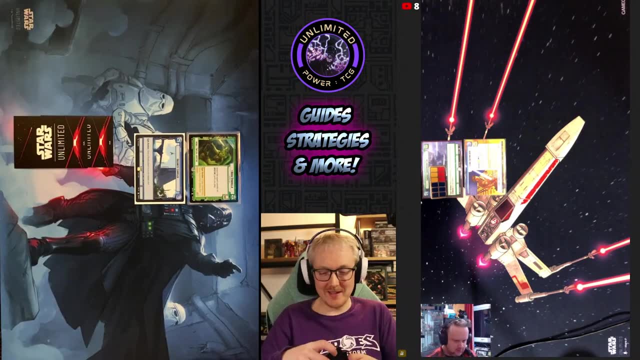 Let's mulligan that. Well. my hand last time was all sixes and sevens, With the mulligans as well. this time it was all ones and twos. so It was probably too many ones and twos, but I'm like F it, I'm keeping it. 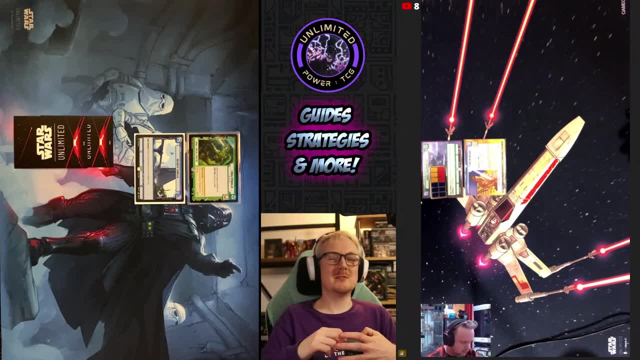 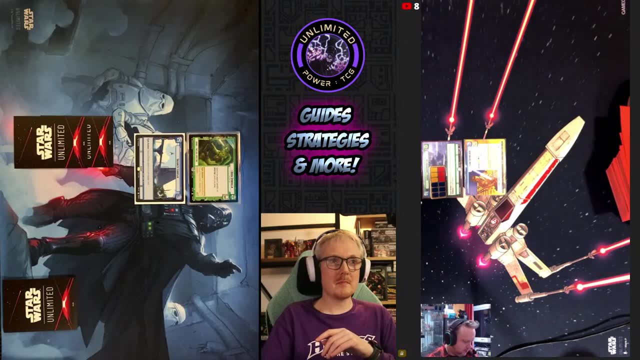 Yeah, you can always play them through. Yeah, I'm just gonna play them all And resource the ones that you don't want. it's nice to have the flexibility Right. so 1,, 2,, 3,, 4,, 5,, 6, this is the hand we're stuck with this time. 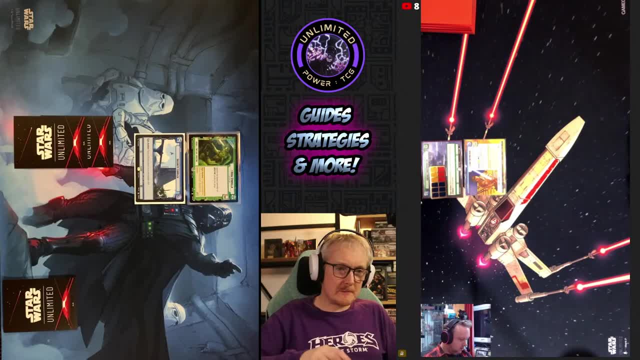 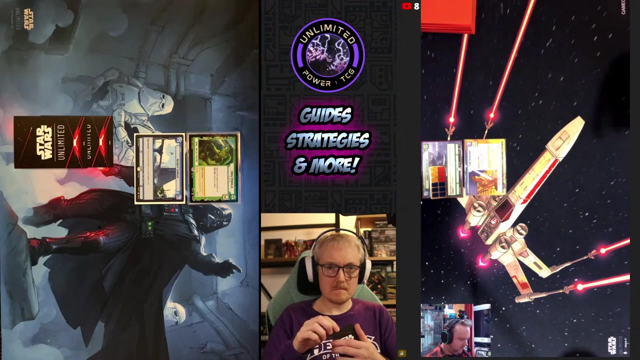 How bad are we? We're not horrifyingly bad. Okay, good, Not great, not bad. I think we're gonna do that and that, Which means: Oh no, oh no, Let's do that, that'll be more fun. Right, let's resource you. 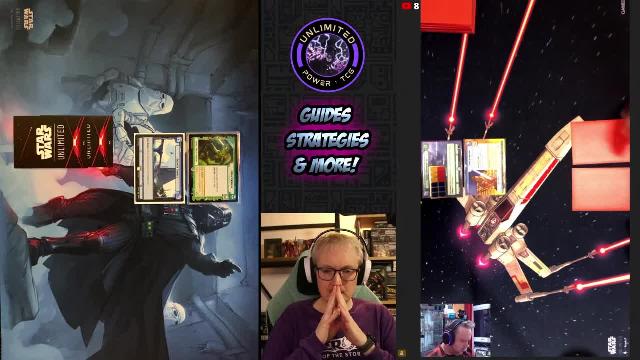 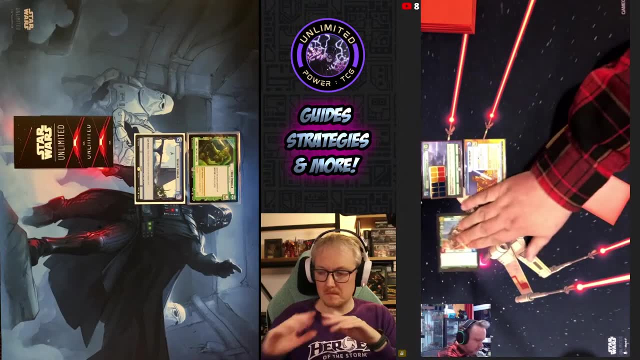 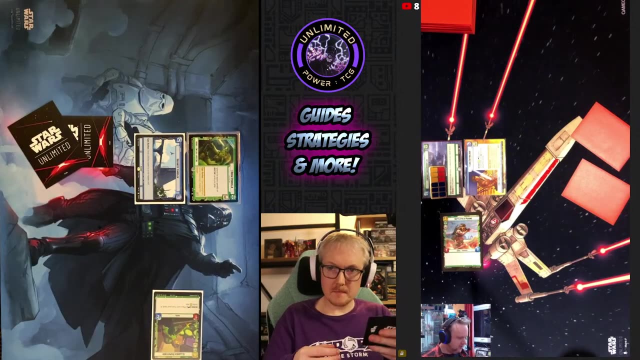 And let's resource you. I'm ready, you ready, I'm ready. yep, Awesome, let's exhaust two And play the Battlefield Marine once again. Cool, let's exhaust one and play Alliance Dispatcher. Seems fair. I will retain the initiative. I'll resource another one to play a Vanguard Infantry. 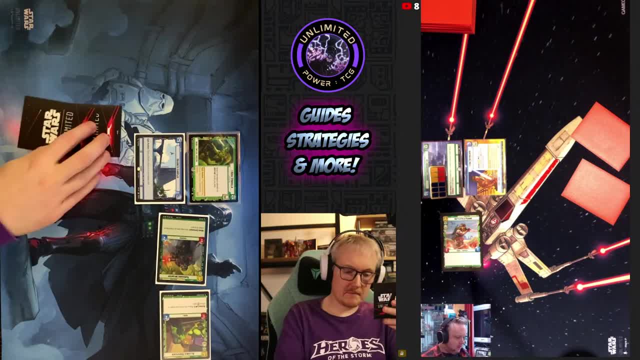 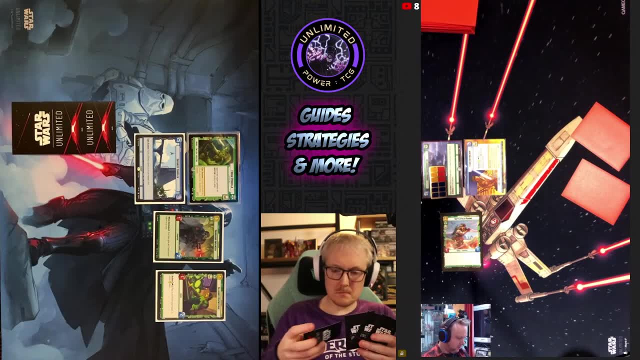 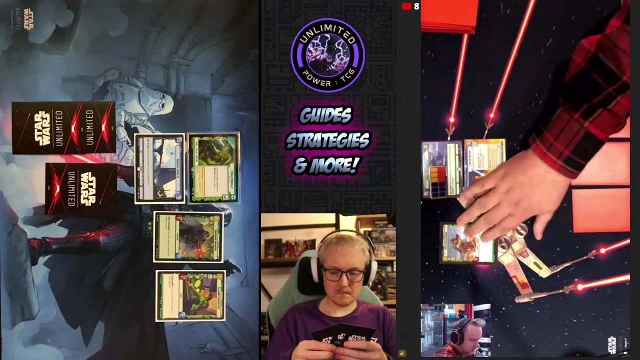 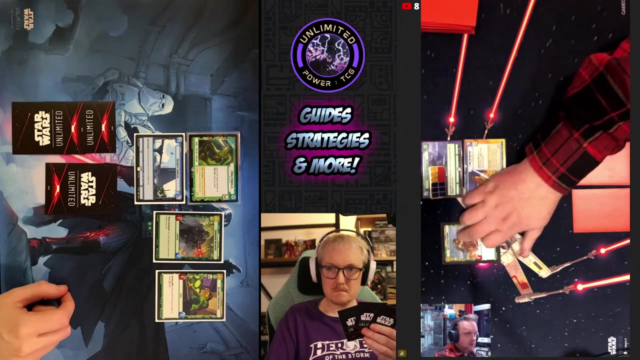 Okay, seems fair, I'm done. Alright, draw two, You can stay, you can go and ready up. Alright, I have the initiative. so I know exactly what that thing's capable of. so let's kill the Alliance Dispatcher. Oh, it's good, isn't it? 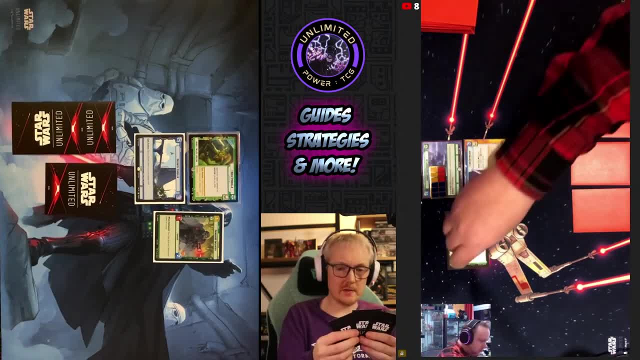 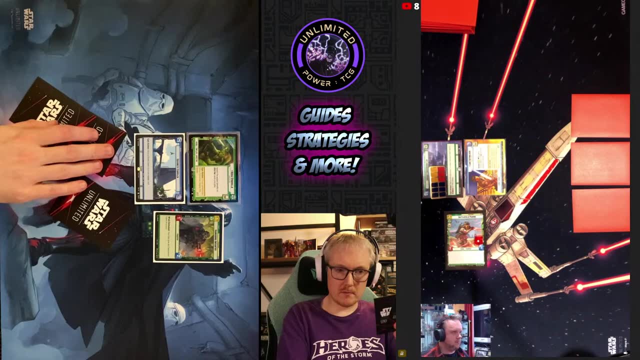 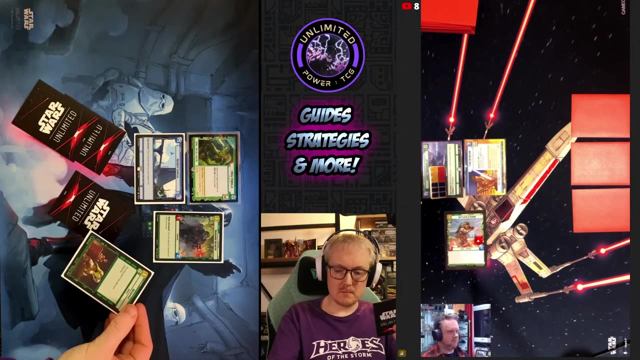 And take a point of damage in return. I do like the Dispatcher. I really like having three in my deck. I will tap Yeah, okay, three to play Resupply. Oh interesting, Does the Resupply come in? exhausted the resource from it? 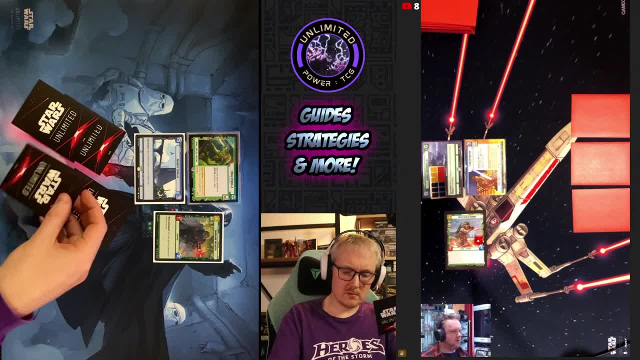 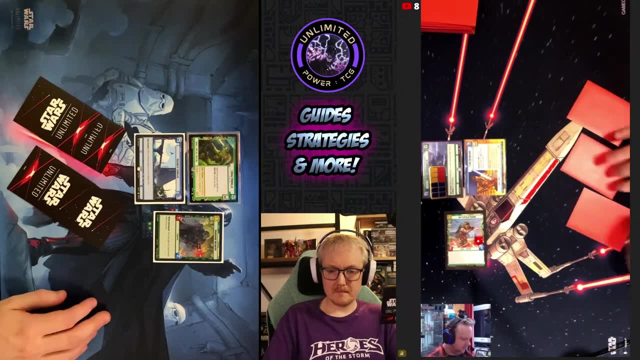 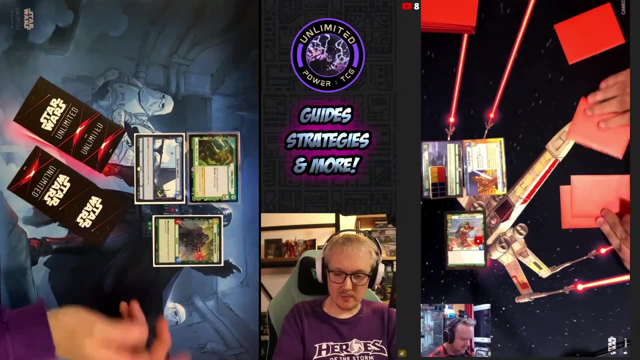 So all resources, Everything that you play, comes in exhausted, unless they say otherwise. Okay, perfect, Cool, so that's your shot. Alright, I will pay three to play a Resupply. Ooh, we're both racing. Okay, I'll attack your base for one with my Vanguard Infantry. 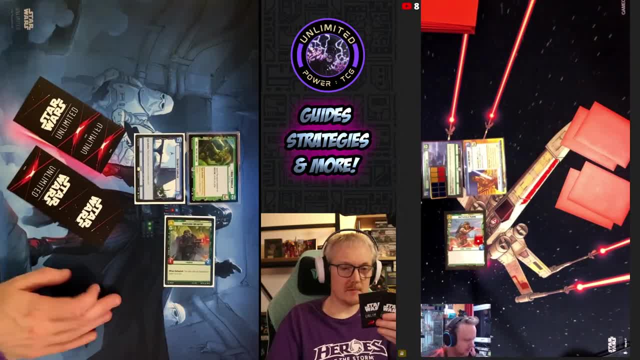 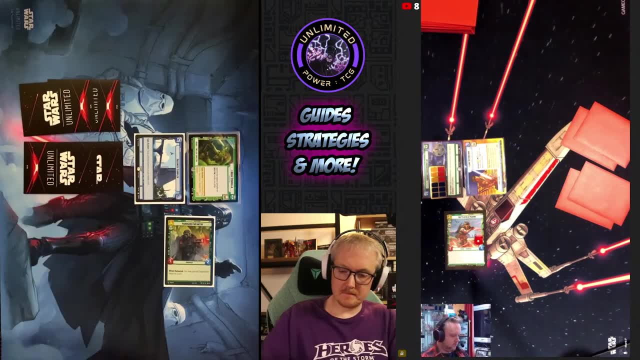 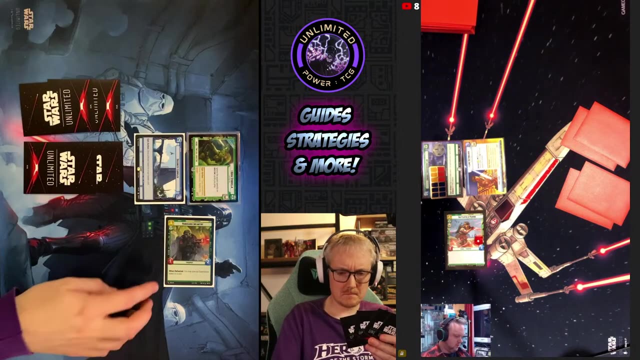 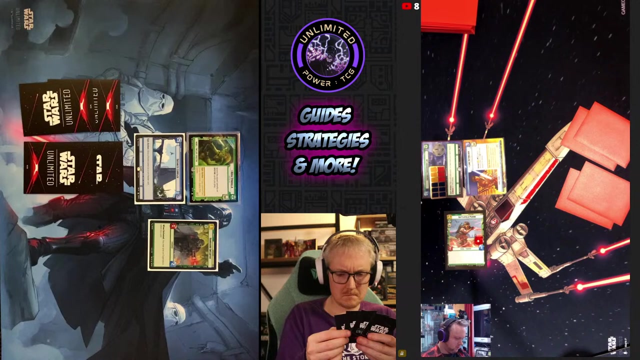 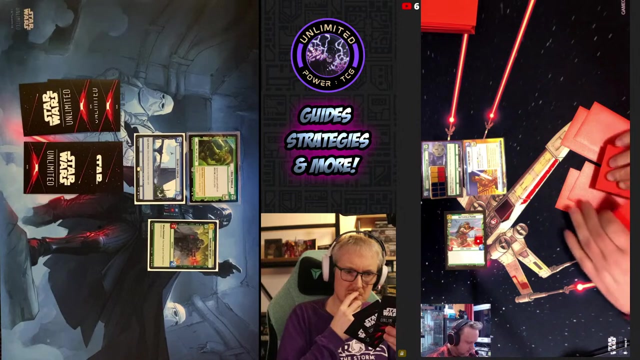 That sounds fair. I will retain the initiative. Okay, All done. Yep, Cool Draw two: Ooh Ooh. Now that's an interesting choice. Oh, man, it's. It's a very interesting choice. Yeah, I'm struggling to resource something here. I think I'm gonna have to resource this one. 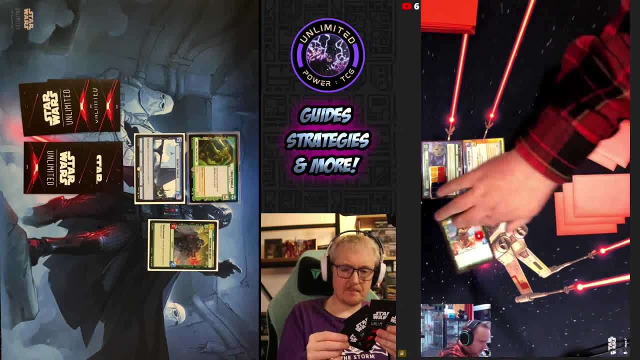 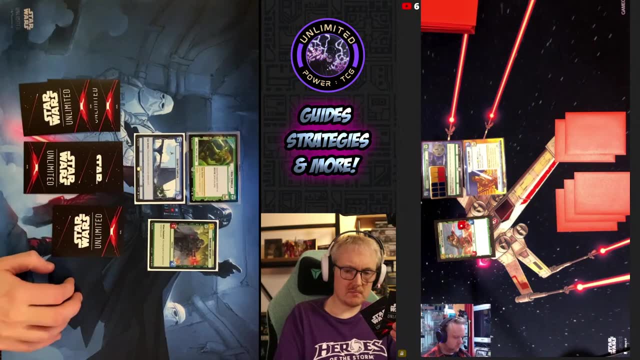 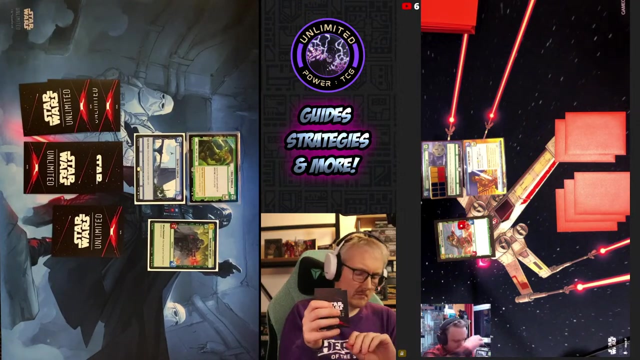 Okay, let's resource that. Okay, I really don't like it, but I guess I'm resourcing this. Okay, Your turn. Alright? Um, so, Which way round are we doing this? I think we're doing it that way round, So let's attack your base for three. 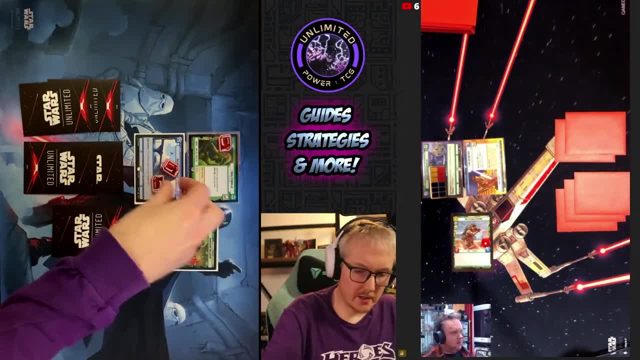 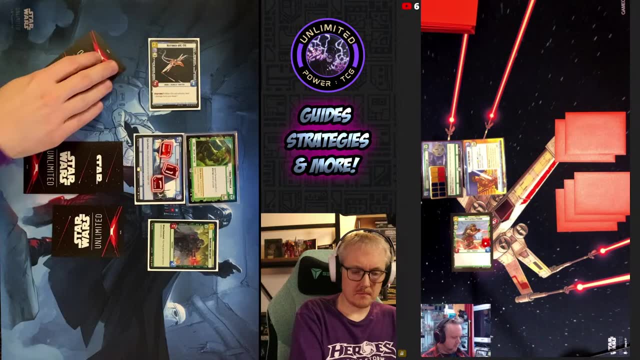 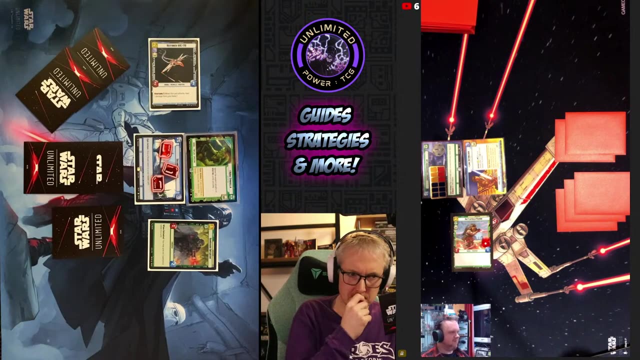 Perfect. Uh, I'm going to pay two To put a Restored Arc into play. Okay, Fair enough. Uh, Seems a bit of a waste really. Hmm, Oh, that's aggravating. Well, it's gonna happen. So, Uh, let's pay three. 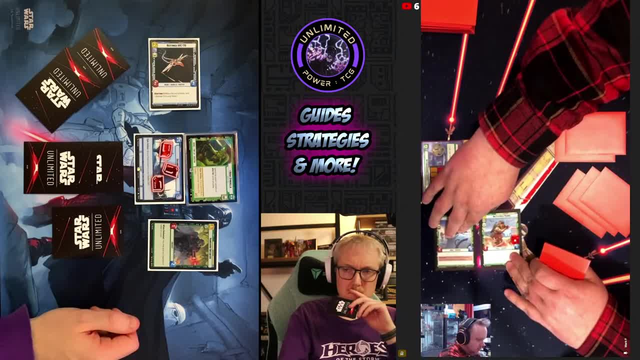 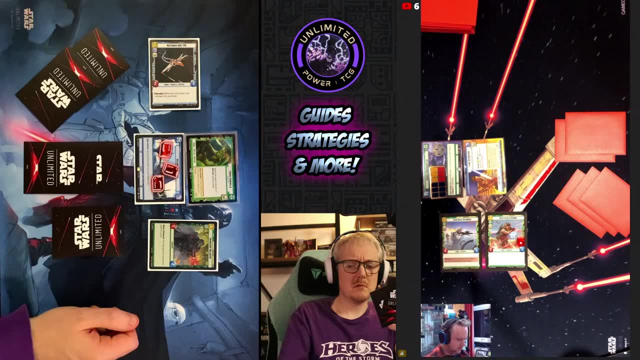 Mm-hmm To play an Echo-based Defender Which is a 4-3 Sentinel. Nice, Not bad for a three, actually, is he? Oh, absolutely, Yeah, it's great. Okay, um, I'm gonna take initiative then, I guess. 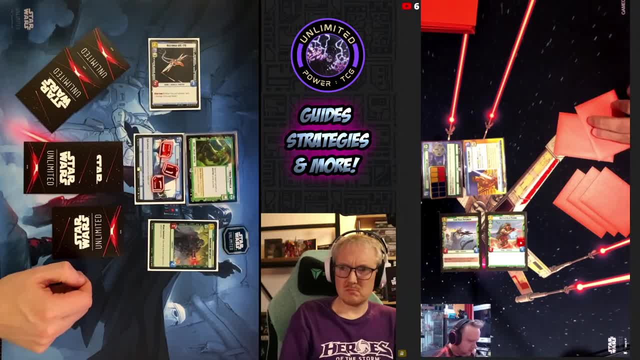 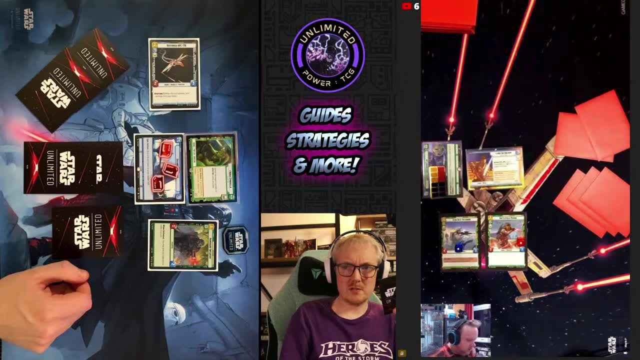 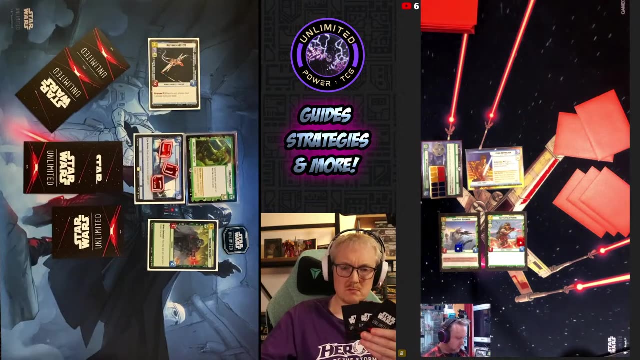 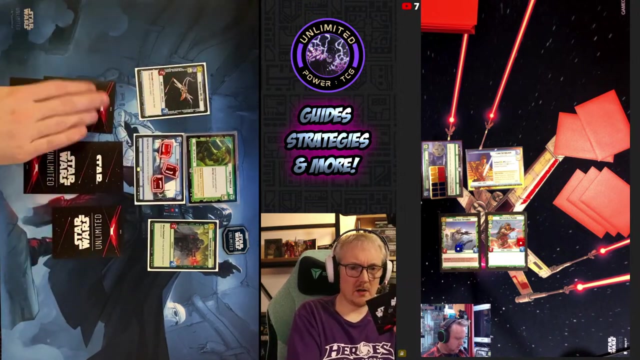 Oh, okay, Cool, Uh, I will pay one To exhaust Luke and give the Echo-based Defender a shield, As he is a Heroic Unit that has newly deployed this turn. Very nice, Um, and then I will pass Cool Two cards. Ooh, Okay, Uh, I will resource. 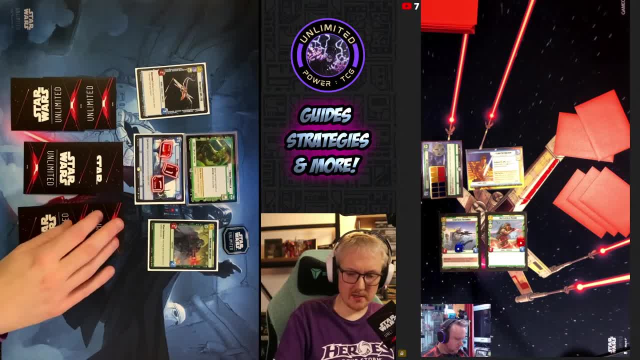 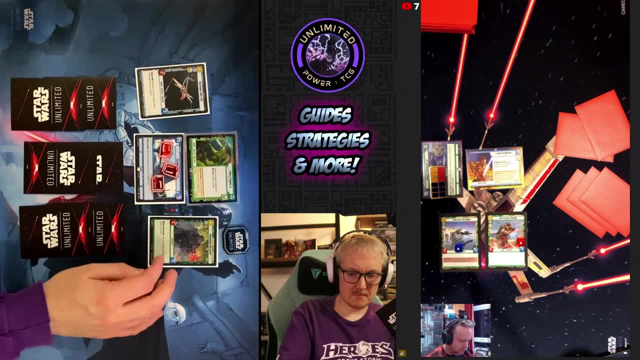 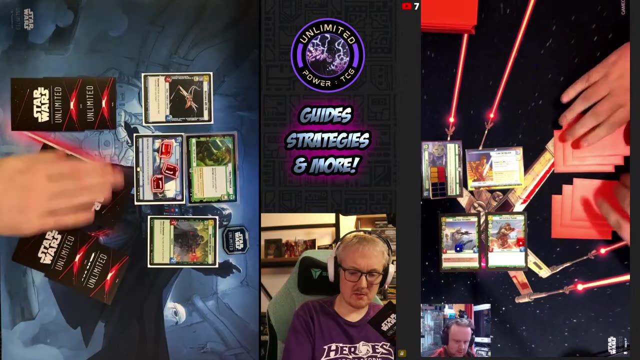 This guy And I. Oops, are you ready? Uh, bear with me. Yeah, I think we're gonna have to resource this. Okay, Are we ready? up, I'll place all six, Yeah, To play Obi-Wan Kenobi 4-6 Sentinel. 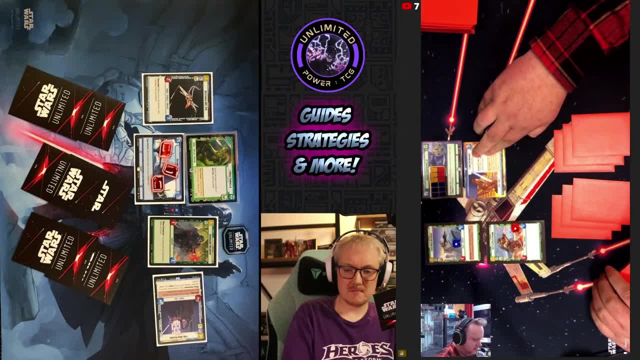 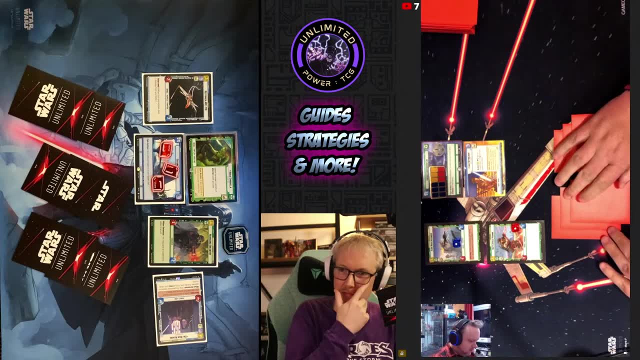 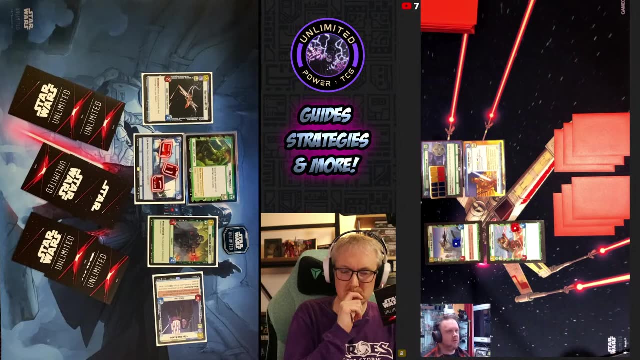 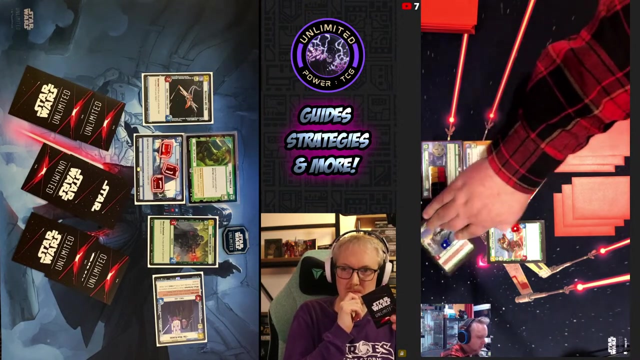 Oh no, Obi-Wan Kenobi. Who could have possibly seen it in a Heroic deck that's running in blue and green? Uh, True, Right, well, Um, You know what? Let's hit Obi-Wan for four. 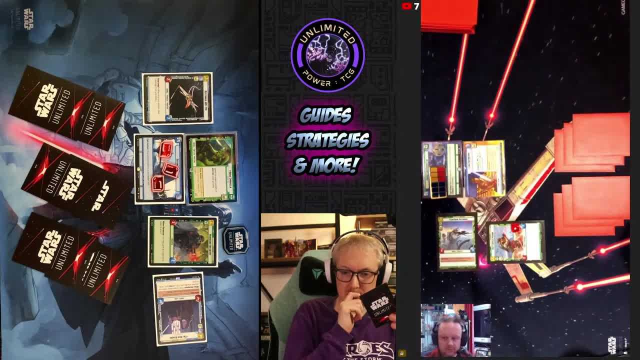 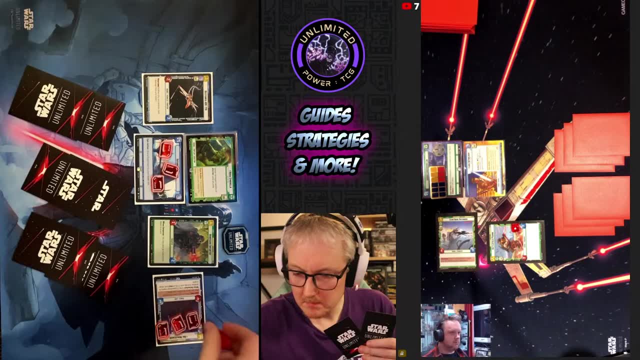 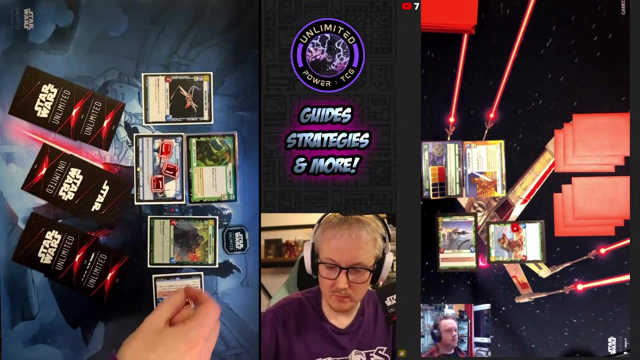 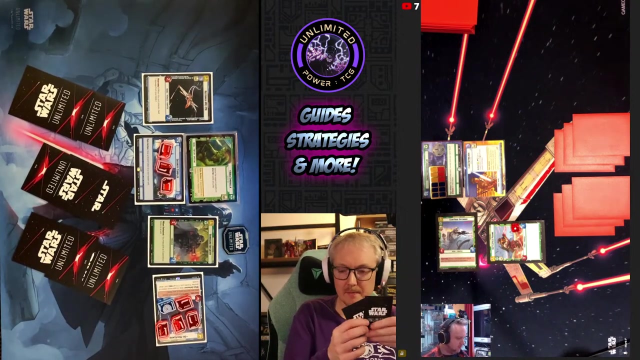 Very nice At the cost of a shield, Yep. Um, then I will Shield Obi-Wan With my Energy Conversion Lab. Okay, fair enough, It's got a security complex. Uh, yes, I know what you mean. Yep, Oh, I keep forgetting that stupid thing. 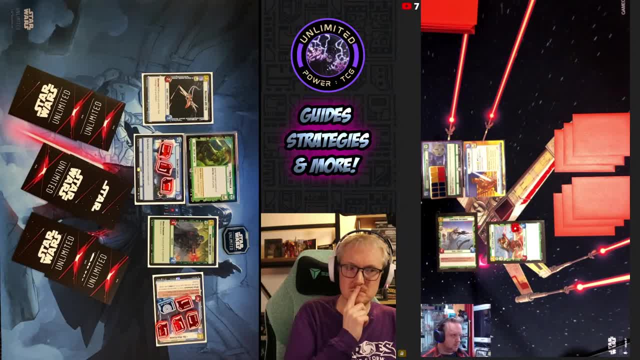 Um, I do keep forgetting it, don't I? Okay, Is that gonna do a thing? Possibly? Uh, I'm gonna have to take out Obi-Wan before then. Uh, what's doing the most damage? That's doing that amount of damage. 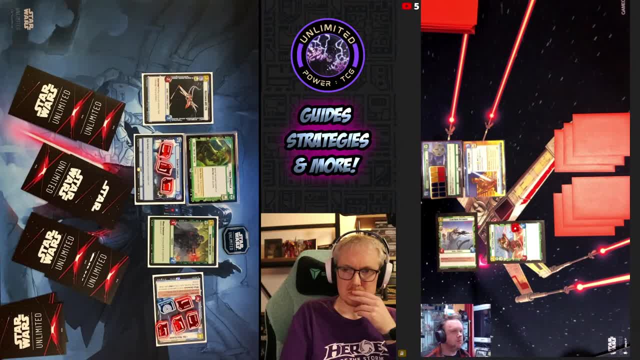 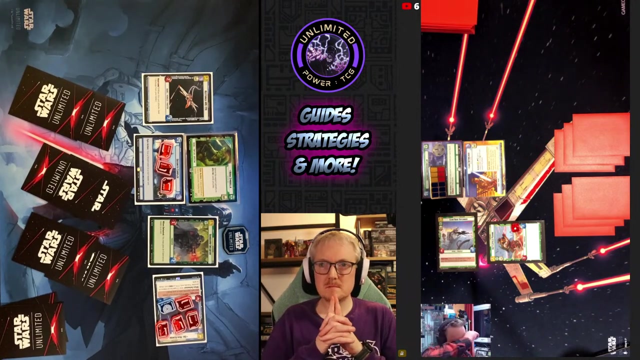 That's doing that amount of damage. So Let's, Let's- Um, I could just change my plan completely, That'd be funny. Let's change my plan completely, That'd be funny. Um, Right, so I'll pay four, Mm-hmm. 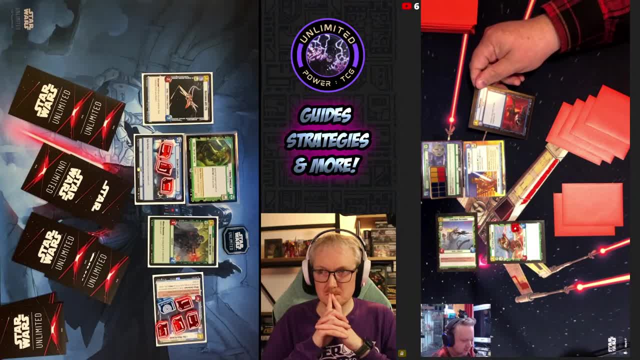 To play Take Down and kill Obi-Wan, Who is a unit with five or less remaining hit points, Which really buggers my shield, doesn't it? That was the plan. Uh, I'll give this two plus one plus one tokens That he gives when he dies. 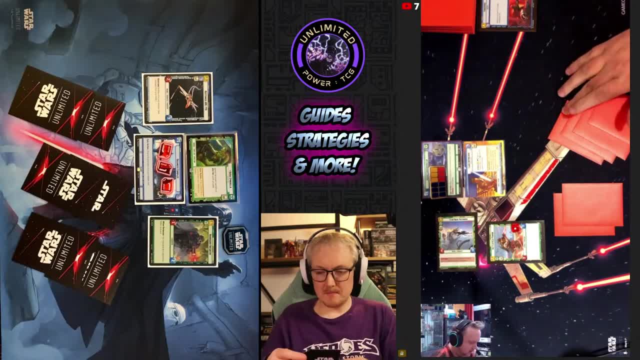 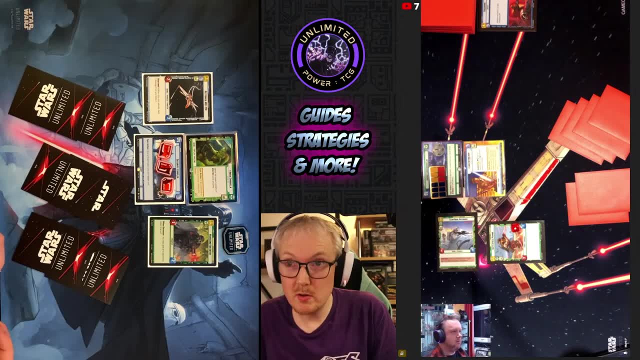 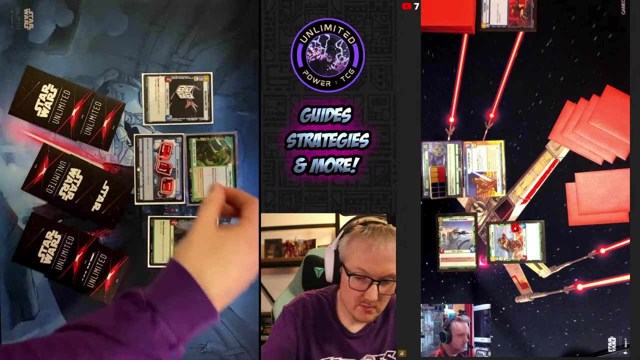 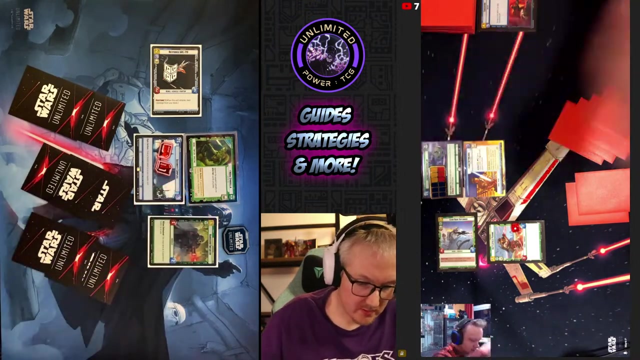 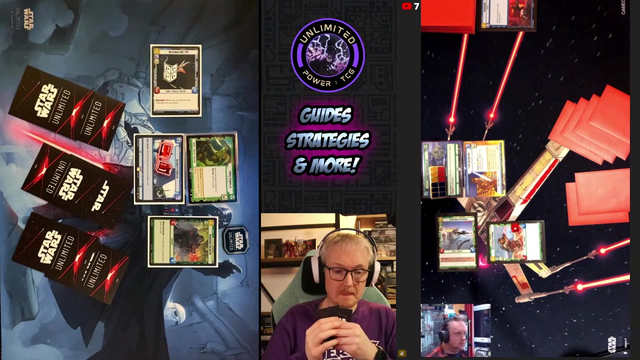 Yep, the restored arc, Okay, And then I'll attack your base And I'll heal my base for one because of that. Fair enough, I will do. Let's do three to base. 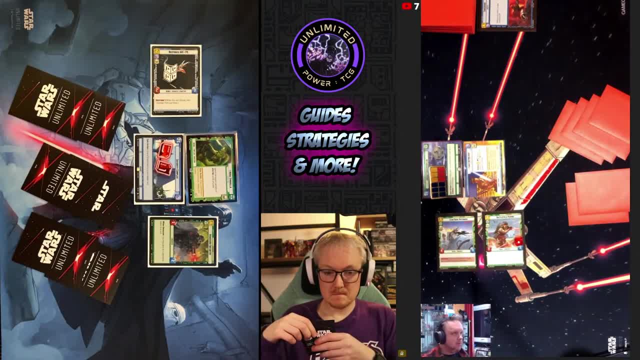 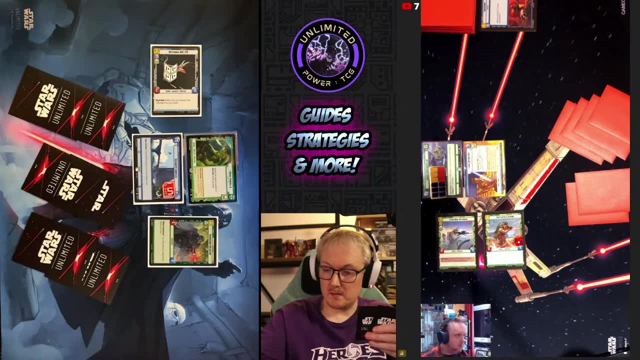 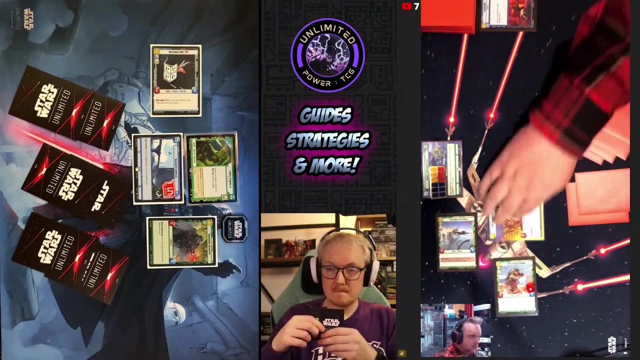 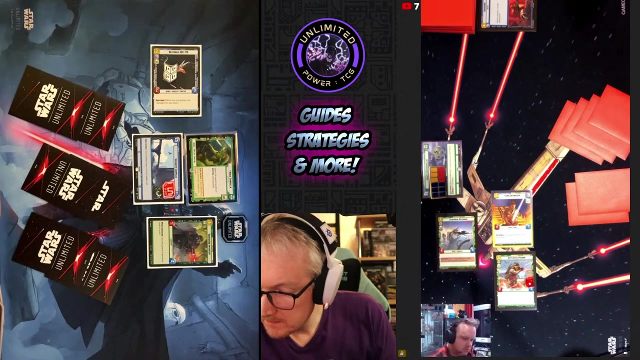 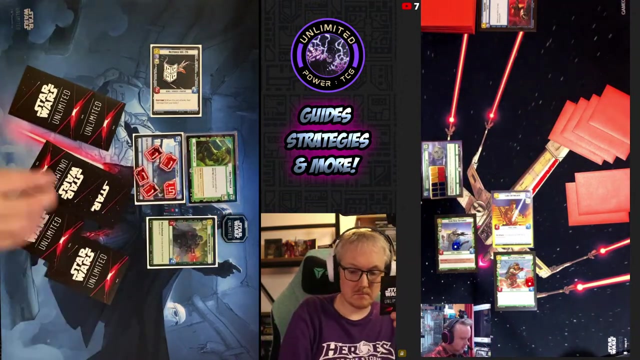 the battlefield marine. I think I'm going to take the initiative. Okay, I'll deploy Luke, I'll do four to base Luke and put a shield on the Echo Base Defender. And I'll do, And I'll do, I will pass. 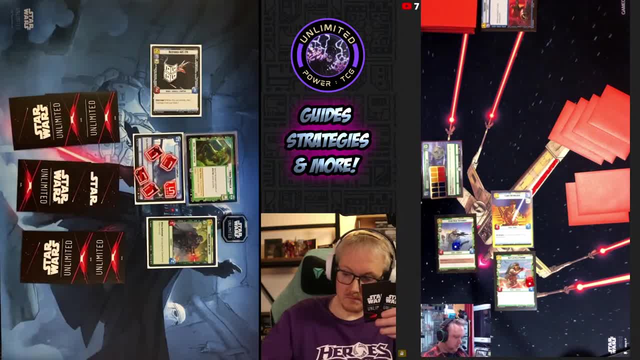 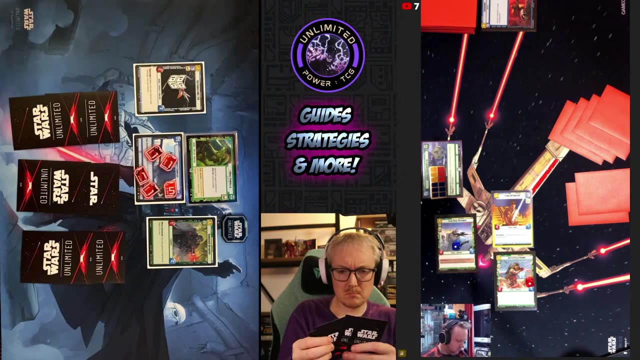 Cool Doop-a-doop-a-doo, Two cards. Yeah, That's going to put me on that much, Which is that and nothing else, or that and that, which is not bad. Okay, I'm going to resource one. 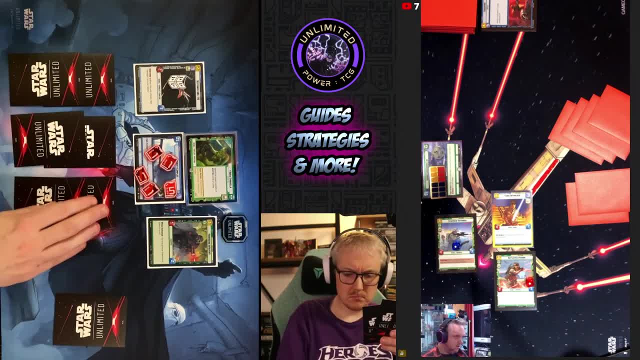 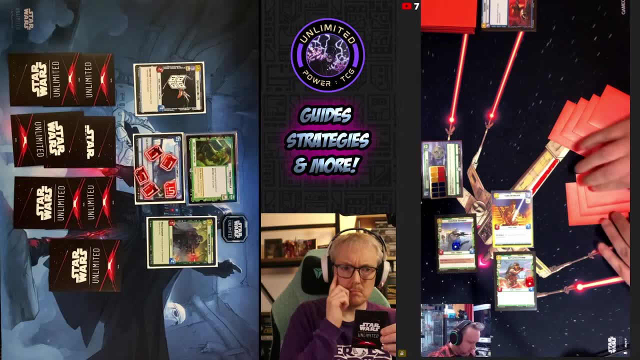 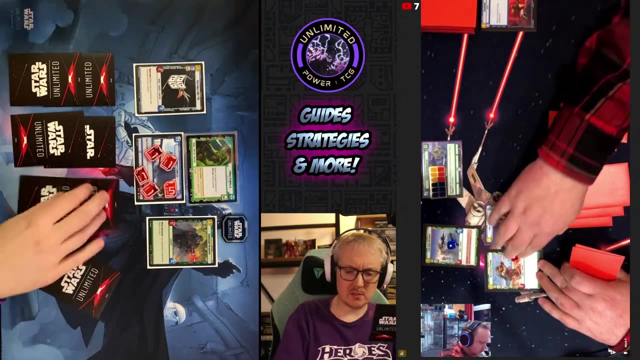 I think I'm going to have to do that in a little bit. Yeah, let's do that. So I'll play one downward to resource Ready up And you have the initiative, sir. All right, I'm going to play all. 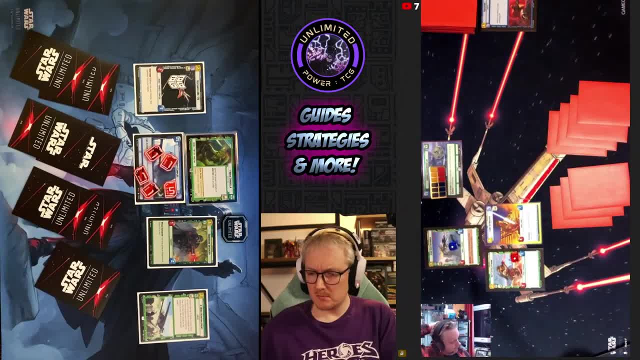 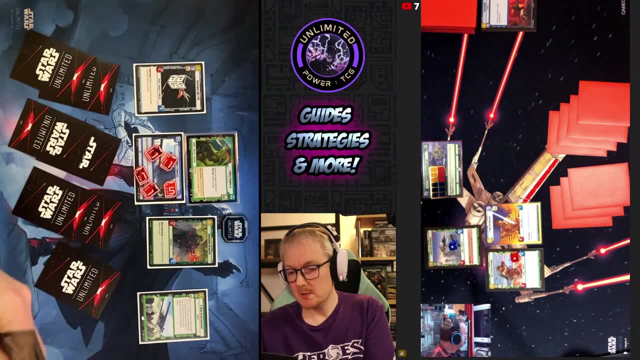 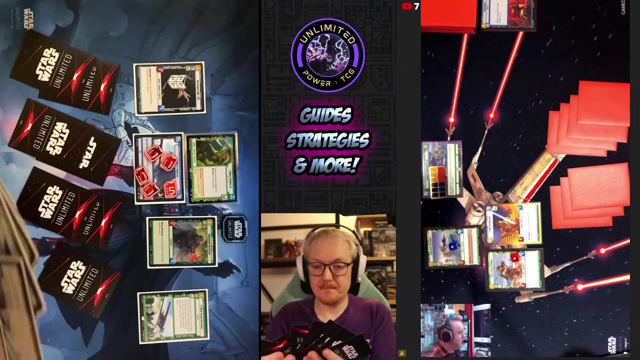 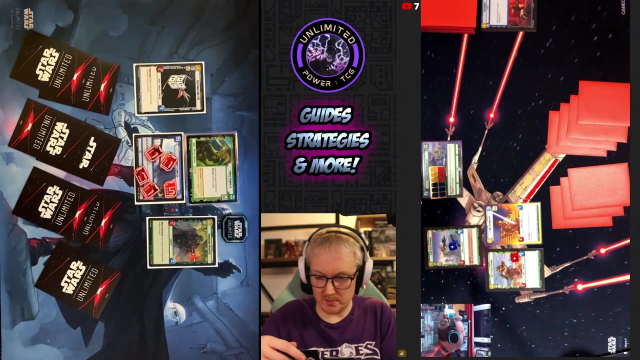 seven Reinforcement. Okay, So one, two, three, four, five, six, seven, eight, Eight, nine, ten Mm-hmm. And I can play up to seven and the rest go just. You can play a maximum of three units with a total combined cost of seven. 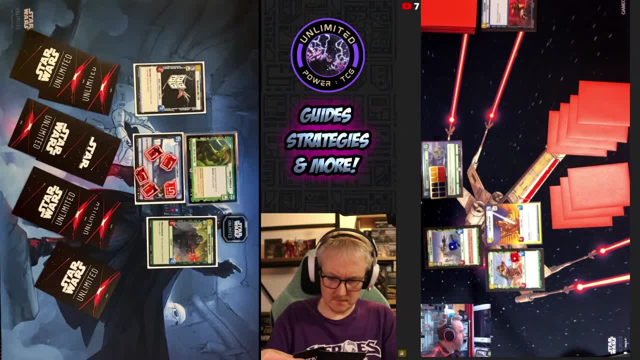 and the rest are to be shuffled and placed at the bottom of your deck. What was in my hand? Yes, okay, Yeah, it's worth putting your hand down, Yeah, so you don't get them confused. Interesting, Okay, I'm going to play an Alliance Dispatcher. 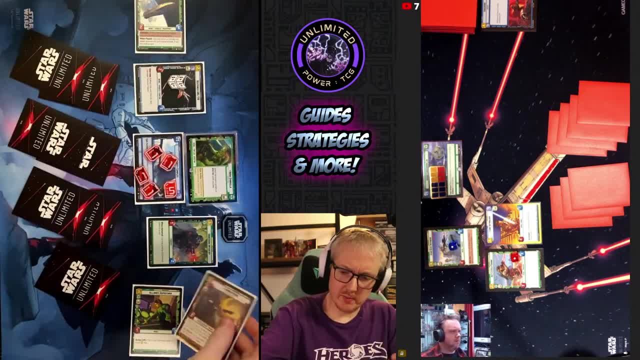 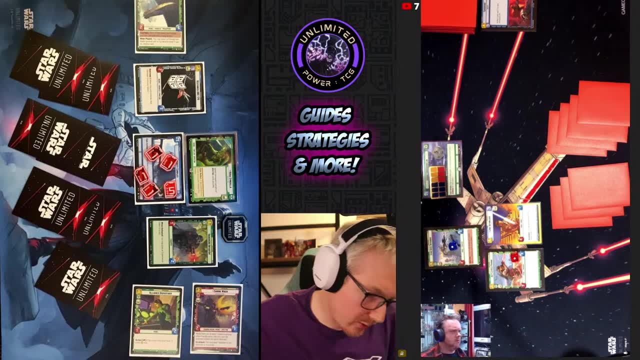 I'm going to play a Bright Hope, Yep, And I'm going to play a Sabine Wren, Okay, And I'll mix these and put them on the bottom. So the Bright Hope, lets me return a friendly. No, I don't want to return anything to my hand, I don't think. 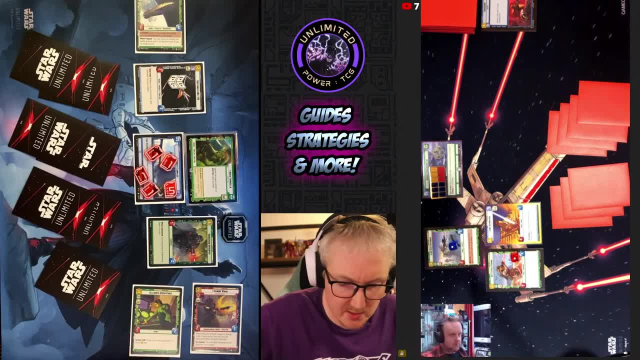 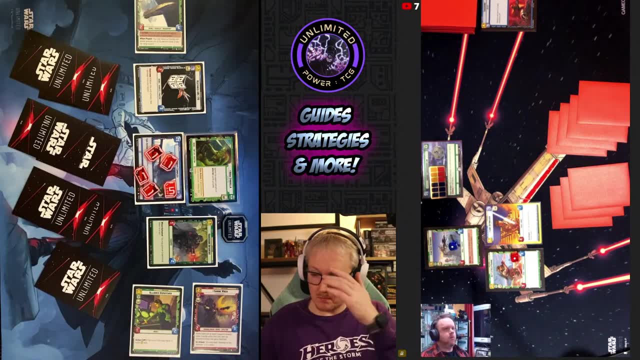 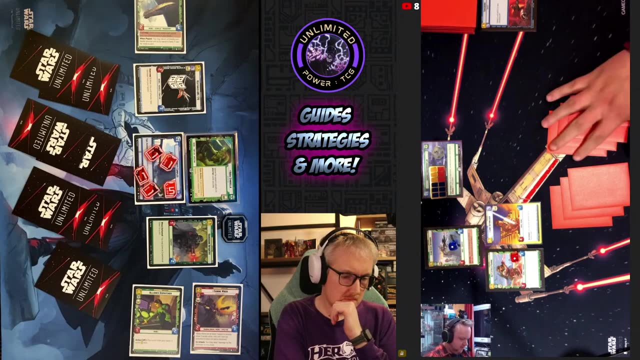 No, it's fine. Yeah, I think that's it. Yep, All right, Okay. So we're doing that much damage there. we're doing that much damage there. Okay, I think I want to pay four to kill your buffed restored arc 170 with another takedown. 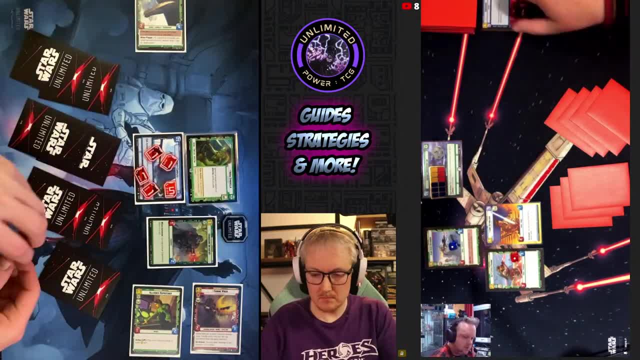 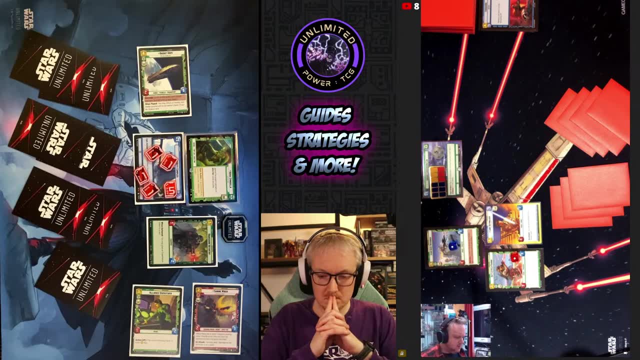 Oh, wow, Okay, You're up. I have a little problem with that Echo-based Defender. Yeah Yeah, Is it too bad sportsmanship of me to say, good, No, I've got nothing doing, man? Um, I guess I'll flip my leader. 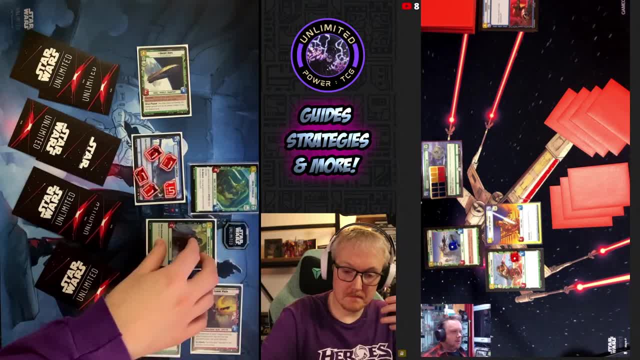 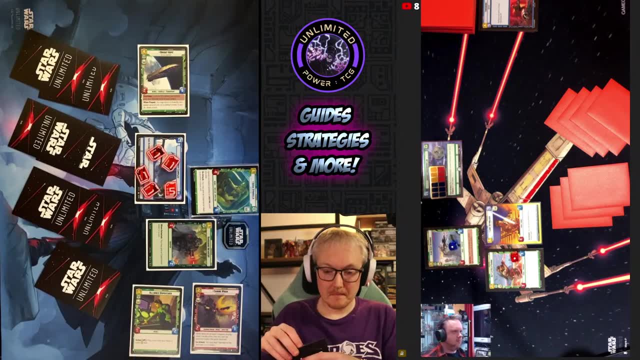 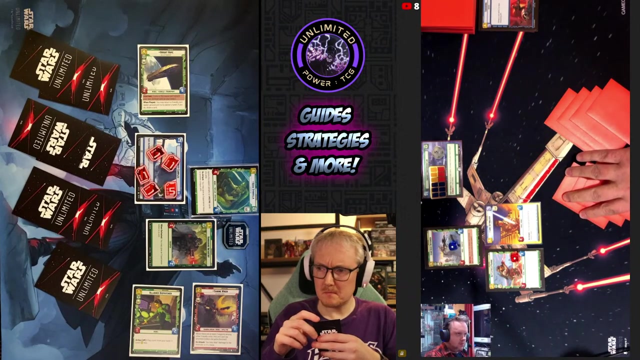 Okay, Here it comes out, Starts doing unpleasant things in terms of experience. So, um, I think that, um, I'm going to play my final three to play down Admiral Ackbar, who's a 1-4. restore one unit. 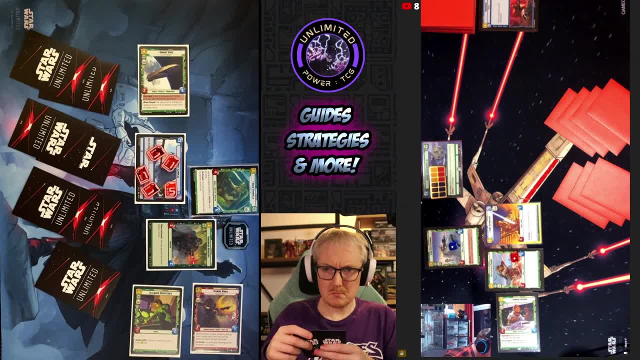 It says: when played, you may deal damage to a unit equal to the number of units you control in its arena. So I'm going to pick somebody in your ground. I'm going to pick somebody in your ground arena and shoot them for four, because I control four units in the ground arena. 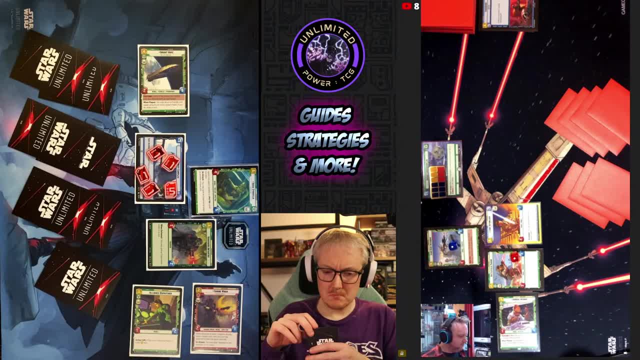 Very nice, And I'm going to shoot Hera for four damage. Cool, Um. That's not really what I wanted to happen there, Because I have seen What's she going to do. Oh no, she, No, she doesn't come in shielded. 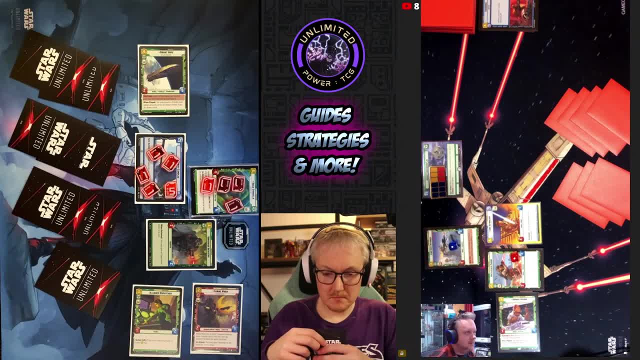 It was the ghost that came in shielded, wasn't it? Yeah, Mm-hmm, Yeah, I don't want her to get a chance to start pumping experience. It's all over everything. So I'm going to kill her. 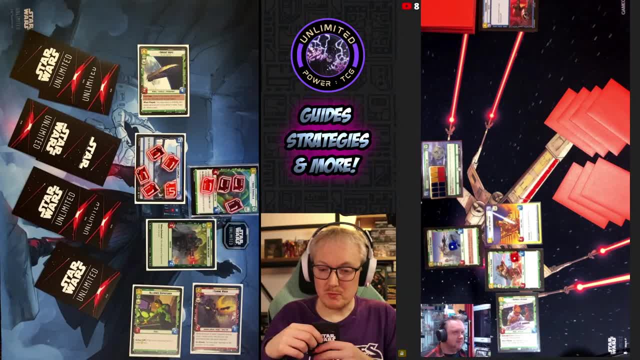 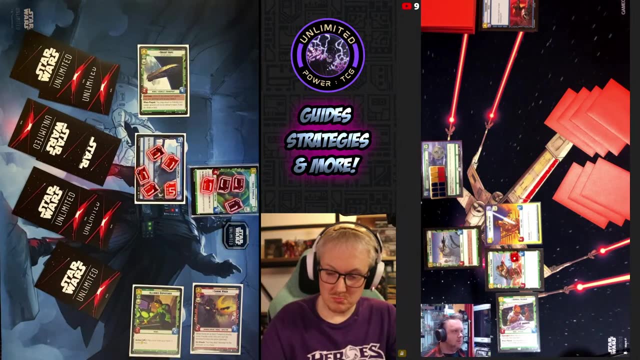 Yeah, that's a good idea. I'm going to remove your shield from your echo-based defender with my vanguard and give the experience token to Ugh, Ugh, Uh, The Bright Hope, The Bright Hope. Okay, fair enough. 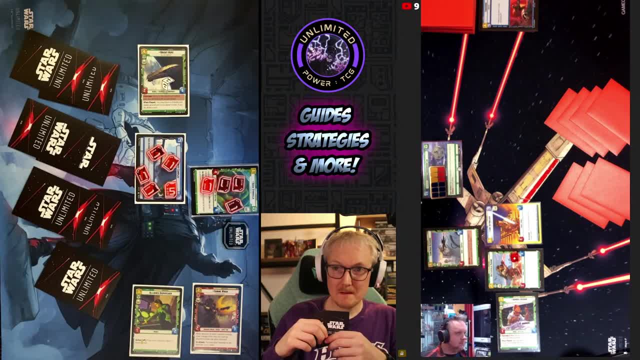 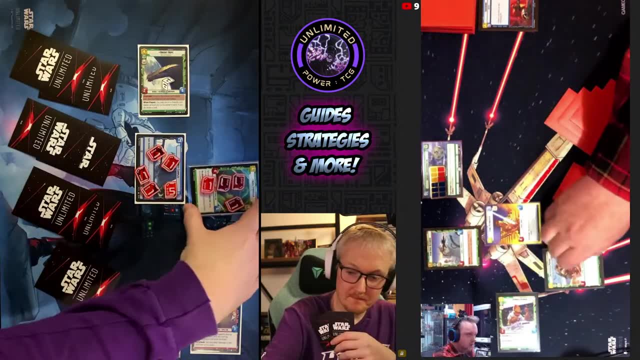 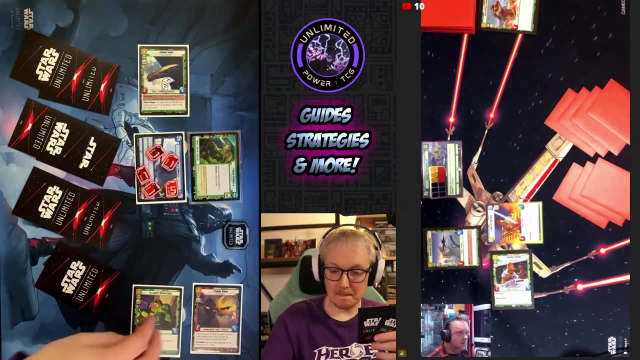 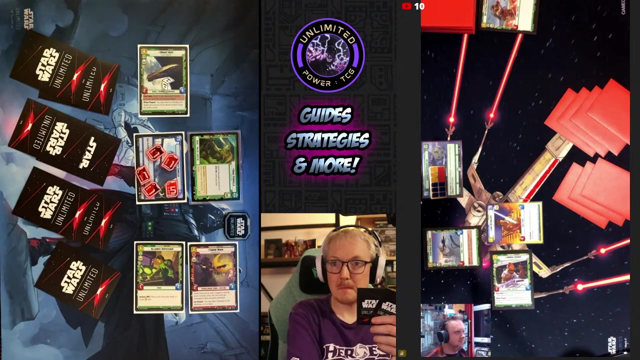 Awesome. Um, I am going to kill Hera with the Battlefield. Marine Cool In a straight trade. Well, I'll take an issue, No worries, Once defeated. she's exhausted, but it doesn't matter because you're just taking the issue anyway, so it's fine. 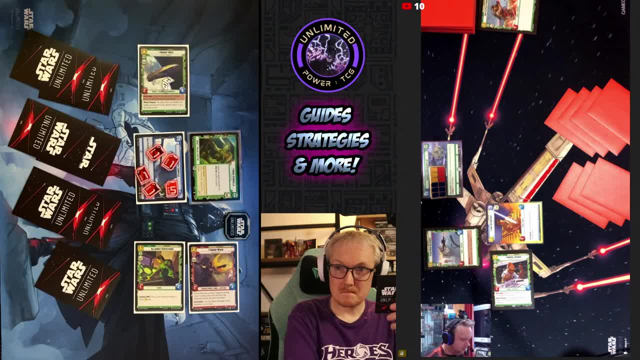 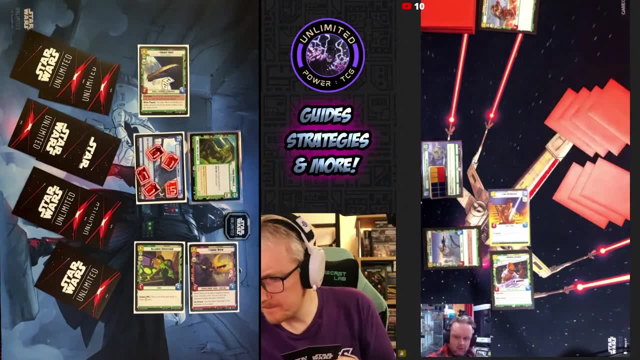 It's not like she does anything either. I'm going to kill Hera once she's gone, so that's all good. Um, Cool, So you've taken the initiative. I will attack fort-based with Luke. Yep, I will give a shield token to the echo-based defender while I'm doing it. 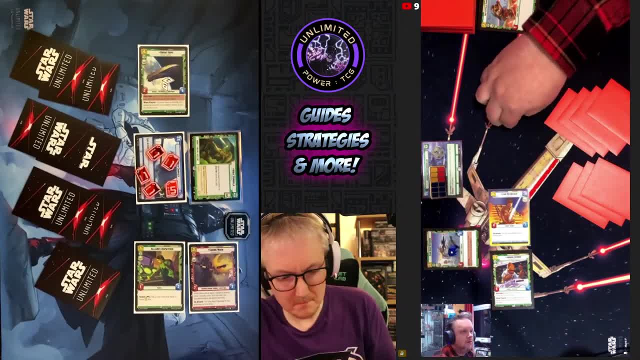 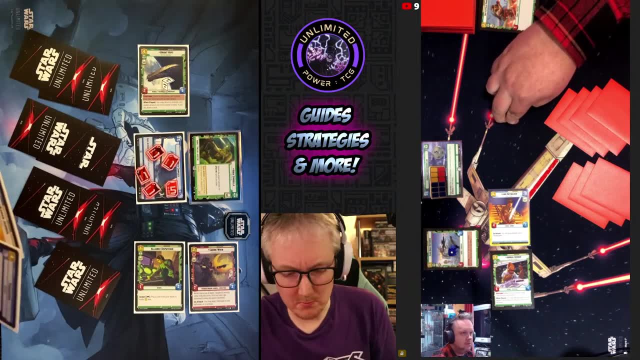 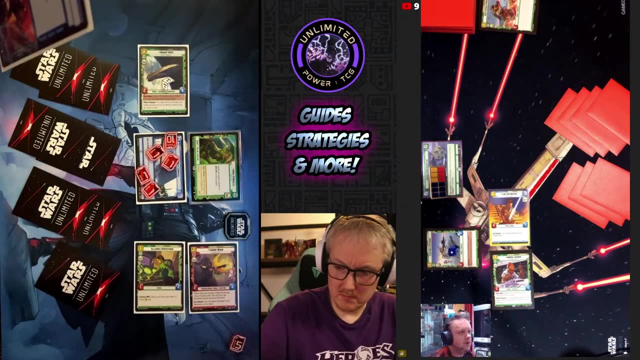 Who will then attack? um, Did you just hear a ping? I didn't. no, Okay, don't worry about that one. Um, The echo-based defender will. Resources aren't Massively useful right now, but you're still. 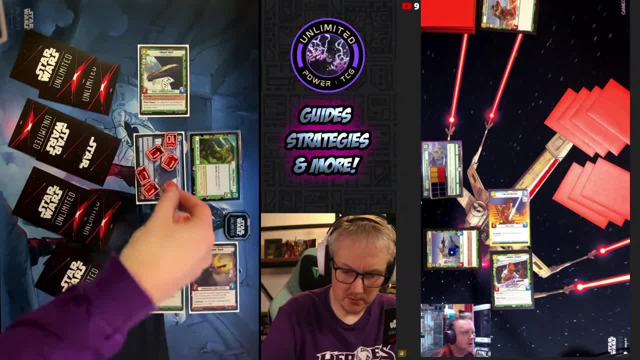 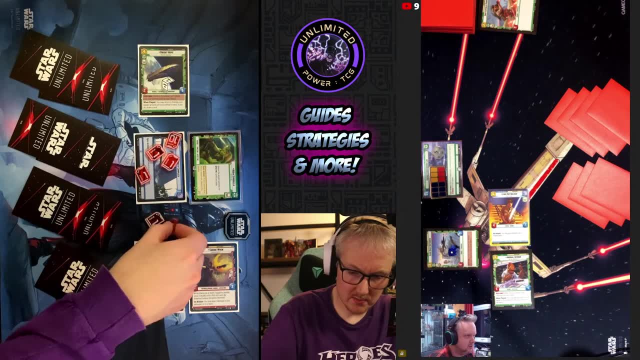 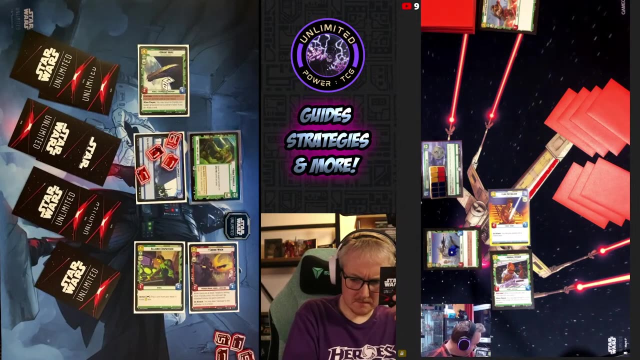 The damage that you're doing. How much health have you taken? I had nine, so if I put down a ten, Another four is thirteen. yeah, That's as high apparently, Apparently so, Um, So if I do another four, that puts you on seventeen, which is 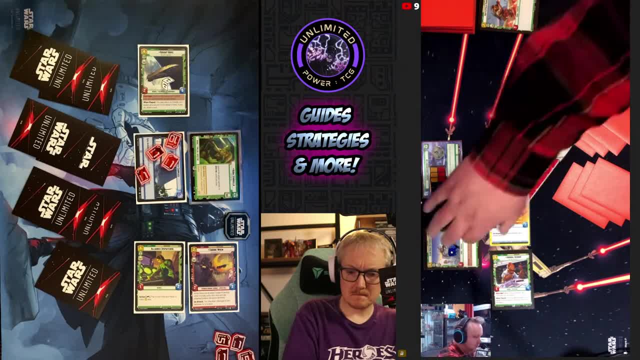 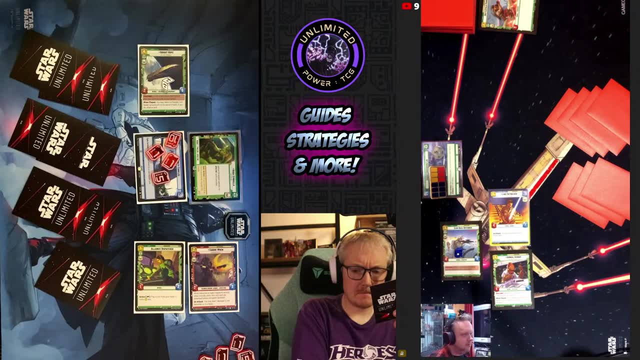 Eight away from death. So yeah, Let's just do fort-based with the echo-based defender. Okay, And I will pass. Yep, Okay, Two cards. Yep One, two, three, four, five, six, seven. 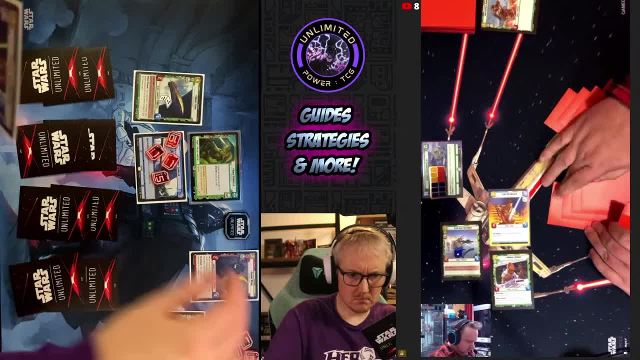 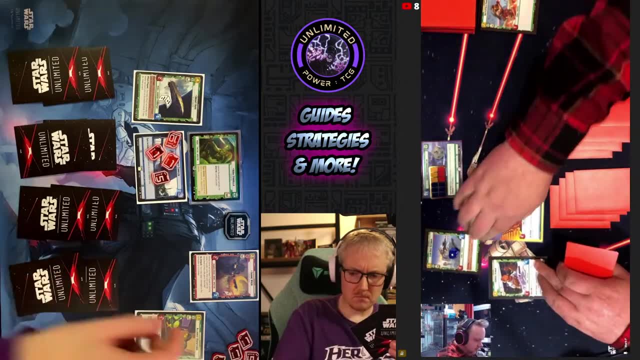 Hmm, Yeah, I think we're going to do that. So let's do that And that's ready up And you have the initiative. sir, I'm going to tap the dispatcher. I'm going to tap. Do you know what? 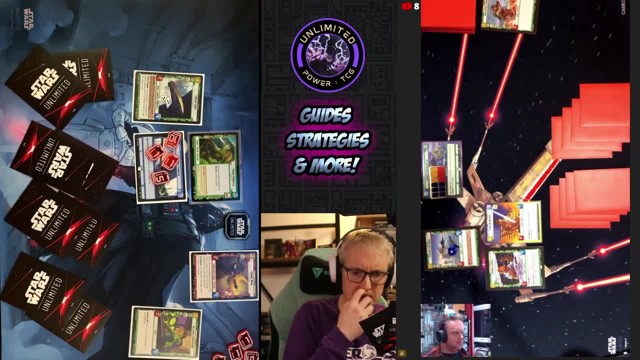 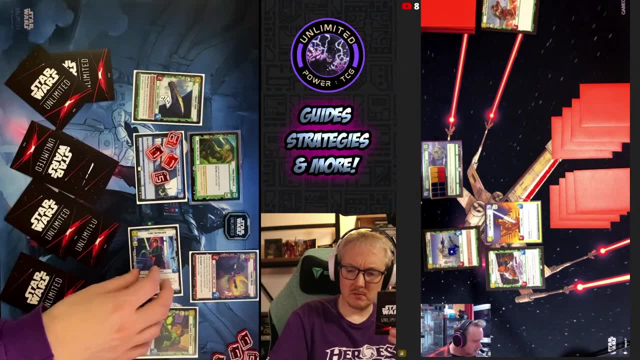 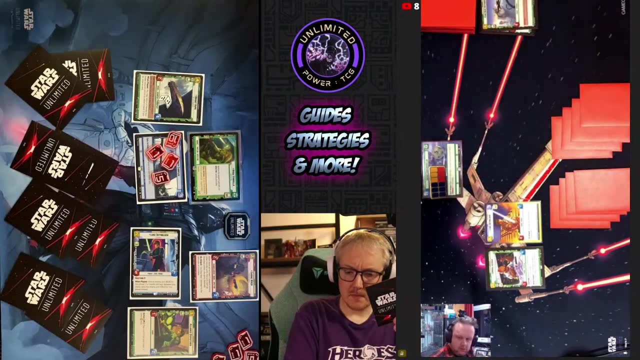 There's no point in tapping the dispatcher. I'm just going to tap seven Yep And I'll play Luke Yep And I'll give your base defender minus three, minus three, Which kills it. Very good, Very good, Okay. 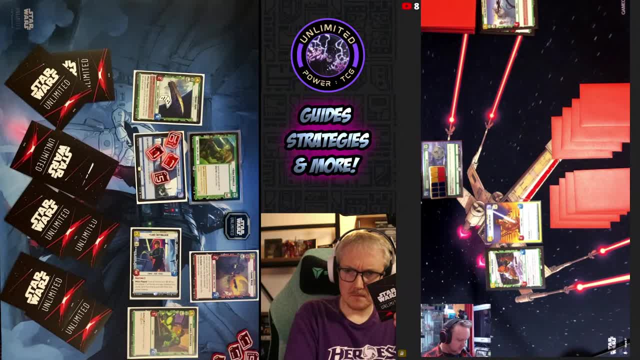 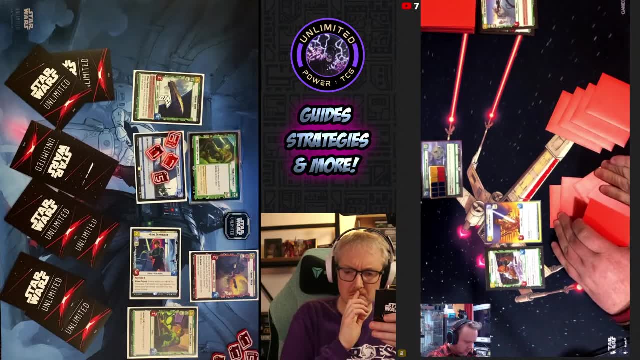 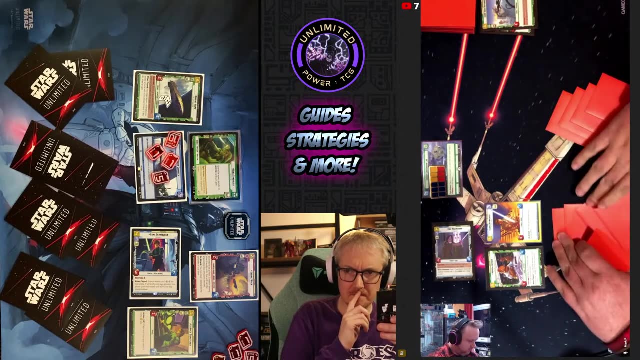 Hmm, Well, I think, in response to that, I'm going to pay six and play Obi-Wan- Very nice, Which will leave me with two remaining unspent. Yeah, I'm going to play Obi-Wan. Do you want to attack your base? for three with the Bright Hope. 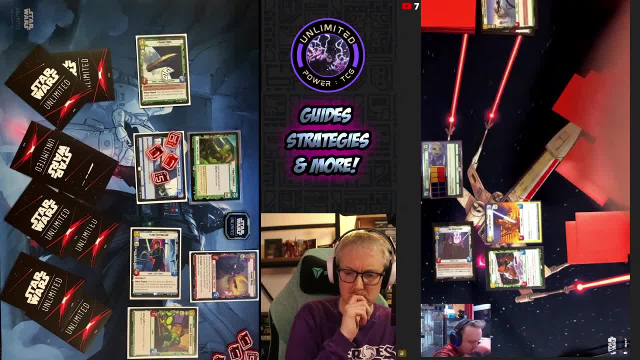 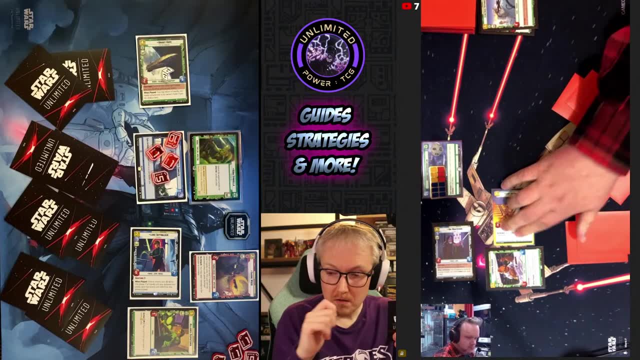 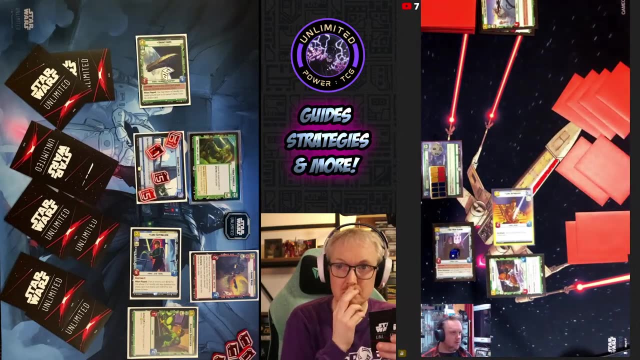 Sure, Fine, I'm happy to take that. Luke will attack your base for four and put a shield on Obi-Wan. Yeah, I've got a real problem here. I'll take Obi-Wan's shield off with the. 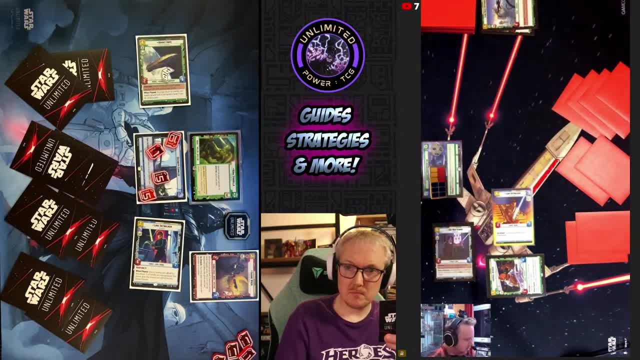 I'll add a dispatcher. Yeah, Dispatcher, Dispatcher. Fine, I need to do. You've spent all your resources. I need to do four damage to you. Either Luke or Ackbar can do that, So I'm going to take the initiative. 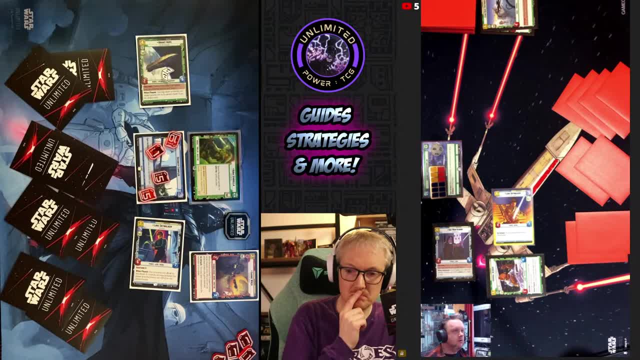 because I reckon I can kill you with the first action next turn? Yeah, probably. Yeah, I was going to attack Obi-Wan, Which will do two to Obi-Wan and one to base, I think. Or does it allow you to do it to Defender as well? 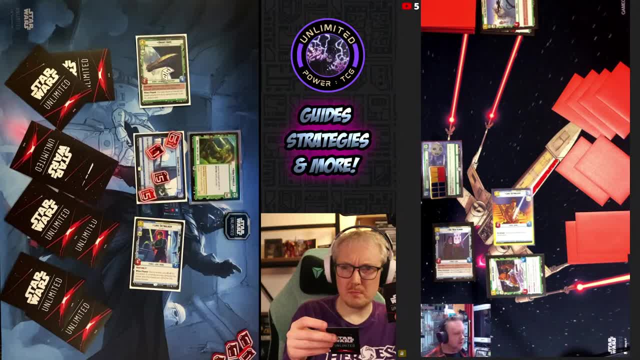 It lets you do it to the Defender as well. Okay, Yeah, I mean you can, But I guess yeah sure, Sabino hit Obi-Wan. Okay, So Obi-Wan takes three, or are you going to split it? 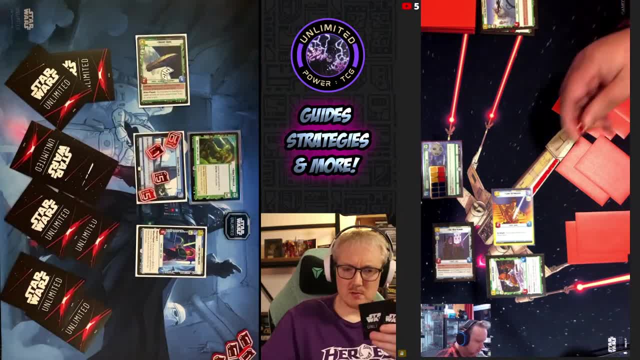 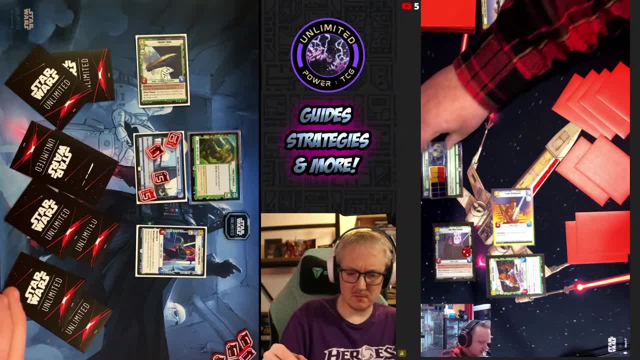 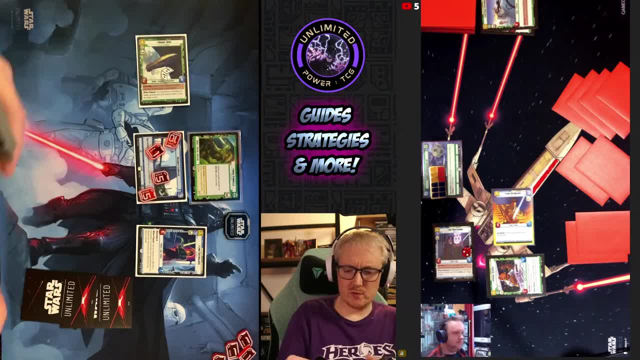 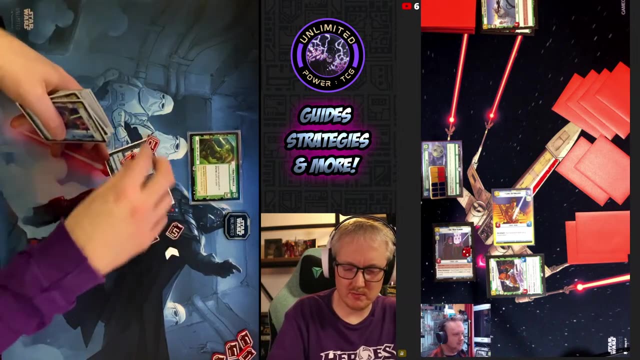 I made a big mistake there. I could have used a takedown when you had that Echo Defender shielded like two turns earlier, but I think I was so keen to play the U-Wing reinforcement. Oh yeah, Yeah, I just like I. just what do you call it when you get like the headlights on? 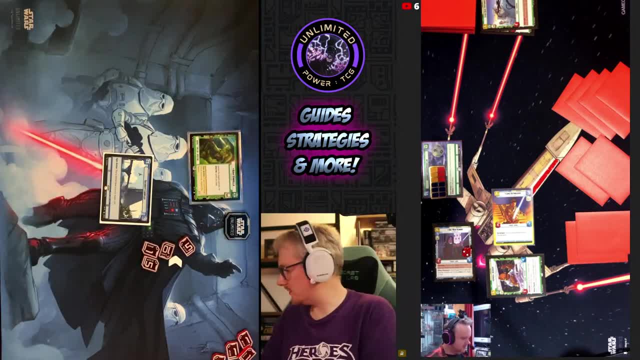 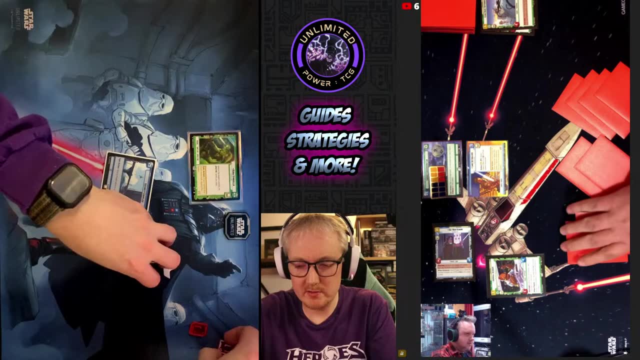 Yeah, I just didn't see that other player at all. Yeah, It was complete tunnel vision. No, I get you. So I thought that that was going to be big, but what would have been much bigger was just get rid of because you kept shielding it. 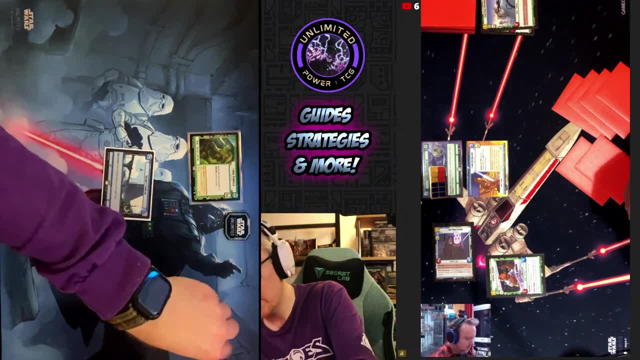 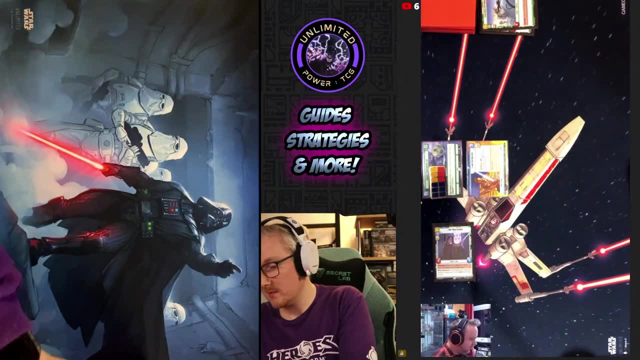 So get rid of it. That would have been a much better player earlier. but good, one game is just a good way to end the night. Yeah, It's almost midnight, We should probably stop. Yeah, exactly, I was going to say I'll keep this deck together and we'll get together for a tiebreaker at. 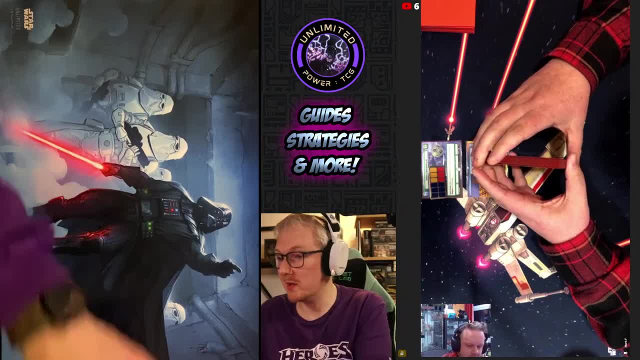 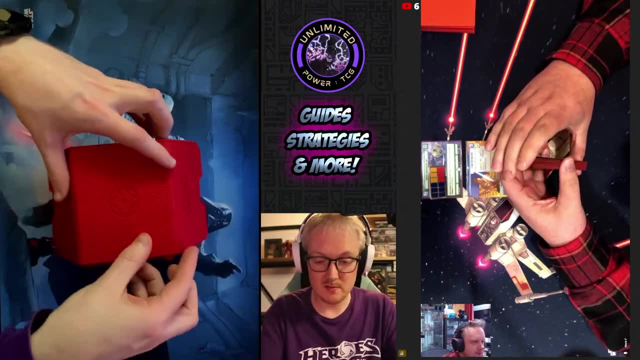 some point in the future. point I was going to say tiebreaker, Tiebreaker next Friday night. Thanks to everybody that hung out and watched the game. Please leave a like on the stream if you enjoyed it. Yeah, It's good to see you as plays. or what you did wrong or you should have done better.